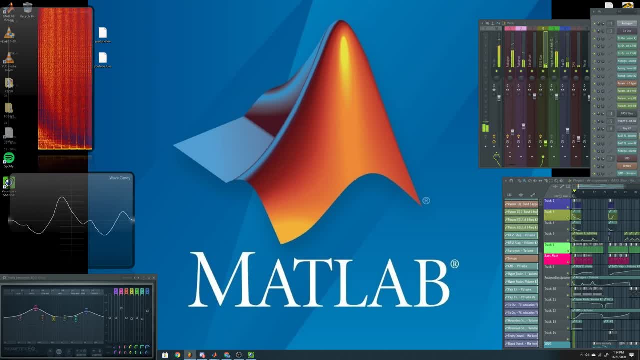 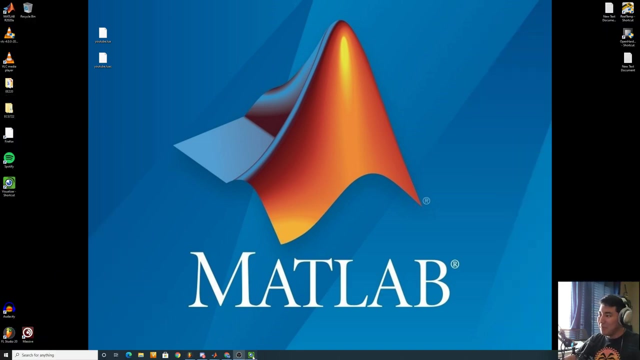 All right, everyone. how's everyone doing? All right, there we go. Oh yeah, that's a quick demonstration of some cool music stuff Sampling. oh, here's a filter. All right, how's everyone doing? Today, we will be discussing. 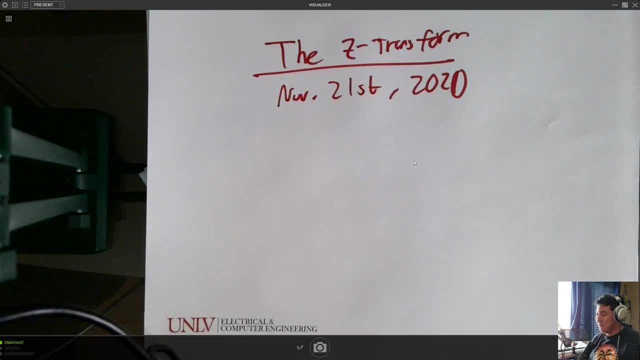 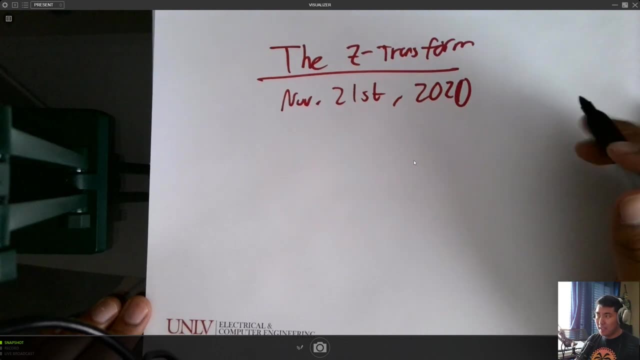 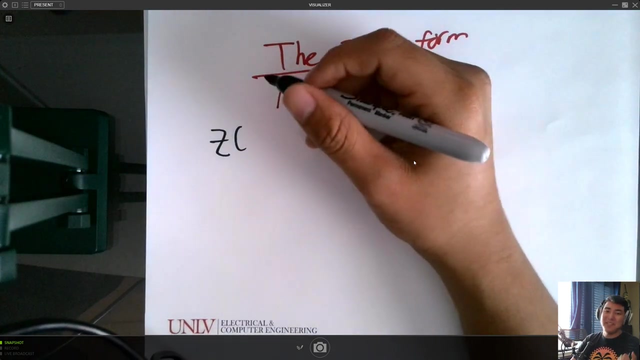 discussing about the Z-Transform and hopefully helping you understand what's going on. So I'll try to make this video pretty short- well, not too short, but just to get a basic understanding what's going on. So Z-Transform, it's an amazing tool. It's basically, you know how, the Laplace 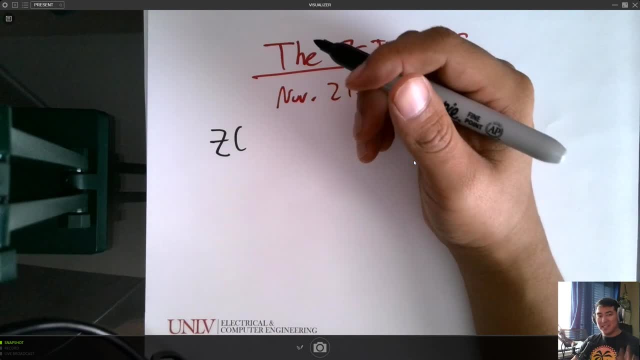 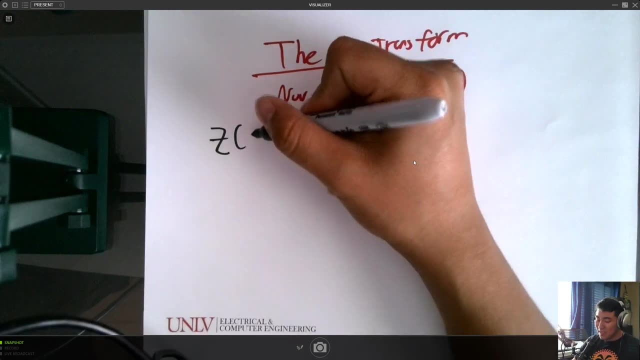 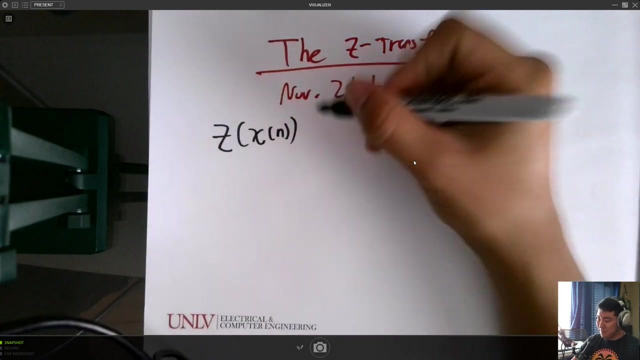 transform is used for analyzing analog systems. Well, the Z-Transform is for discrete systems, but this is a special little rule, so I'll just establish that right now. We're just going to go over how to practically do this. So the Z-Transform of a signal, the rule is we're going to analyze a. 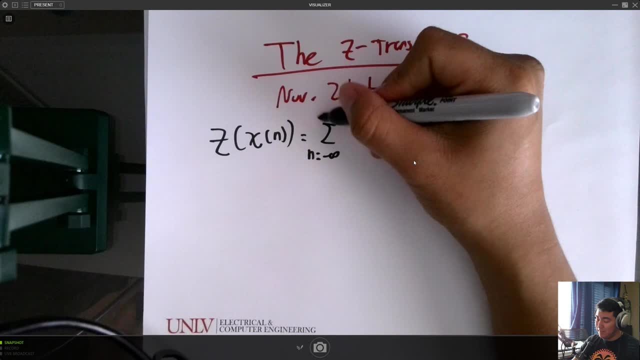 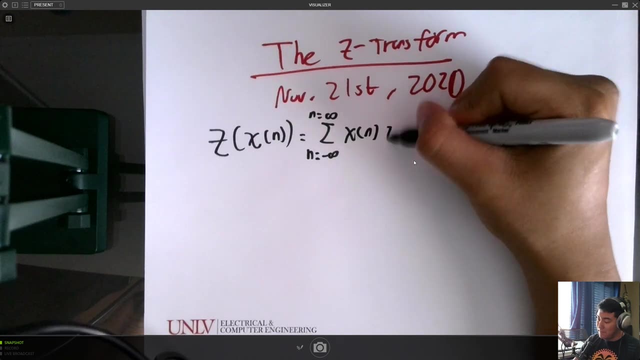 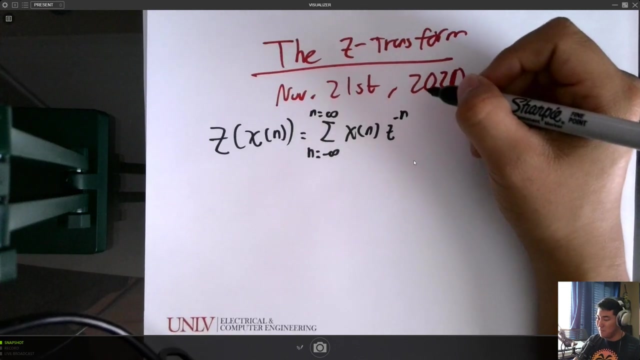 signal from the first point, which is well, minus infinity, to the final point, on that signal to infinity, the entire signal of z to the minus n, And yeah, we just multiply that z to the minus n term. So that's how we turn it into the Z-Transform. So now the one thing I want to. 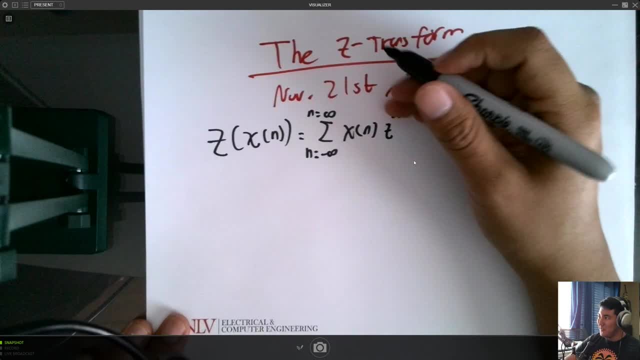 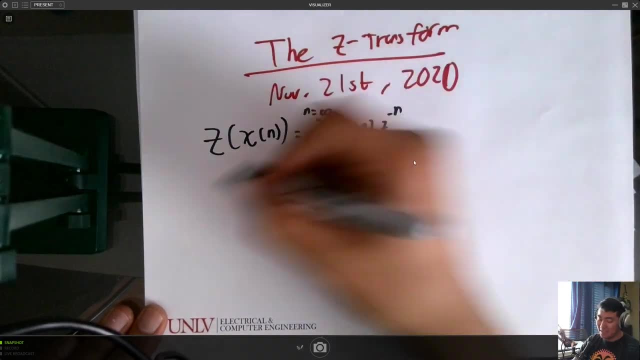 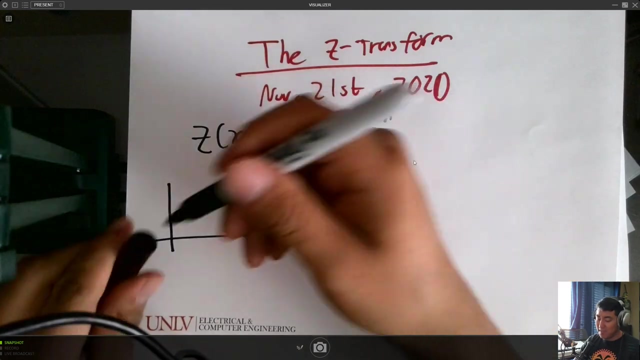 discuss is basically: well, what do we do And what's a Z-Transform? How do we start with this Z-Transform? So let's say I wanted to choose, well, some finite signal. We're just going to use an example. Let's do this And let's assume that a 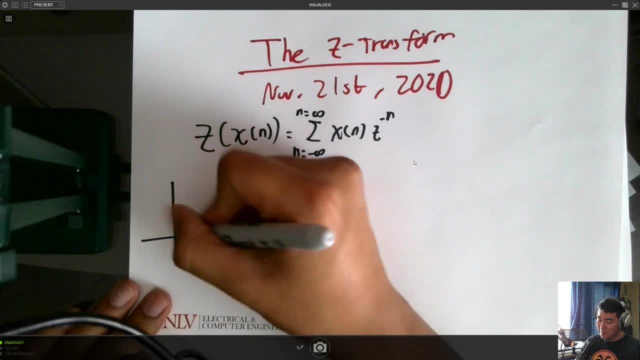 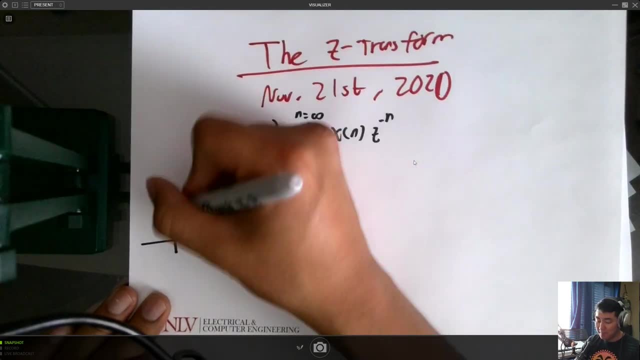 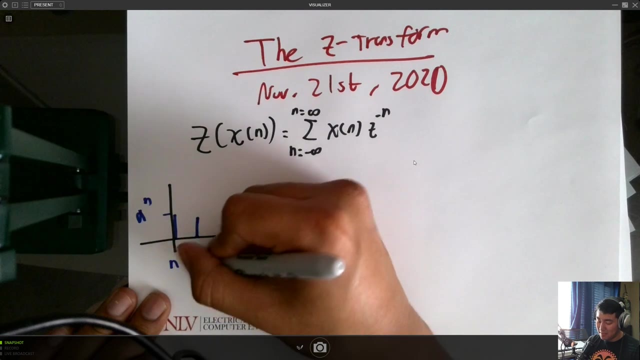 signal exists just for a few seconds. Let's just do this: two, three, just some random signal whatever, Or the amplitude, let's just call it a of n, So it just changes as a function of. well, n is equal to zero. one, two, three, And then let's just 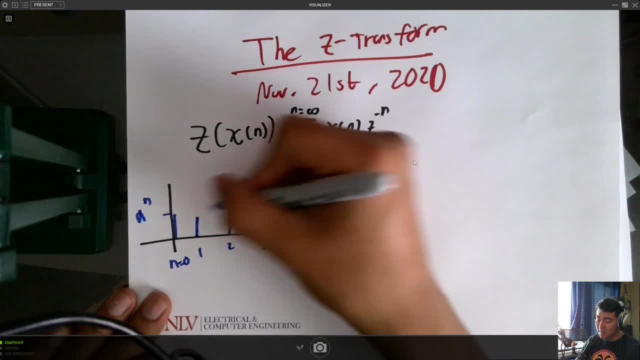 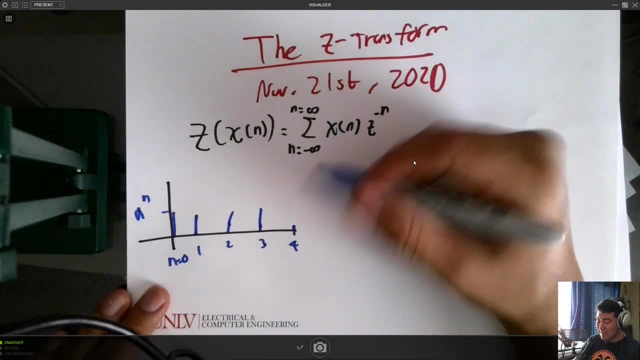 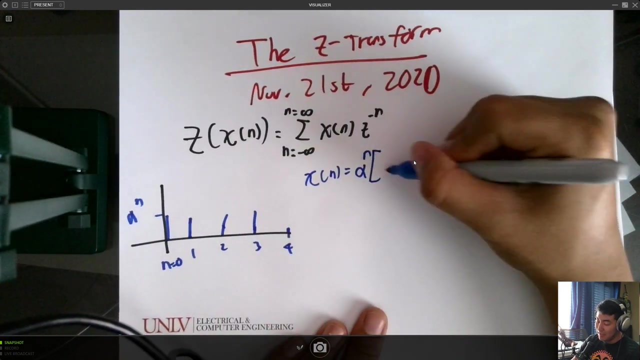 say, a four just turns off, It doesn't exist. So let's just do that for an example. So what we're going to do is, well, we have this signal that we can. let's just define it as it has an amplitude: amplitude of a- n. It exists at u of n, So it starts at n is equal to zero. 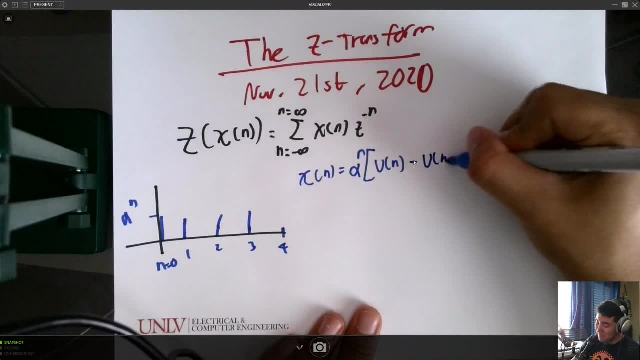 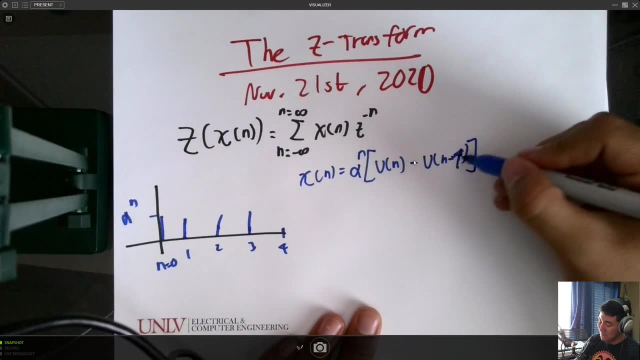 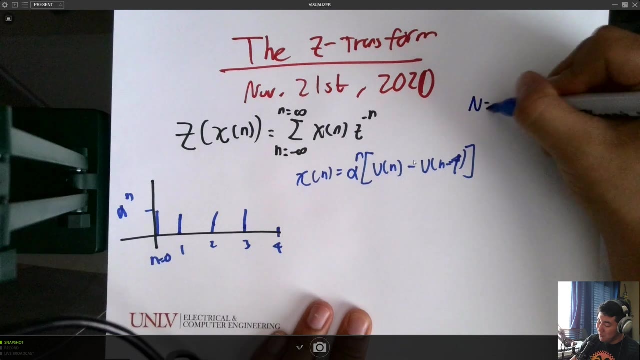 But then it ends at u of n minus four. There we go. So u of n is equal to four, n is equal to four. This turns into one. This is always one. That's zero, So that's a finite signal. So if we wanted to say how many elements are in here, we have 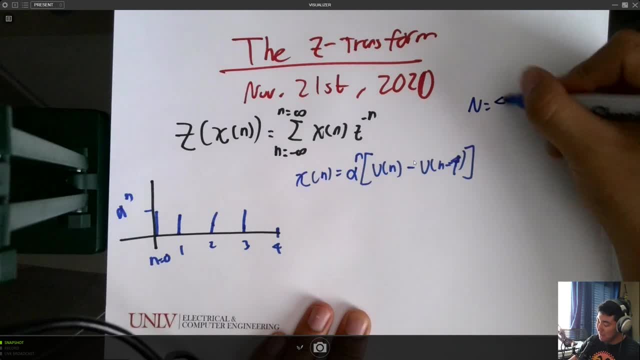 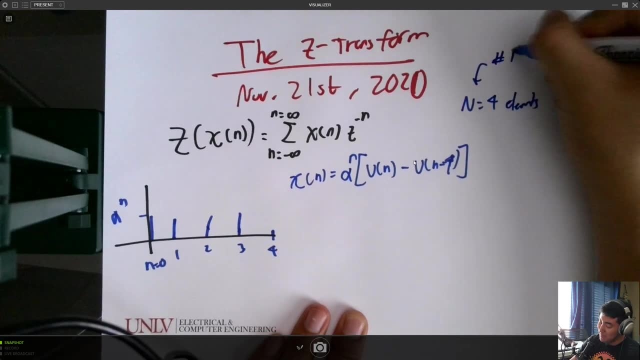 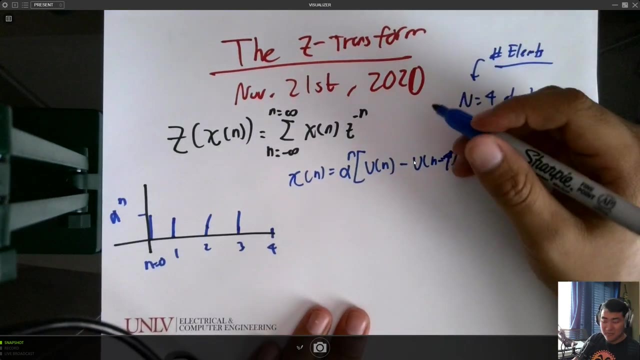 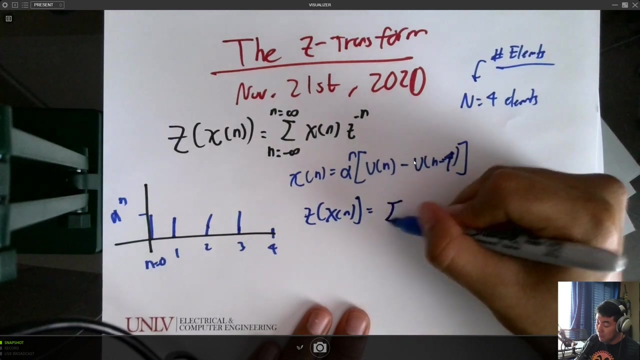 one, two, three, four. So we have four elements. So n is just basically treated as our number of elements. So that's a quick little rule we have to establish. So now we have our finite signal. Now let's take a z-transform of it, So then it's equal to. we're going to look at the entire. 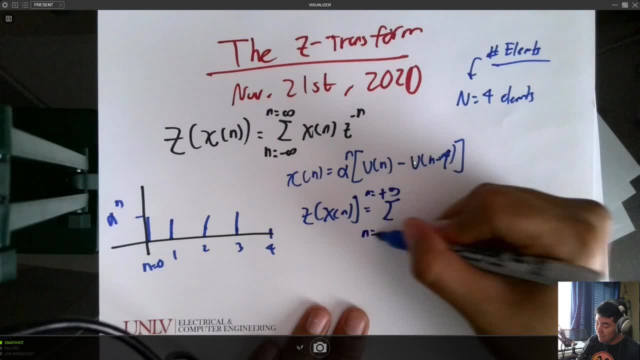 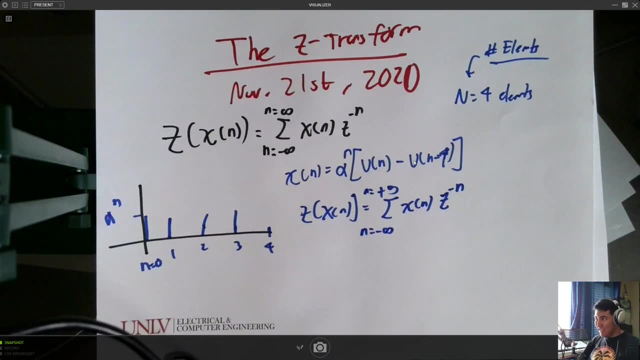 signal. n is equal to positive infinity, n is equal to minus infinity of x, of n, z to the minus n. There we go. And now you're saying, oh gosh, it's a sigma or a summation, And don't worry. 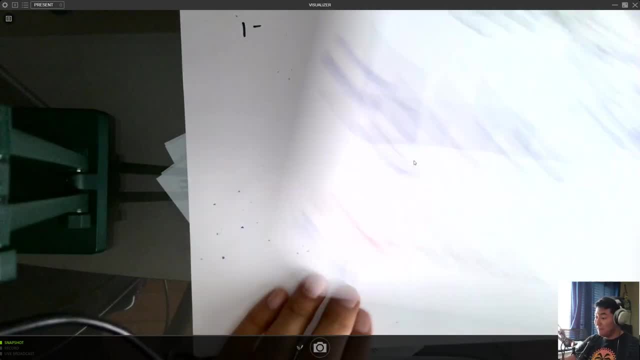 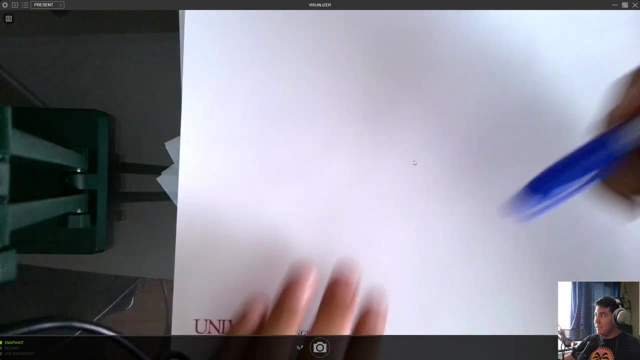 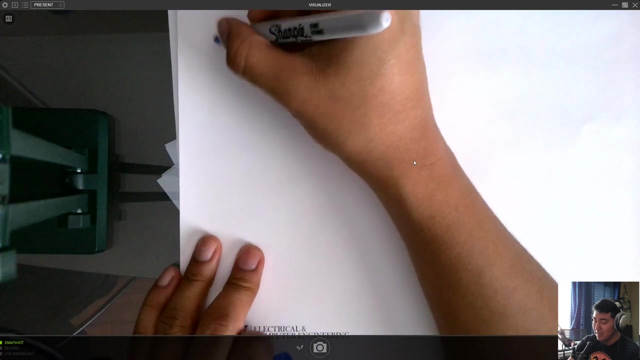 we'll walk through the step, just in case you don't know what's going on. So let's do that The following: grab a piece of paper, go There we go. So let's just rewrite this as positive: infinity n is equal to minus infinity. 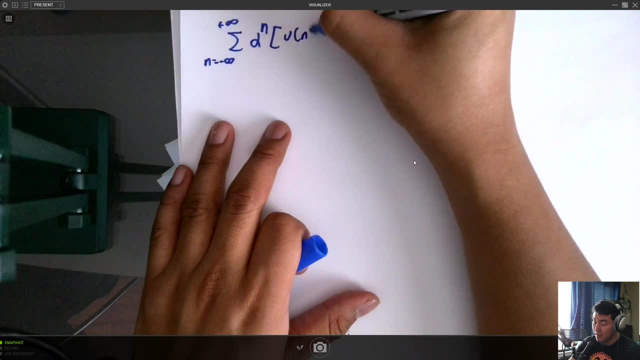 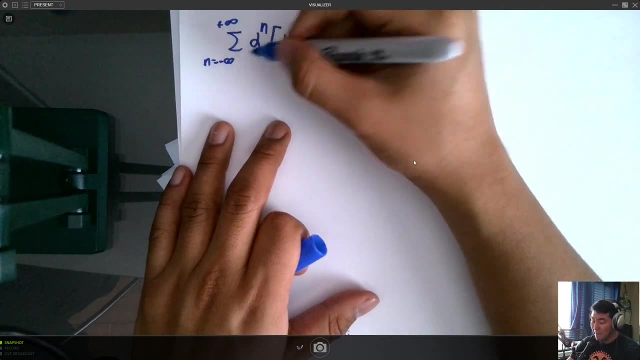 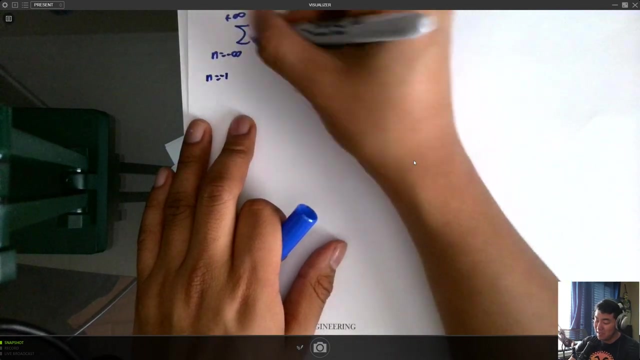 of alpha of n? u of n minus u of n, minus four of z to the minus n. So how do we approach this So that we know that if n is equal to minus one, that means u of n is going to equal to zero? 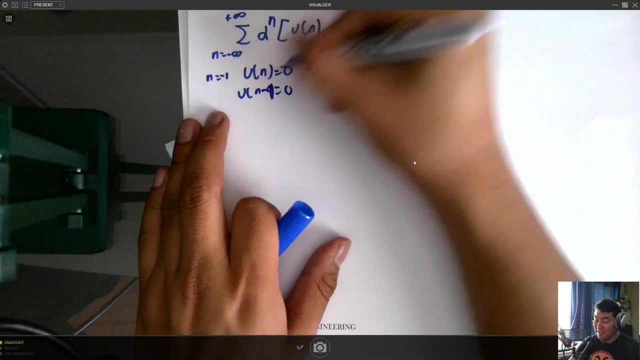 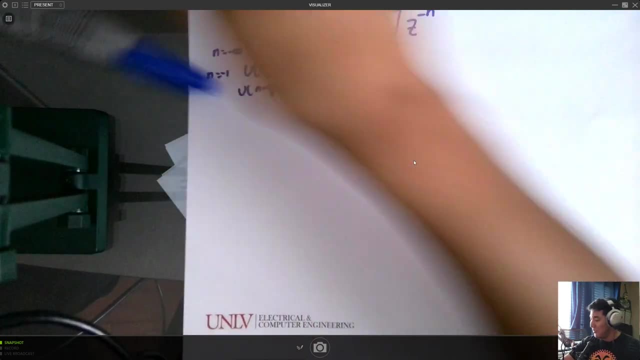 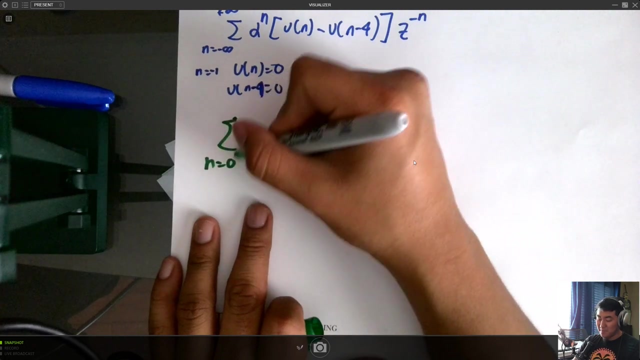 and then u of n minus four is also going to equal to zero. So that means well, nothing exists when n is equal to minus one any other negative numbers. So that means we can change. we can do a following change: n is equal to zero because that's the only point it exists at. 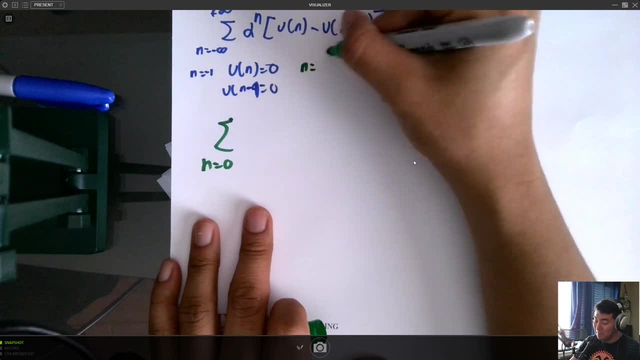 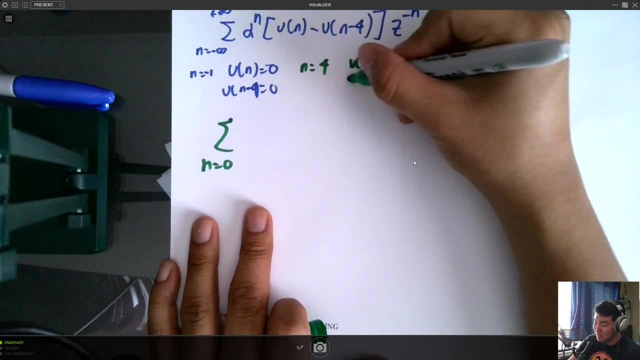 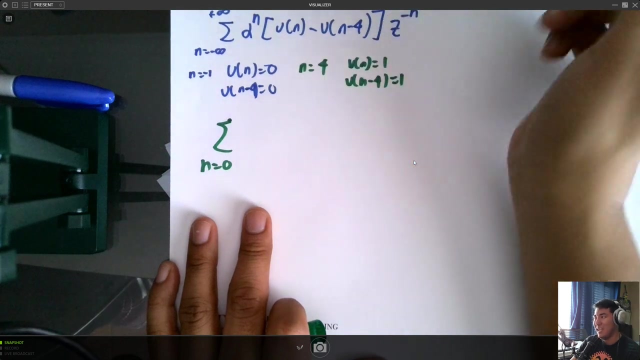 And then if we look at the top terms, if n is equal to four, then that means, well, this becomes a one. u of n minus four is also equal to one. That cancels out that whole thing. So nothing exists at this point and all the further points that go up. 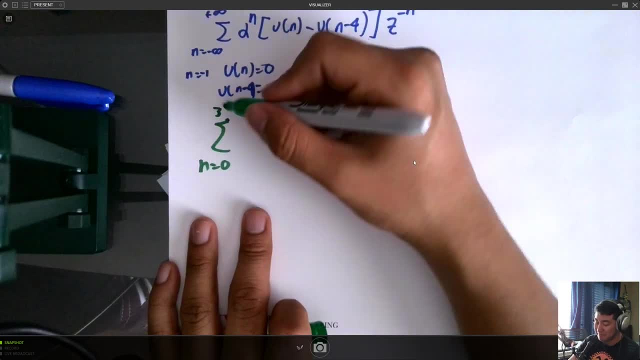 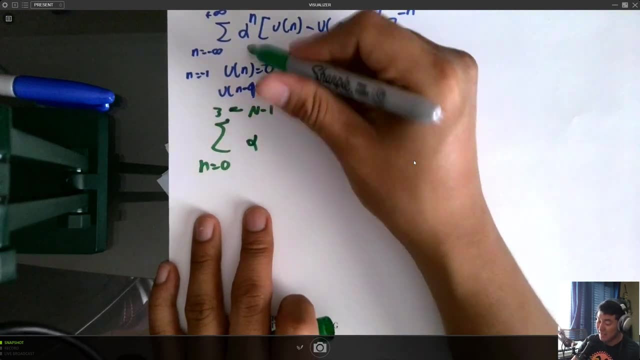 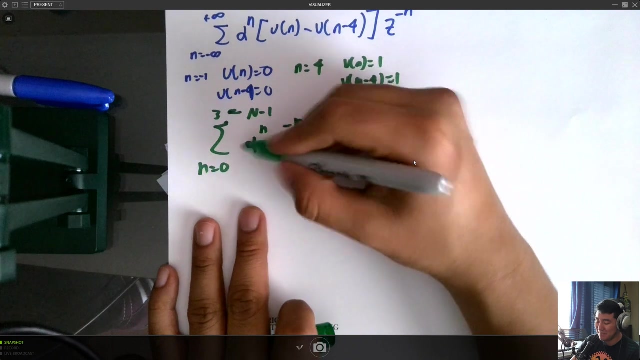 So if we do this, let's do three. Well, we can call this one n minus one for a surprise at the end. So alpha of n z to the minus n. So now you're like, oh gosh, this is a summation right here. What do we do? 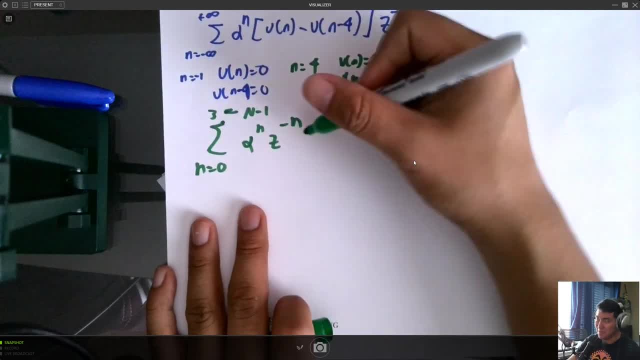 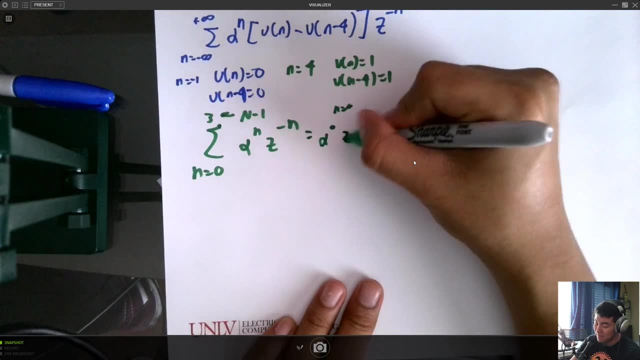 So the first thing you could do is, if you wanted to, you can just brute force solve for this system. So let's just look at: n is equal to zero. That means alpha of zero z to the zero plus n is equal to one alpha z to the minus one. 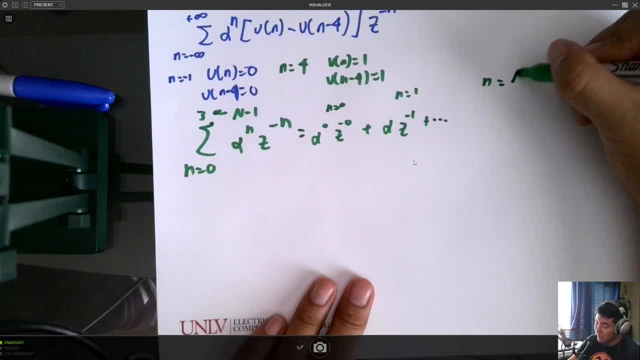 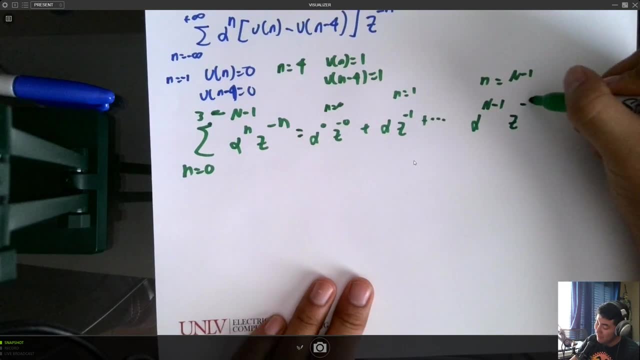 Then plus, you see the pattern, And let's just do n minus one- And we're doing it like this to show you a surprise Alpha of n minus one z to the minus n minus one. And there you go. Now you have this system. 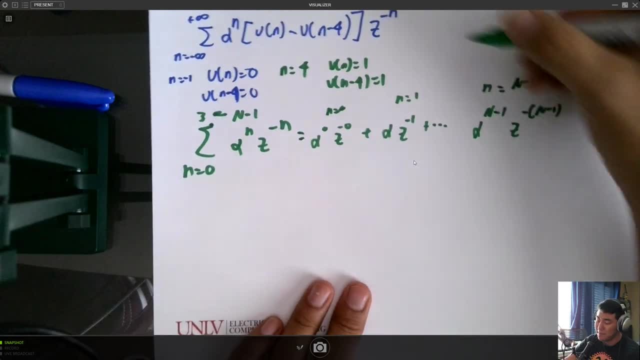 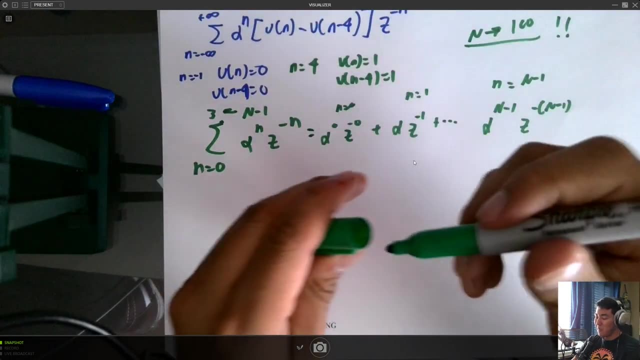 And you're like, okay, why didn't I just write the whole thing down? So what if n goes to like a big number? I can't do that, that's too big. So what we want to do is we want to find a little technique to make this simpler. 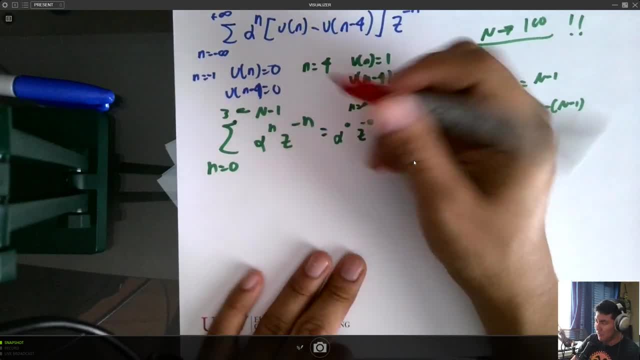 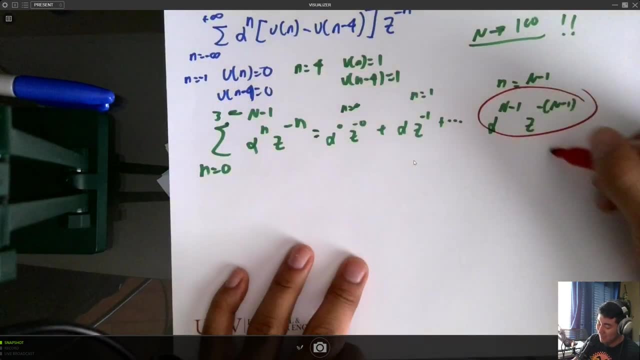 So there's a little trick I wanted to show you. Well, it's not a trick. You see this pesky term right here. What if we wanted to multiply this whole thing by alpha and z to the minus one, so that we can get rid of that and that? 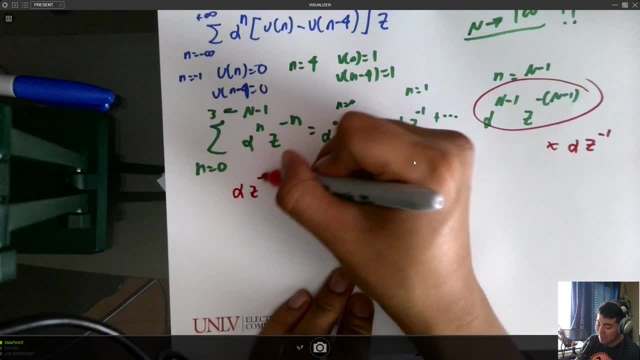 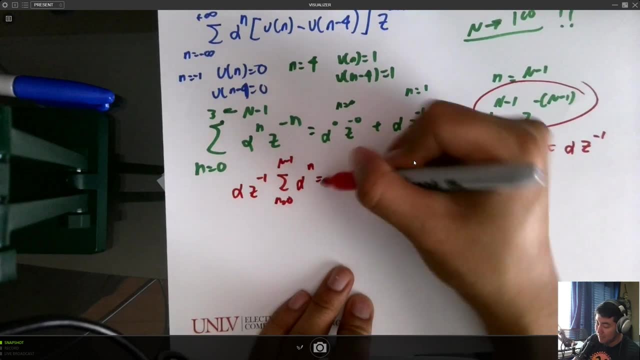 So we can do that. If we were to do alpha z to the minus one of that whole thing, n minus one, n is equal to zero. of alpha of n, z to the minus n is equal to. well, we get this. one is one alpha. 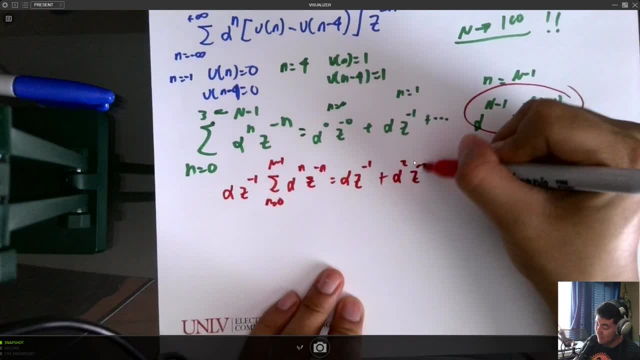 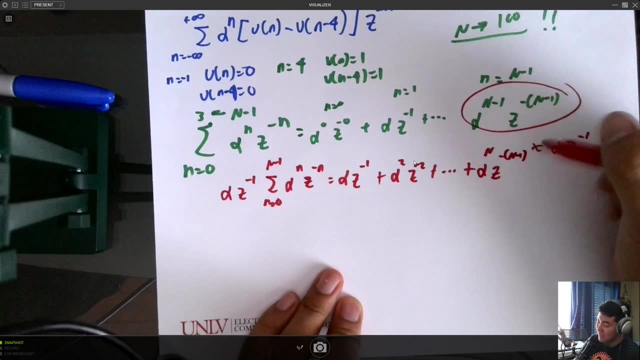 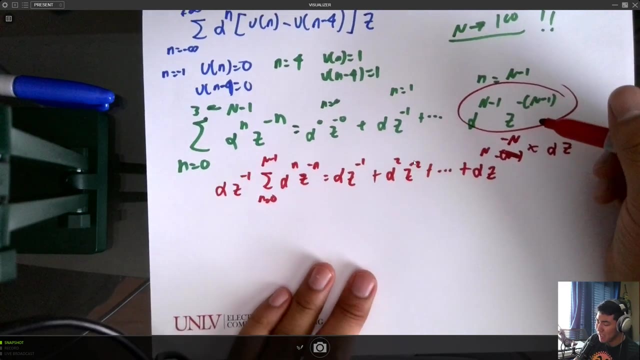 z to the minus one Plus alpha two. z to the minus two plus alpha of n. z to the minus n minus one. So there, oh no n, there you go. So that gets rid of that n term. 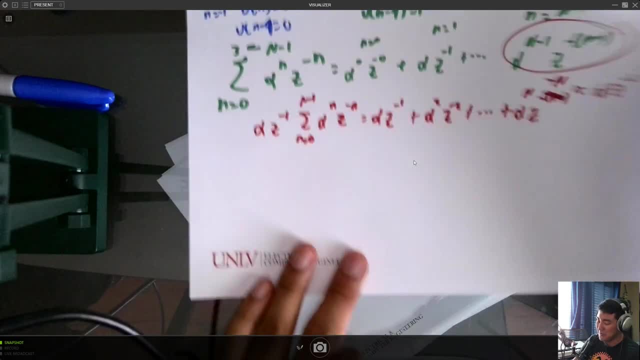 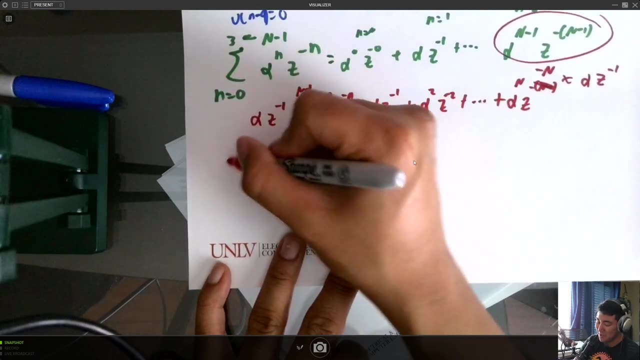 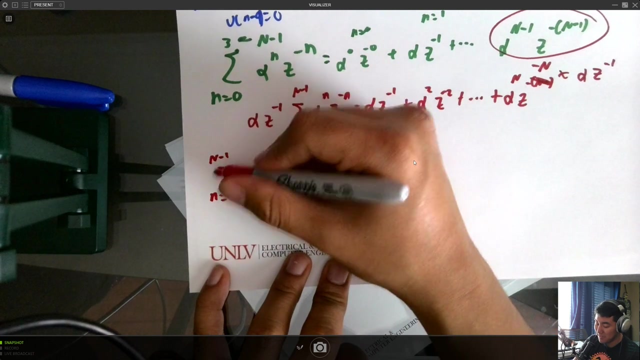 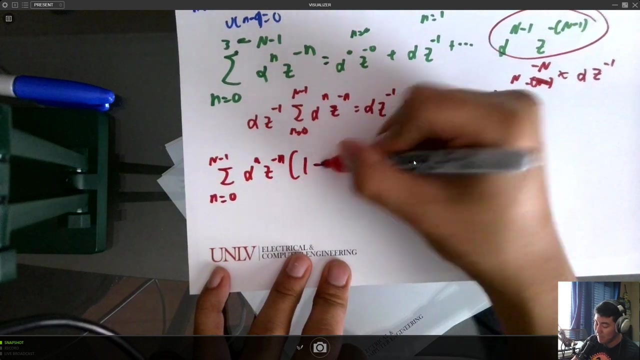 And then you're like: okay, and now, what do we do? So there's a cool thing, What if we took this guy this right here and subtract it with that? So if we do the following this: Okay, So if we do this: n minus one, if we took this alpha n z to the minus n of one minus. 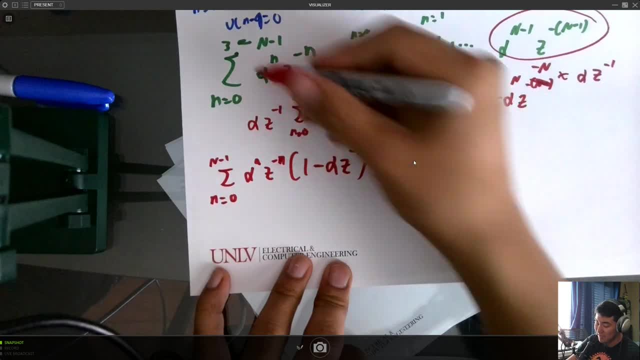 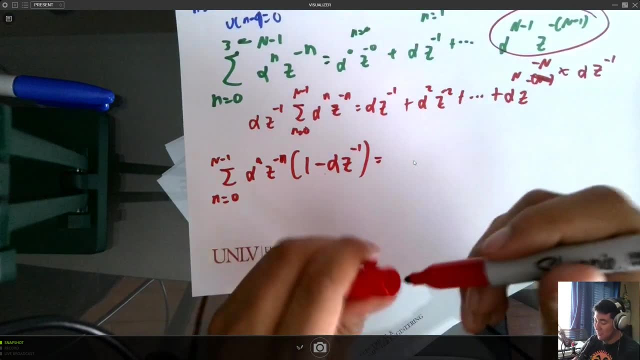 alpha z to the minus one. so we're taking this first term and then minusing this cool term which is going to equal. well, let's just do that mathematics to show you, guys, what's going on. So we're looking at this term right here. 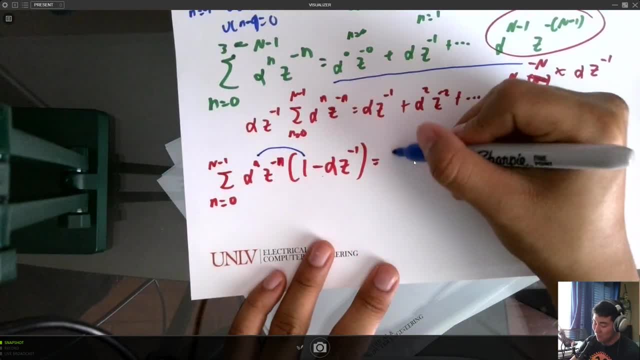 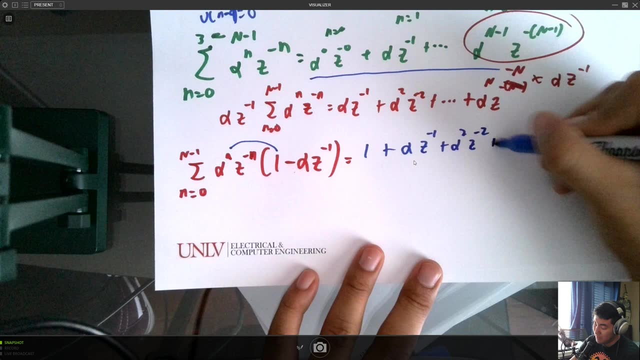 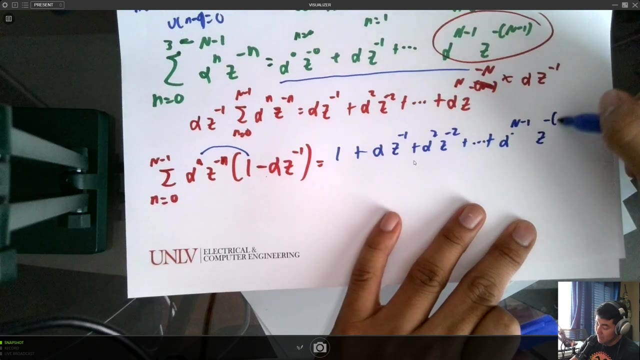 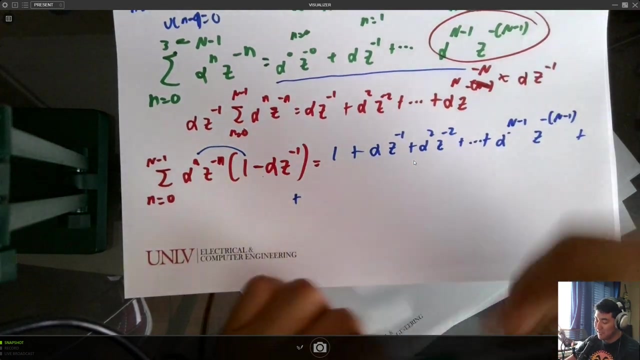 If we do one times this, we're going to get, well, one plus alpha z to the minus one plus alpha two z to the minus two, plus alpha n minus one z to the minus n minus one plus plus. now we're going to do this term, so we're going to multiply this to this, which. 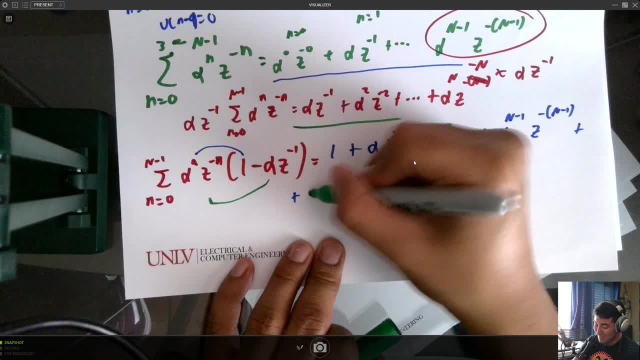 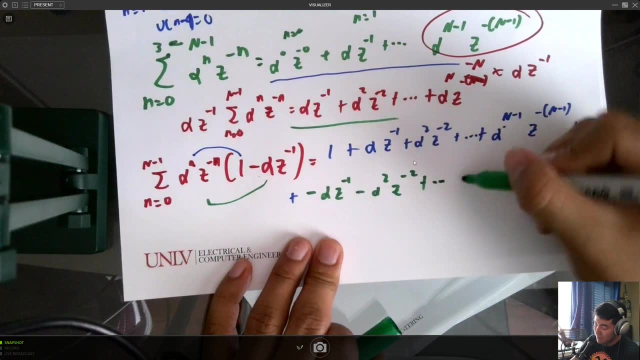 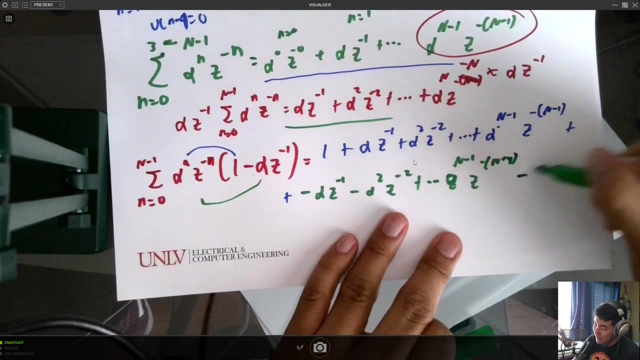 we already did. It's this right here: Minus alpha of z to the minus one, minus alpha two z to the minus two. plus alpha n. minus one z to the minus n, minus one. minus alpha of n z to the minus n. 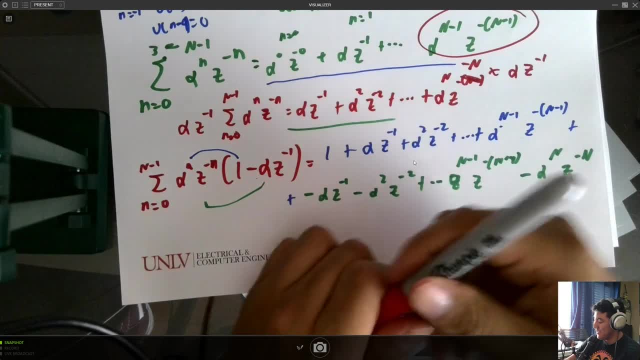 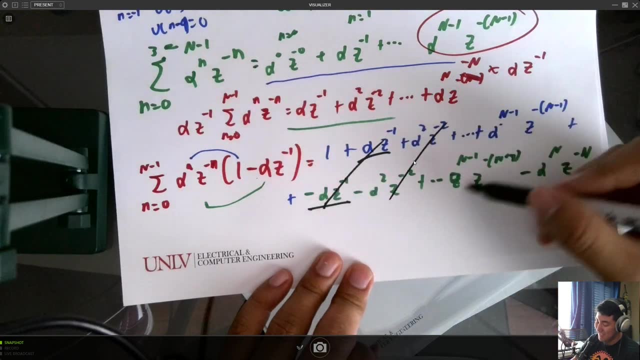 Then you're like: oh, I see a pattern. Suppose we did this. See how this term right here, this term here, looks similar. I can just cancel that All the way until we're done. Okay, We're left with this term right here and this term right here. 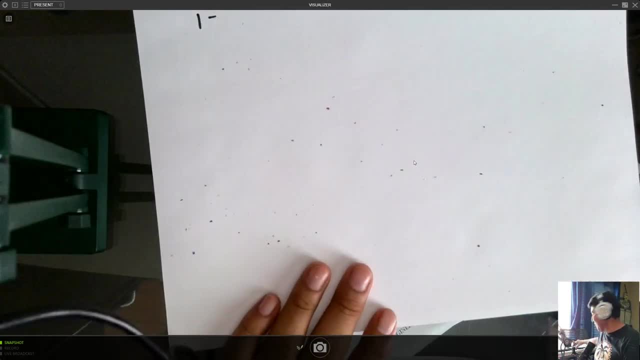 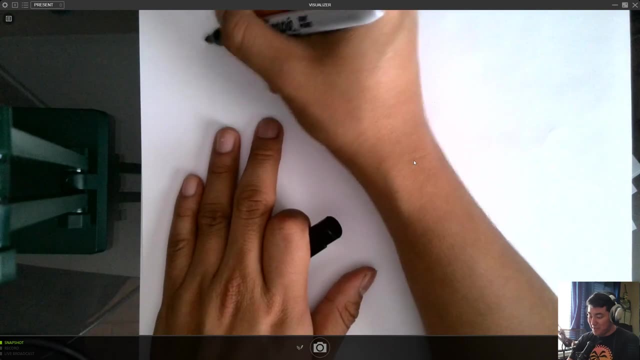 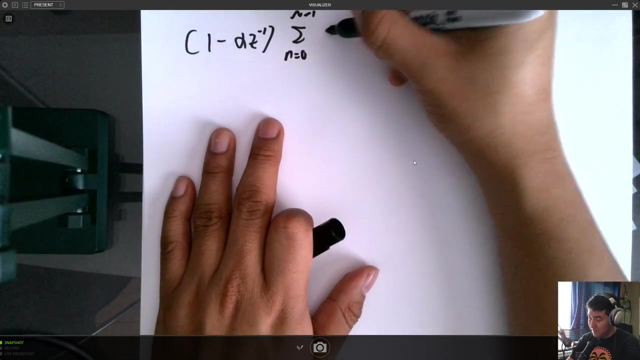 We're doing this because there's probably someone saying: I don't know how to do these systems at all. Don't worry, We're here to show you that. So if we wanted to put the final result, let's do 1 minus alpha z to the minus 1 n. minus 1 n is equal to 0 of alpha of n z to the minus n of 1. 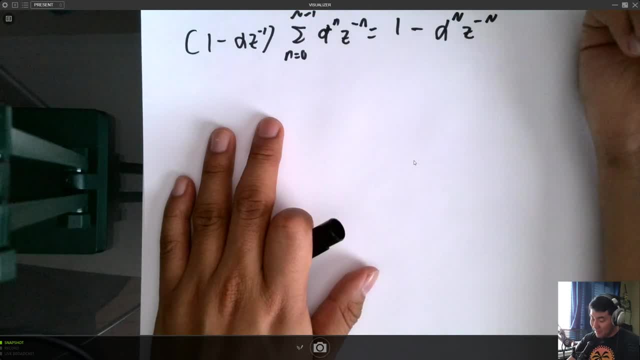 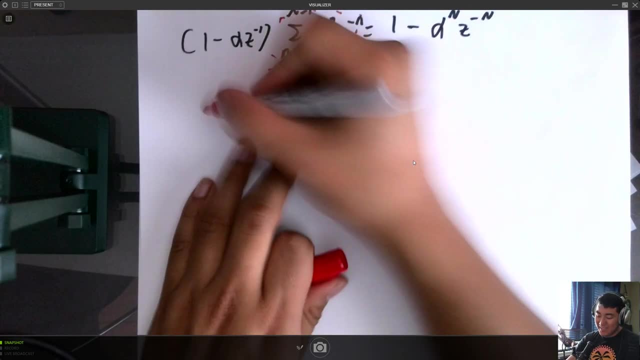 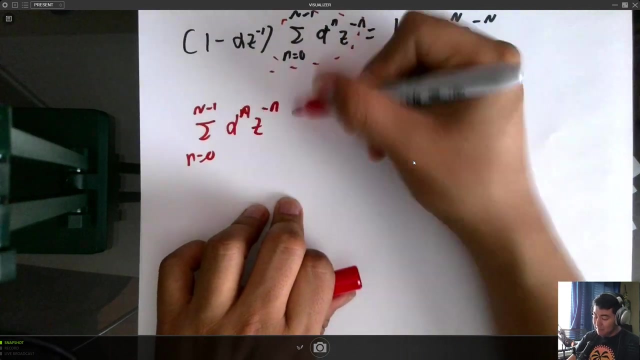 minus alpha of n, z to the minus n. There you go, But we want this. What we want is this. We want this. Ah, we can find that right now. 0 alpha of n is what we wanted to find initially. 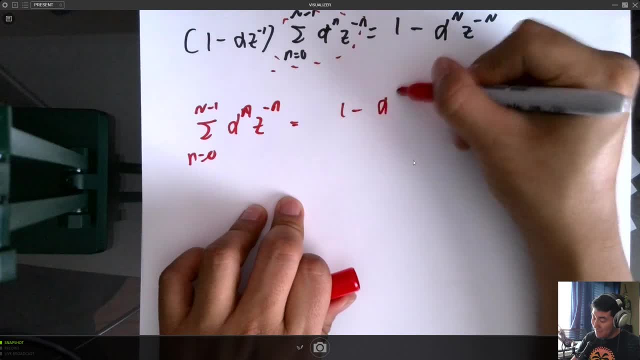 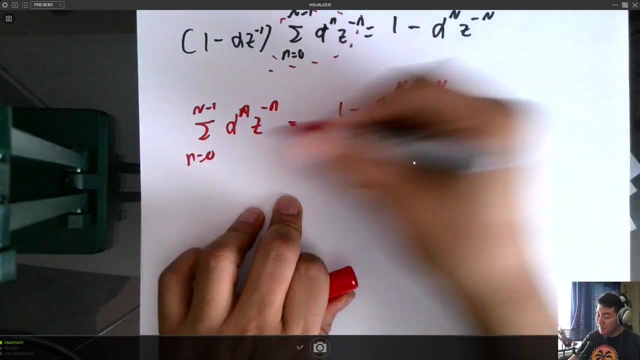 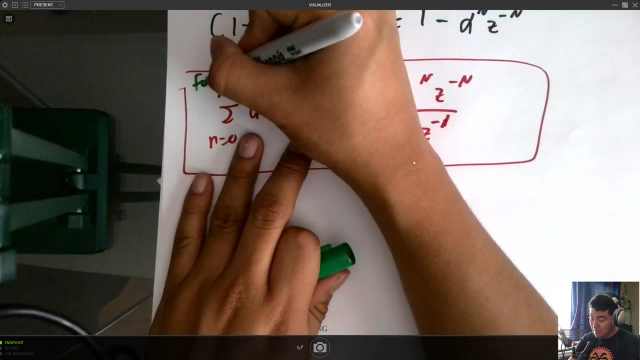 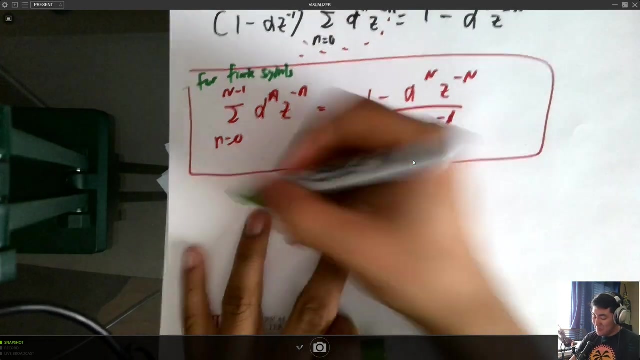 which is equal to 1 minus alpha of n z to the minus n, 1 minus alpha z to the minus n to minus 1.. And there you go. This right here is for finite signals. Now suppose that n goes to the number of elements that we have goes to infinity. 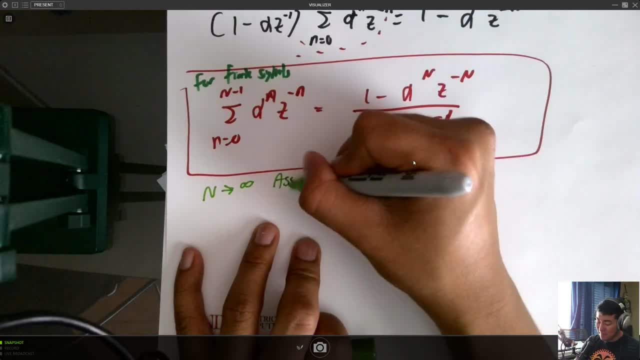 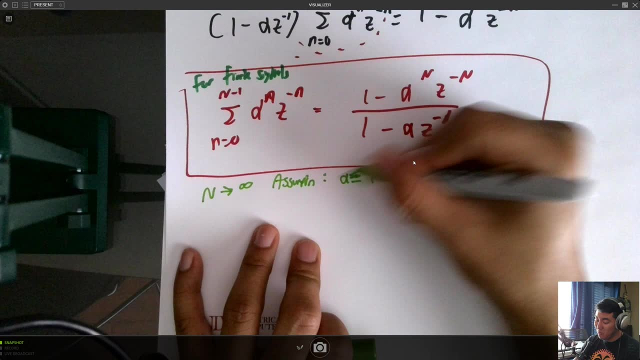 There's a whole bunch, There's an assumption. There you go. The assumption is that alpha should be less than or equal to 1.. Actually, the magnitude has to be less than or equal to 1. It has to be equal to that. 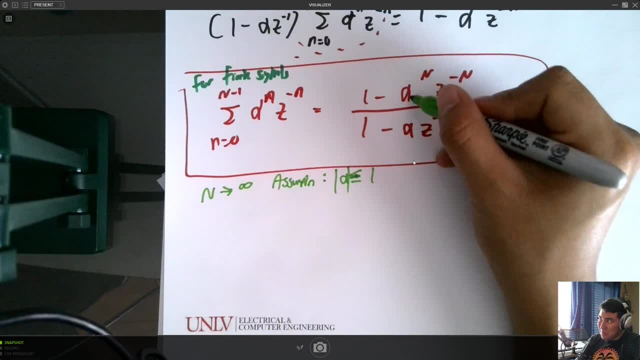 Because if we look at this term, if alpha is equal to 2, then we have 2 times 4, 2, 4, 8, it goes to infinity. This term goes to infinity blows up and we don't want that. 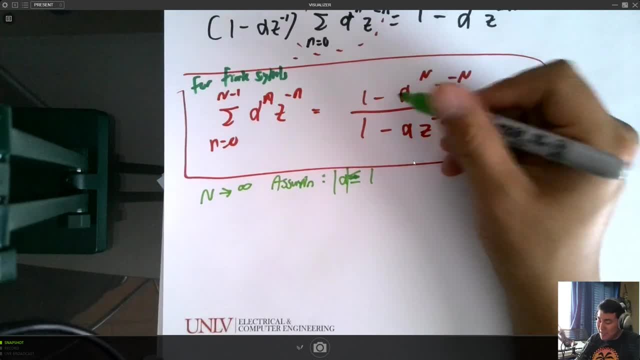 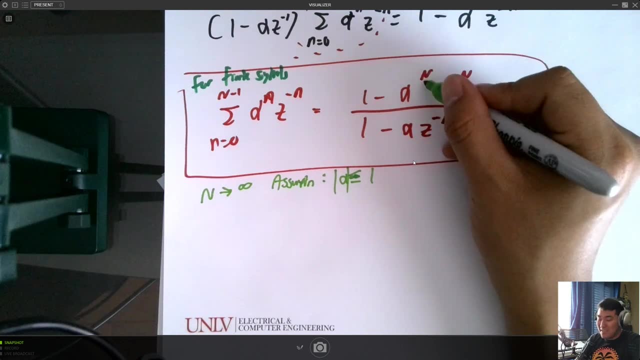 And this term actually dominates more than this. so, yeah, it goes to infinity. So if this were 0.1, then it's just 0.1, 0.01, it gets smaller as we go higher in n, So this actually disappears. 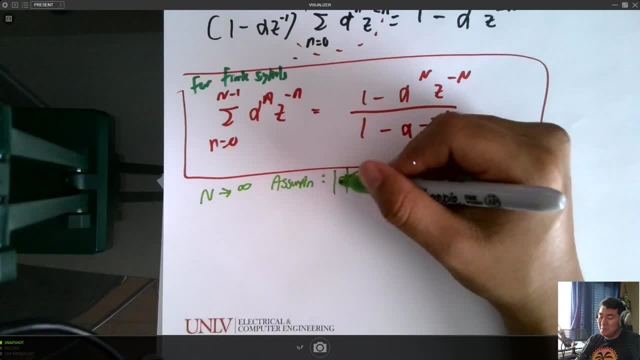 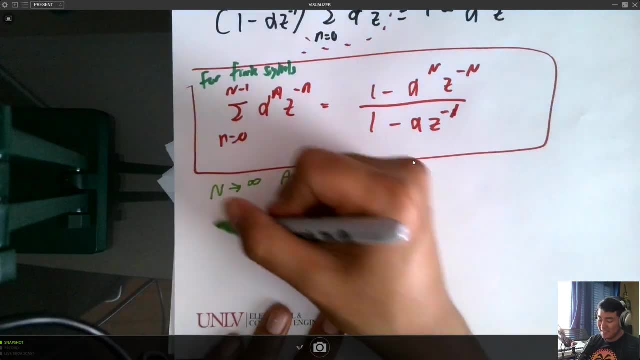 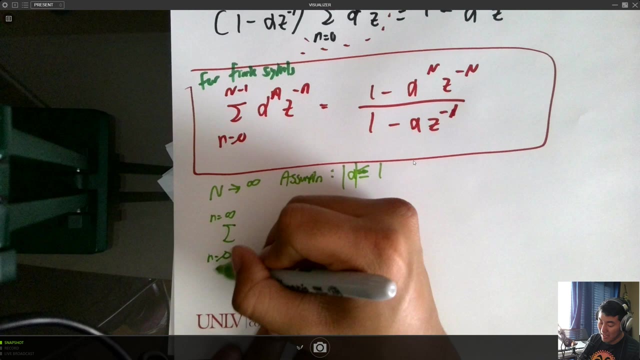 So the assumption is: alpha has to be less than or equal to 1, the magnitude. So if we took that into consideration for all general signals, then n is equal to infinity. n is equal to 0. Note: it has to be 0, right here. 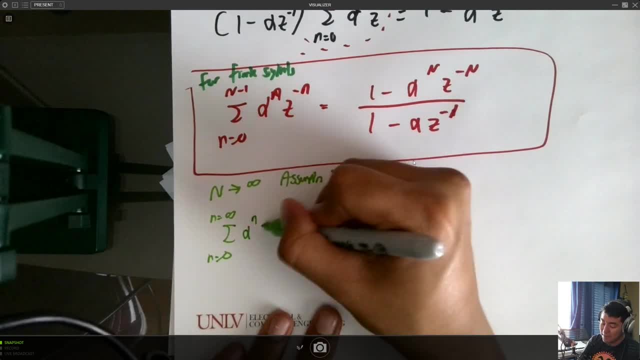 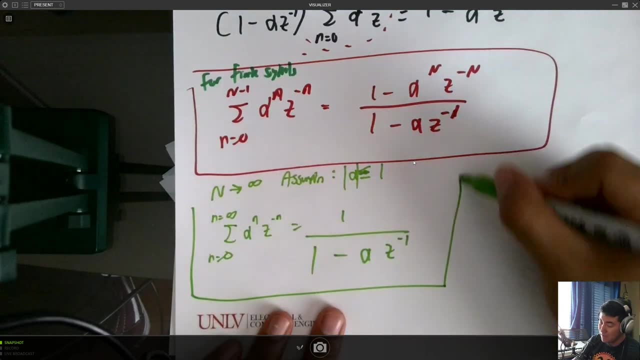 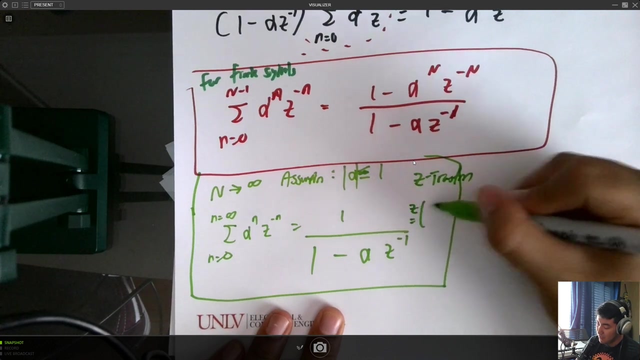 You can do shifting properties, if you need to, Of alpha of n. z to the minus n is equal to 1, 1 minus alpha, z to the minus 1.. And there we go. This is the z-transform. z-transform of x of n. 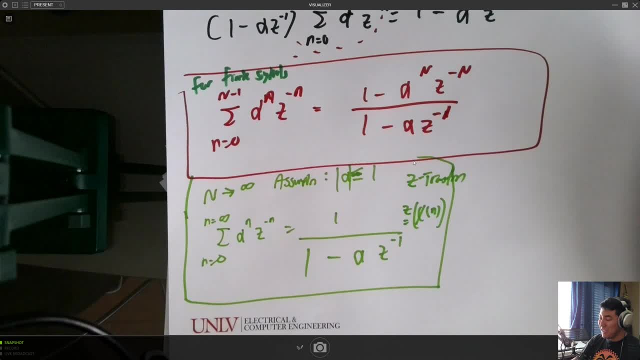 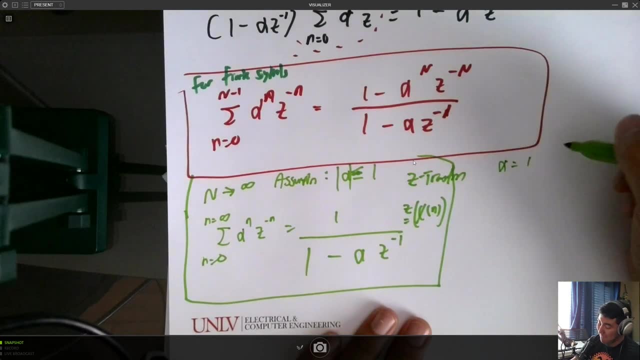 There we go. So now you're like saying, OK, if we were to go back to our thing, what if alpha is equal to 1?? What if alpha is equal to 1?? So if we were to go to the time domain? 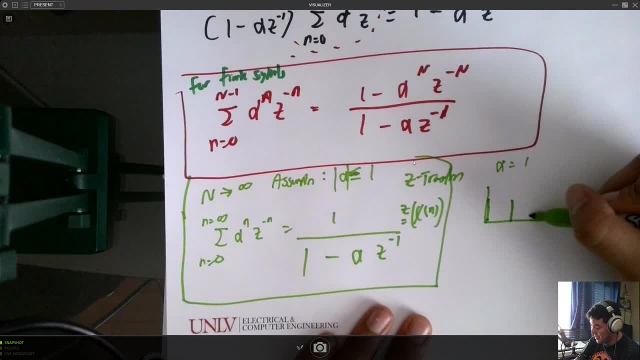 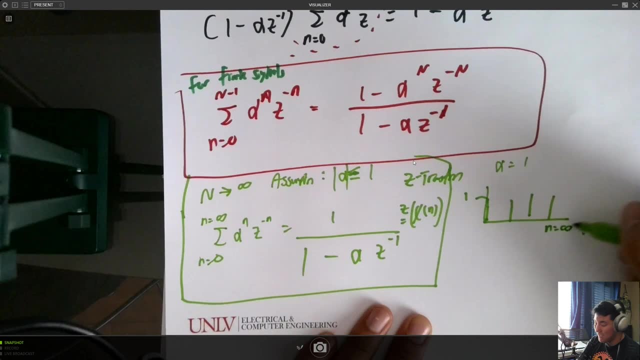 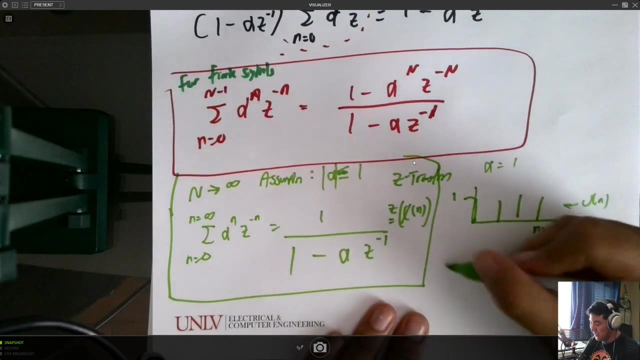 the n domain, then we see that if we just plot these points, if we have a constant magnitude of 1 and it goes to n is equal to infinity. what's that? It's a unit step. So that means unit step. So that means, if we wanted to do, alpha is equal to 1,. 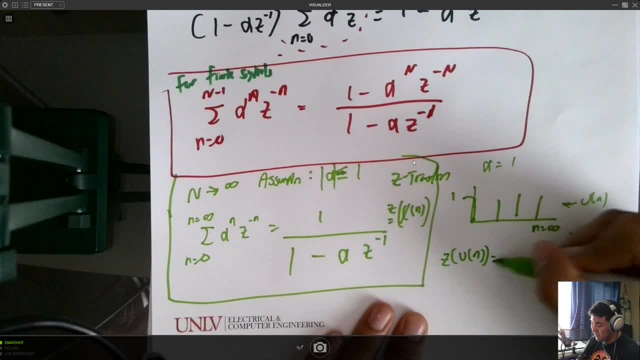 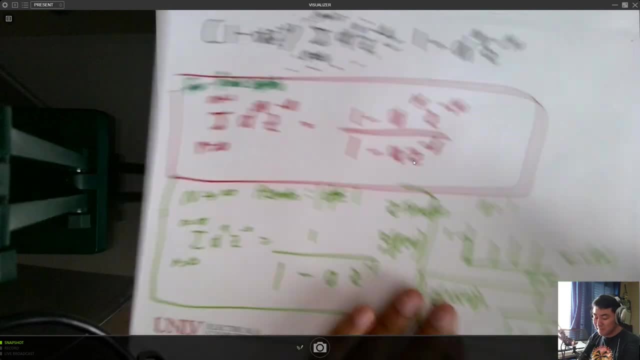 that means we're actually doing the z-transform of the unit step, which is equal to 1, 1 minus z to the minus 1.. So that's a little thing I wanted to show you there. Hopefully that clicked into your brains. 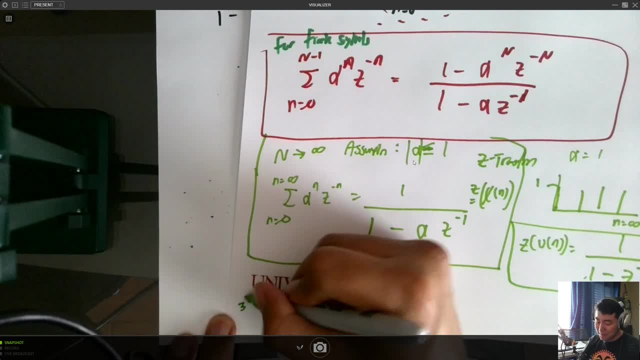 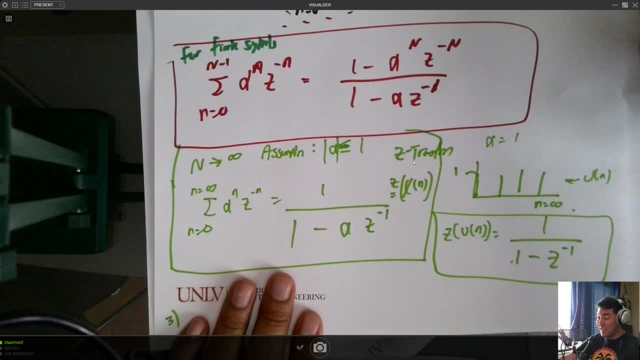 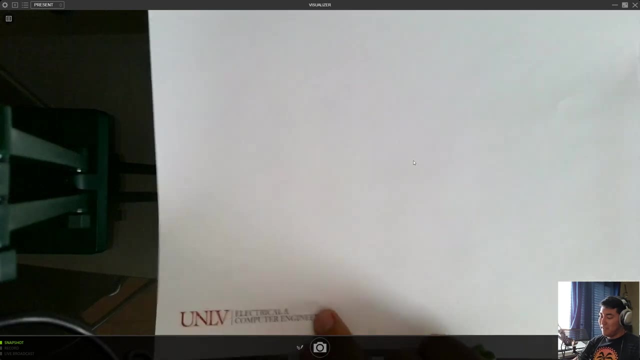 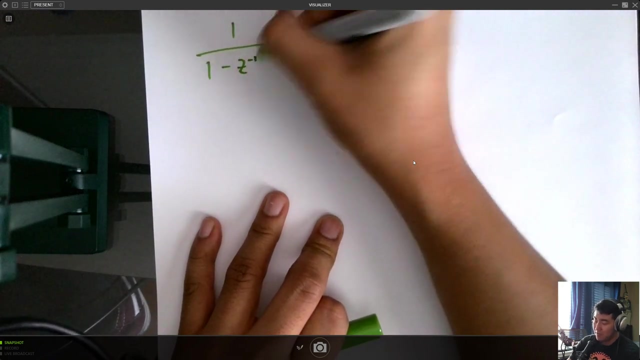 And let's do the following three. There we go. Now we want to say, OK, what do we do? The next thing I got to show you is z-diagram, z-plane, the z-domain. There you go. So let's bring back our system: 1, 1 minus z to the minus 1.. 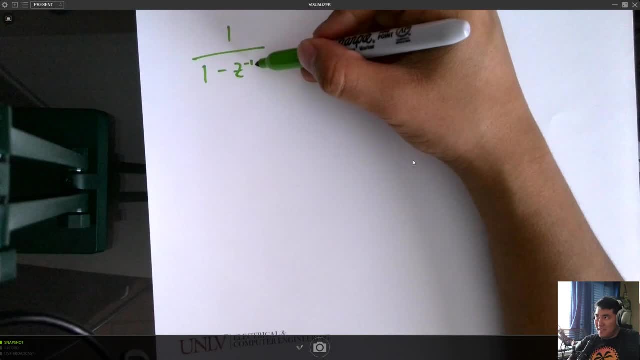 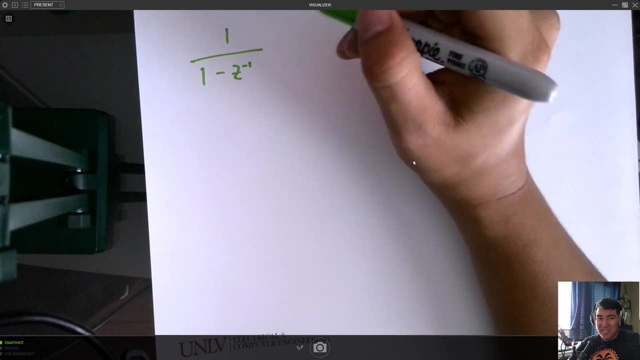 I want to ask you this: Where does the system well, where's the poles and the zeros? And you're probably saying, oh, we can see the pole. But I'll tell you now. there's actually one thing you got to do and I will be checking for this on your assignments. 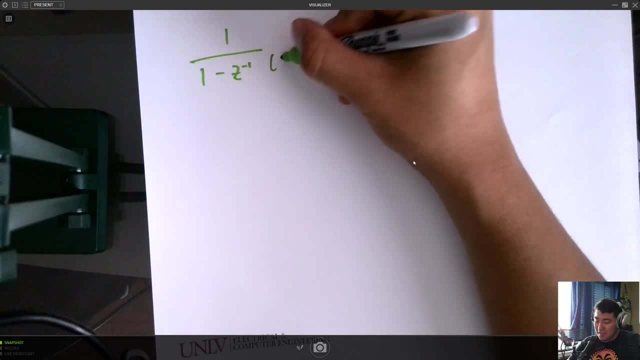 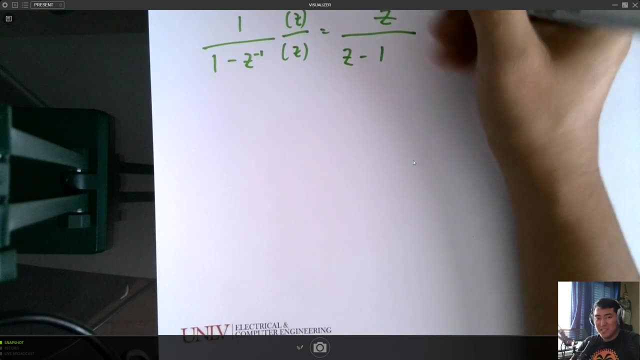 You actually have a zero in here and you're like saying: what? how? If we multiply this by z, you notice that, and I think this actually is easier to see. So if you wanted to see where the actual zeros are, that's where it pops up. 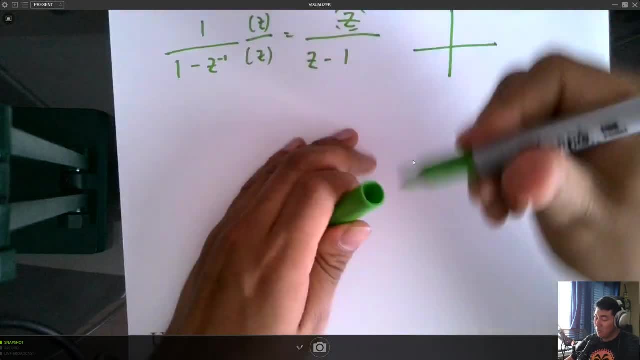 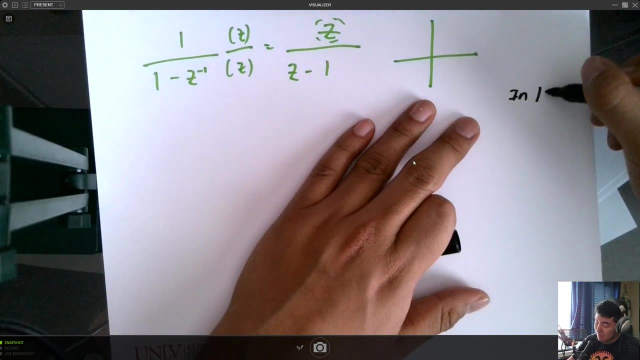 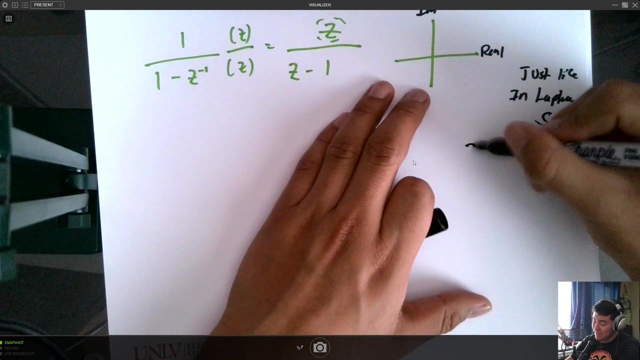 So the z-transform of this system is: well, where do we have a zero? Zero, just like in the s-domain, in Laplace. Well, just like in Laplace s-domain, we can plot the real and the imaginary. Z is actually going to have some real component plus some imaginary. 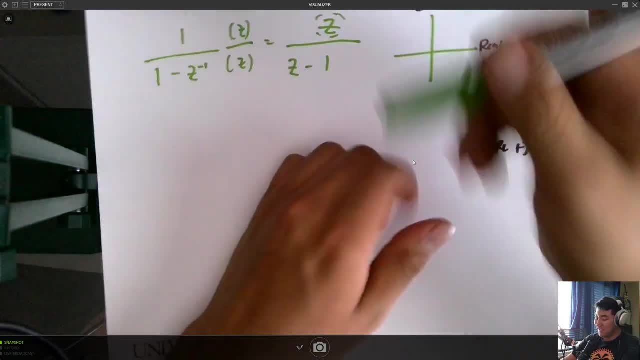 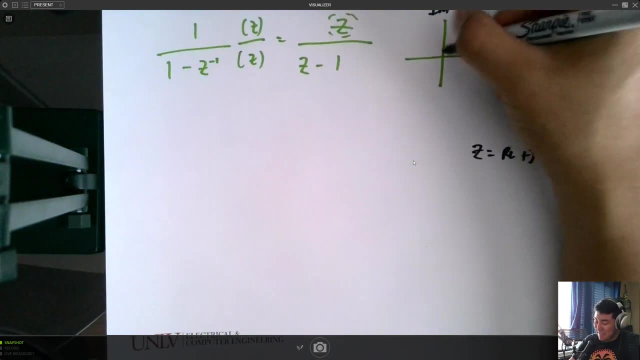 So if we were to look at this system right here, well z is going to equal to zero, The zero is going to be zero. So that's really easy to plot. There you go, And then the pole. we notice that if well z is equal to one, that's a pole. 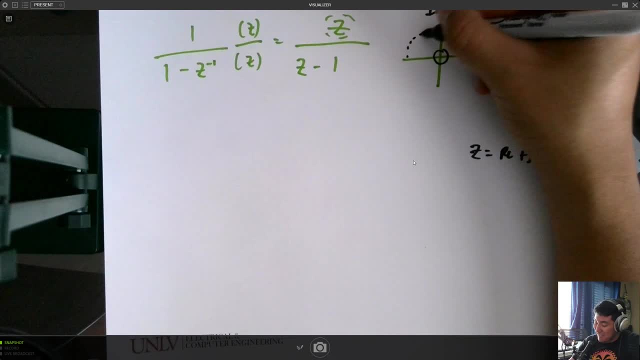 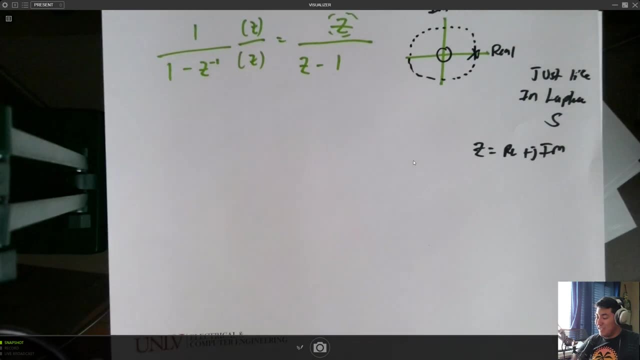 There you go. So one last thing I got to show you is the unit circle, And that's how you would draw your little diagrams. And now you're saying: well, now we have this system, Now, what else can we do with it? 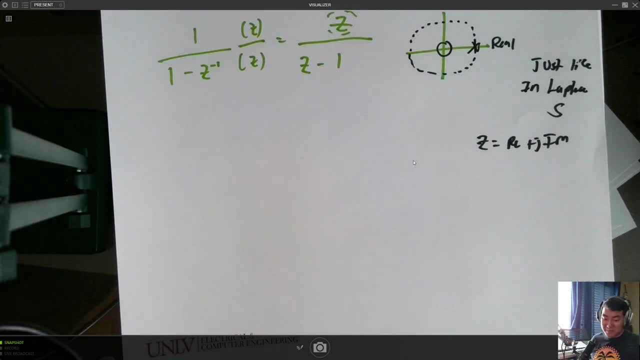 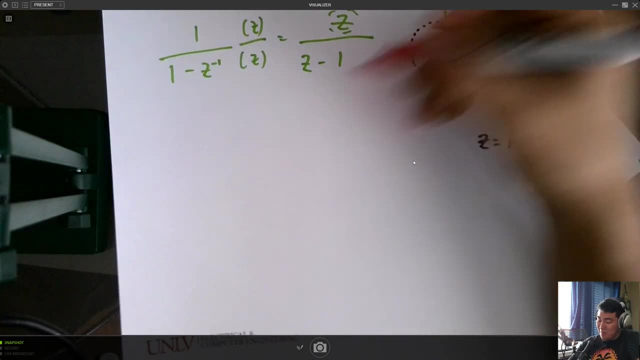 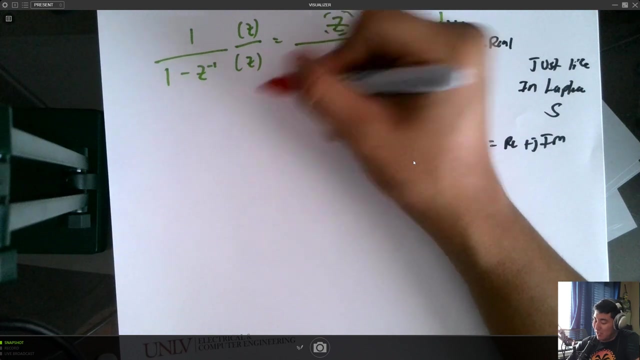 Next thing I got to show you is the residue theorem. And the residue theorem, just like in the Laplace transformers, What's the transfer? or if I were to say: well, in reality, instead of z to the n we're actually looking at. 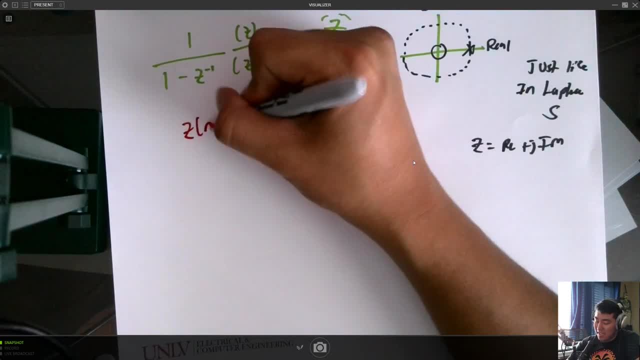 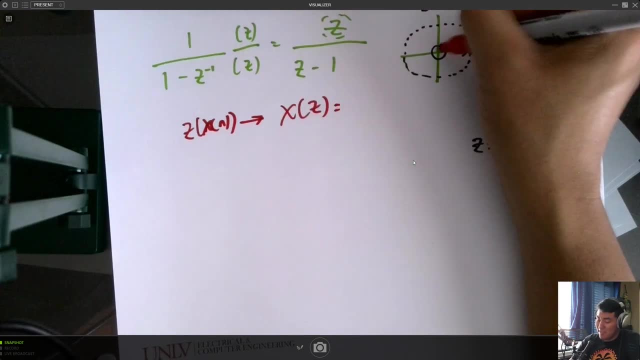 x of z. So the z transform of x of n results in this. So if I wanted to look at this system, what's x of z when z is equal to zero? It's zero. The magnitude is zero, It's just zero. 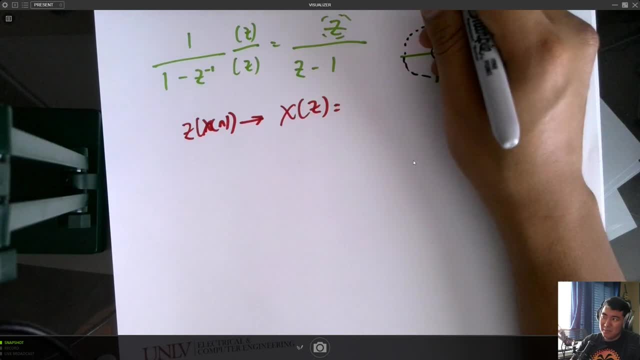 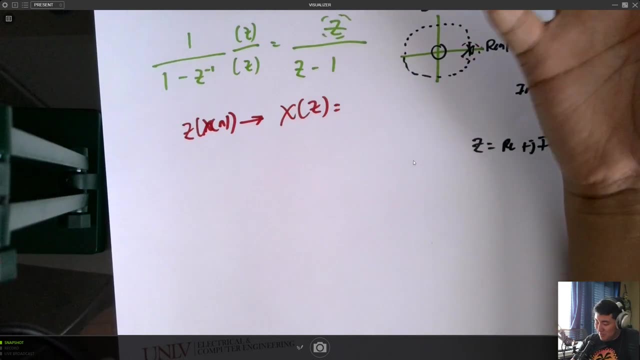 But what if we're at the pole? What do we do if we go back into the time domain, the n domain? What does that result with? So if we look at this pole we got to look at, well, what does a residue do? 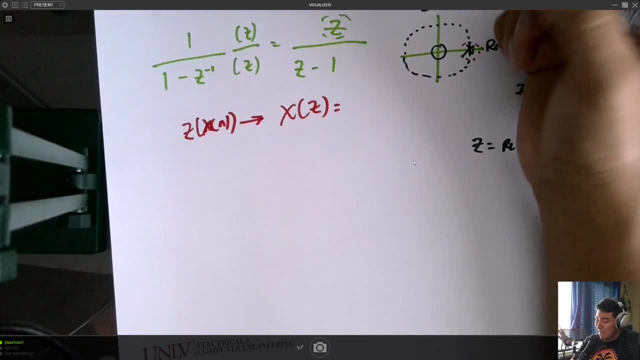 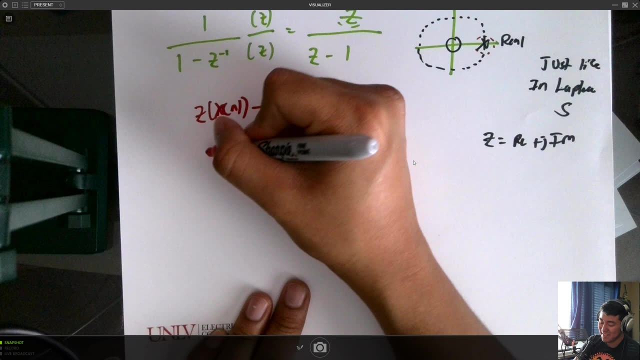 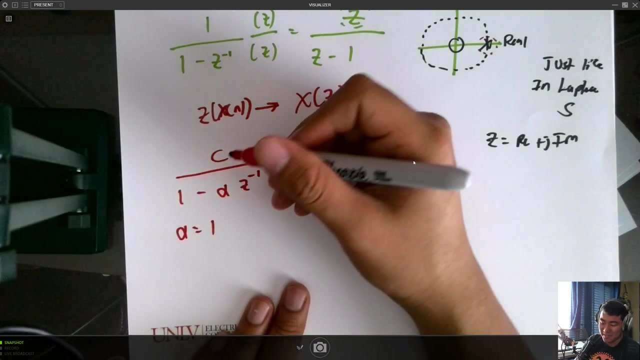 What's the residue of that pole? So one thing I wanted to show was: well, with the unit step, suppose we had a constant c and one minus alpha to the minus z to the minus one. If alpha is equal to one, that's our unit step. 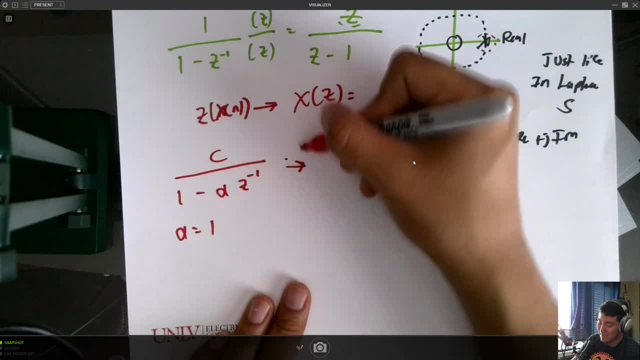 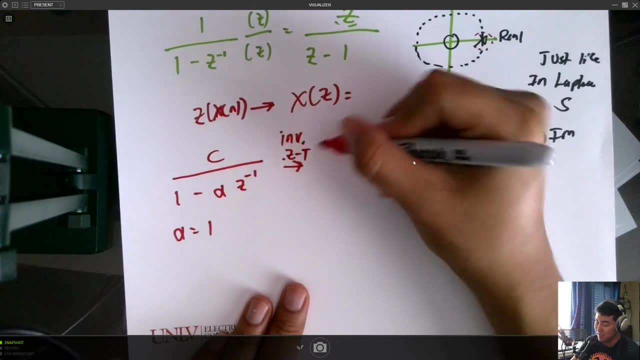 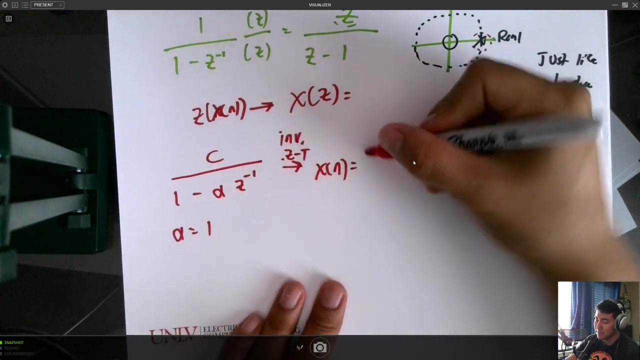 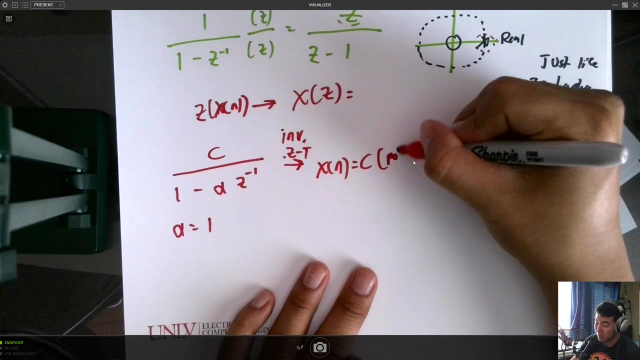 But if we have this pesky c, the inverse z transform is going to equal to. let's just call it: x of n is equal to c, because that's a constant: the pole. what's the pole value? Pole to the nth power. 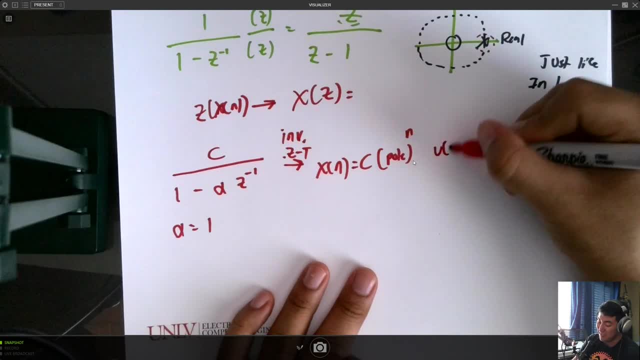 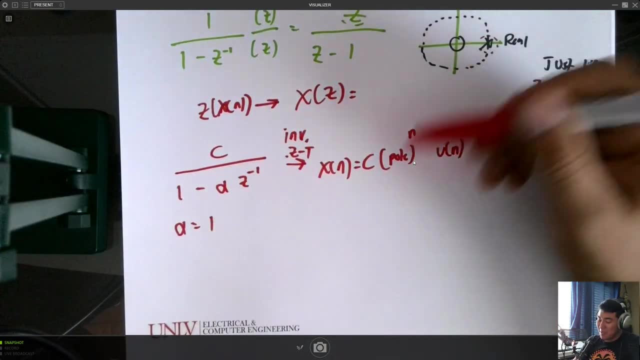 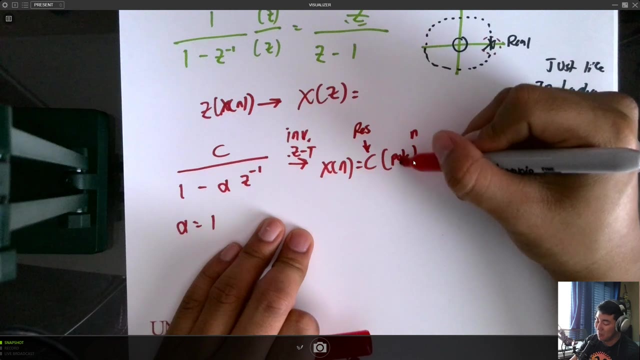 And that's it. But for causality we want to add that right there. So the rule is, if we look at every pole we can just do: oh, whatever value the residue is, a residue times the pole to the nth power. 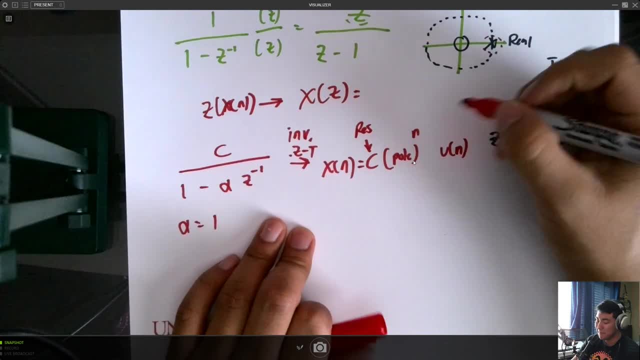 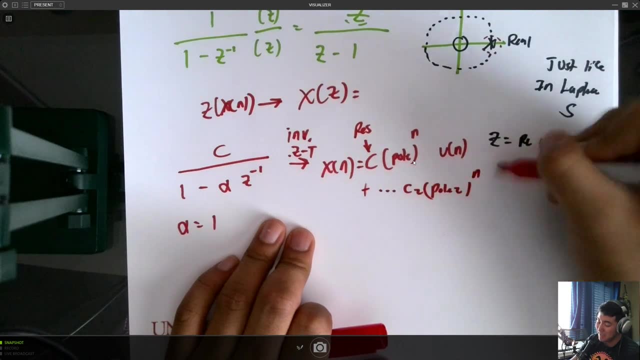 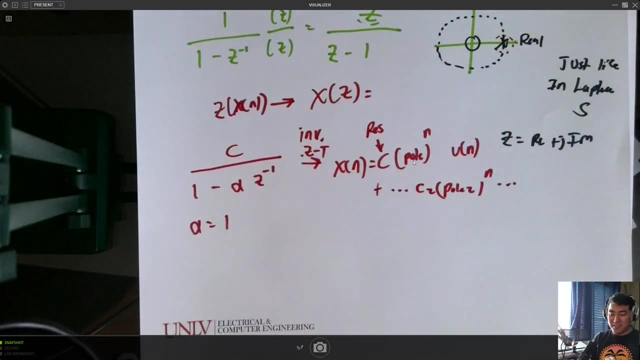 the pole to the nth power and then times u of n to make a causal. So that's the theory plus c2 of pole two, depending on how many poles you have. So that's what we wanted to do. So to demonstrate to you this, 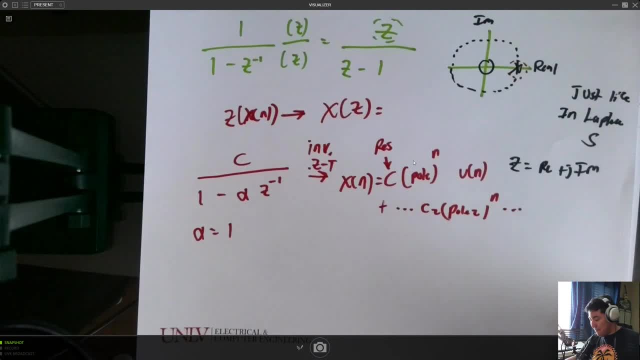 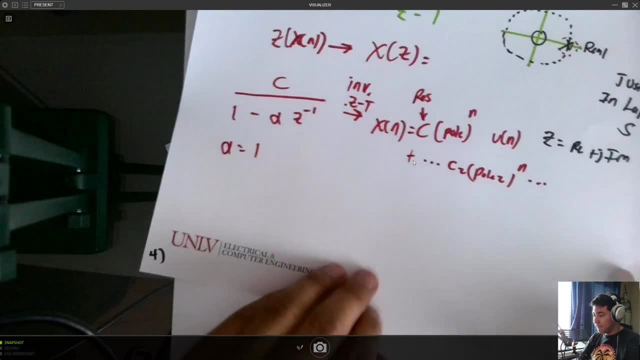 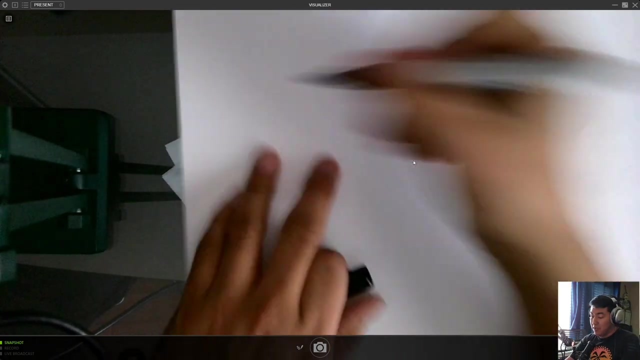 let's show you another quick example. This right here is four, And we'll start with: let's just build a system, Let's just choose a random system, And the system I want to do is, well, just pick a pole right here and it's on the unit circle. 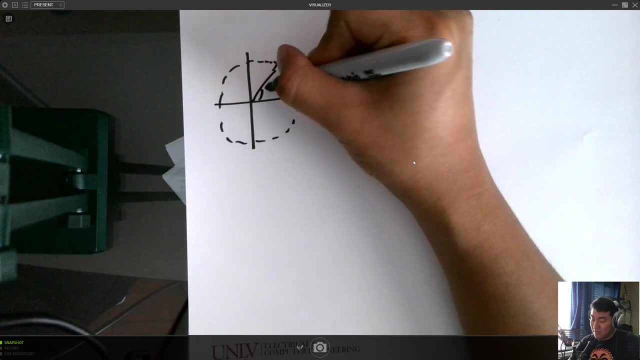 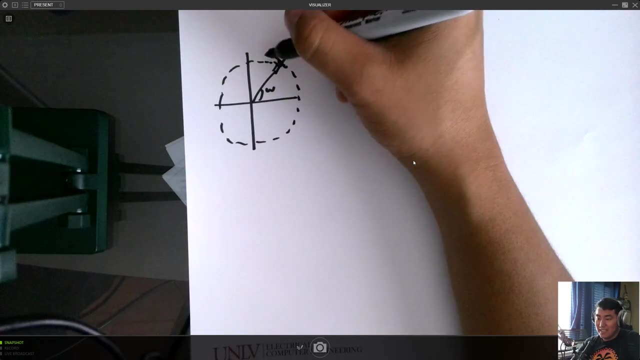 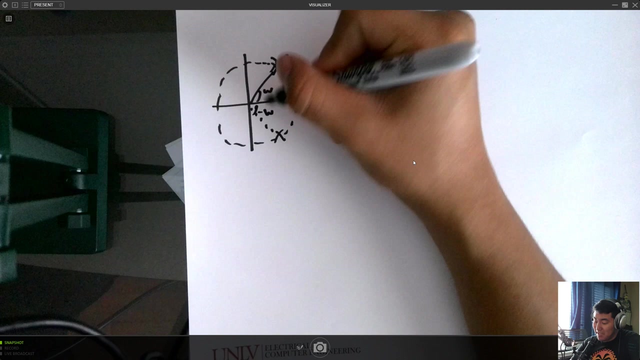 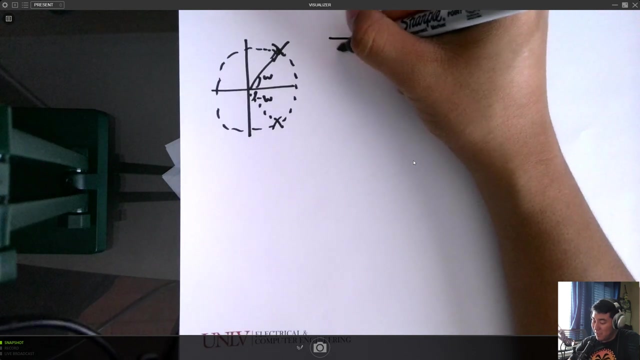 OK, And let's just choose this as omega. So the thing with poles being on the imaginary part of the Z-transform is you have to have a complex conjugate at the same, minus frequency, minus omega. So where this is. well, if we wanted to mark that pole. 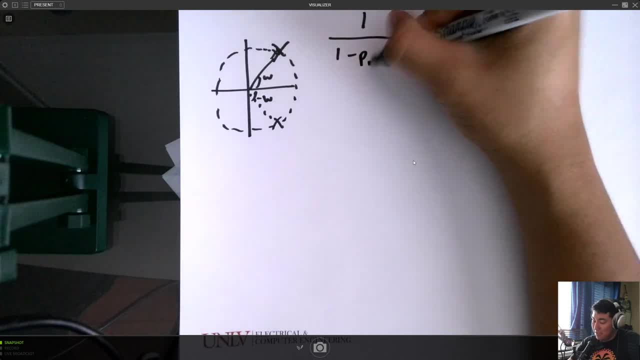 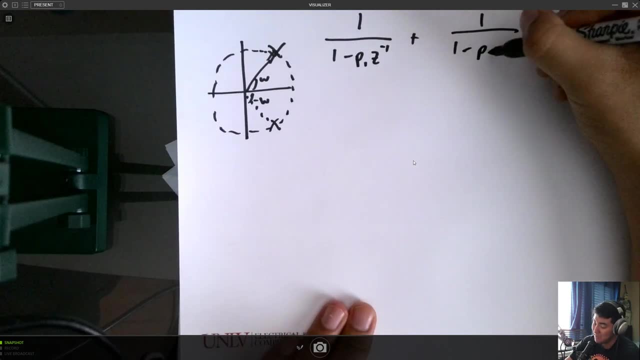 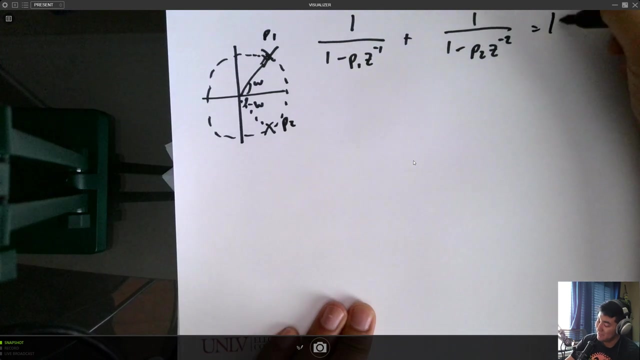 one minus. well, the pole value z to the minus one plus one, one minus p, two, z to the minus two. This is pole one, pole two, And if we multiply this, actually this is equal to- let's just call it- h of z. 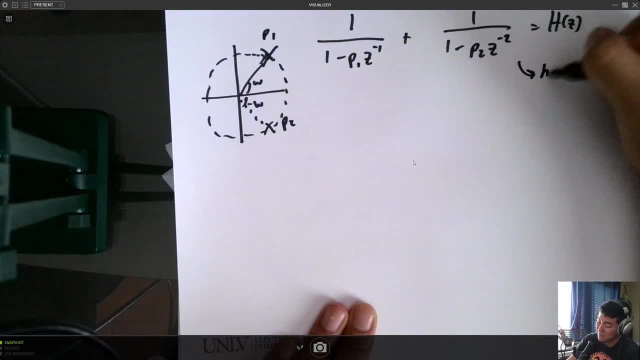 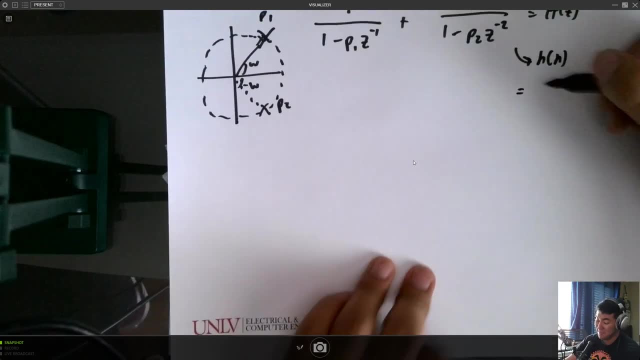 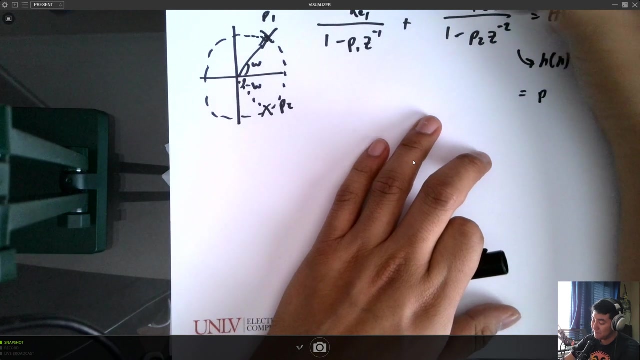 So if you wanted to take this into the inverse transform, it's really easy, It's not that bad. You just add these terms and you're done. So if you wanted to go, actually let's show that right here. P actually let's do re one, re two. 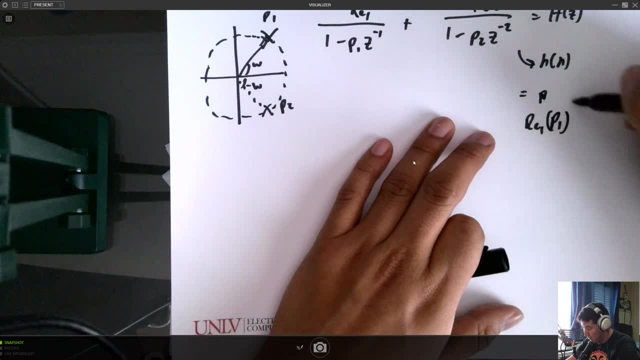 Re one p one plus re two p two. All this to the unit step. Don't forget the unit step. If you don't put the unit step, you will get marked a point off. Well, not for me, the exam. 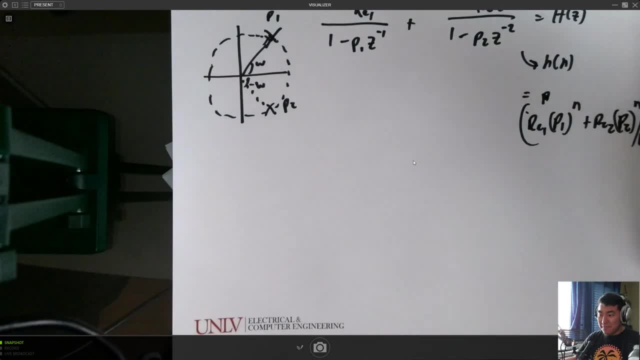 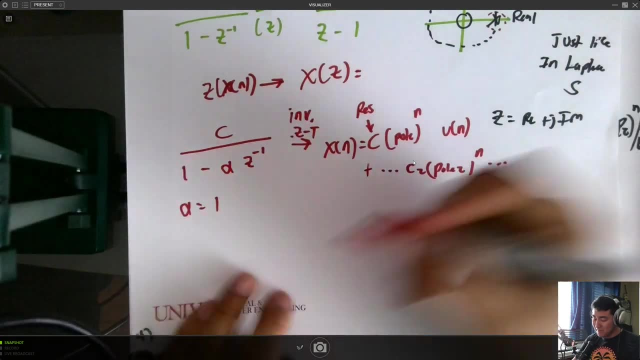 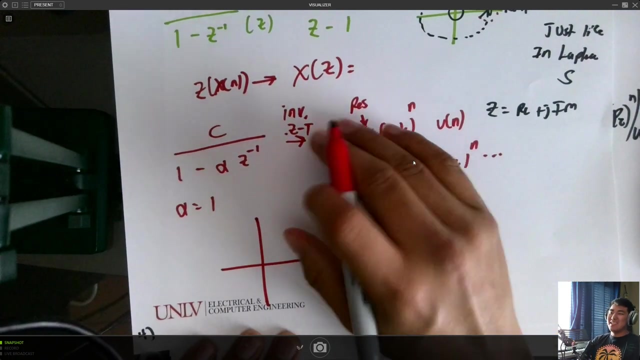 Just giving you a quick hint, because we want to have stable systems, cos one stable systems. OK, if you want me to give you a quick note on that, if you recall that I just said: oh what if alpha, like alpha, has to be less than? 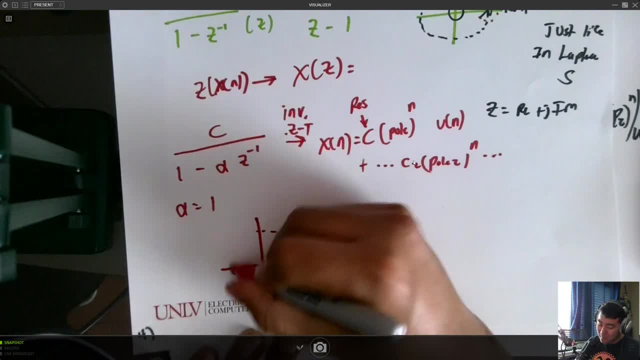 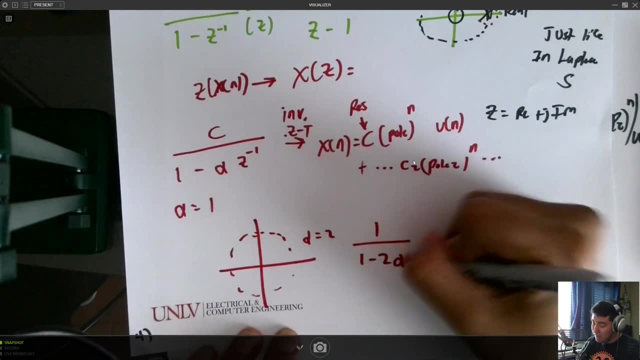 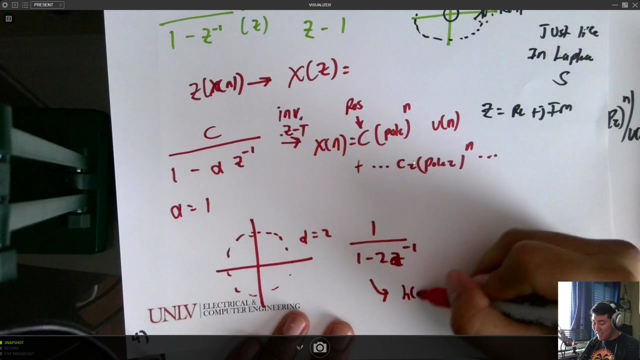 or equal to one. what if alpha is equal to alpha is equal to two? let's say So that means the pole one over one minus two, z to the minus one. If we wanted to turn this into that real domain, h of n is equal to two to the n. 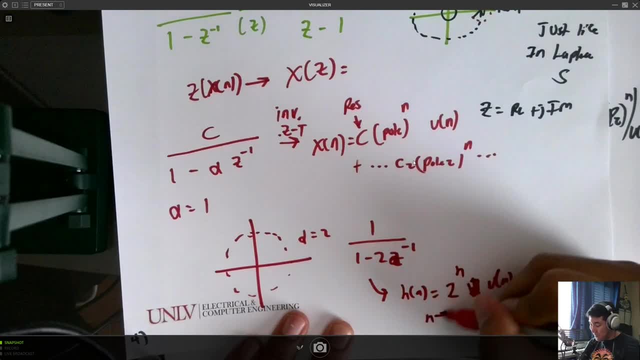 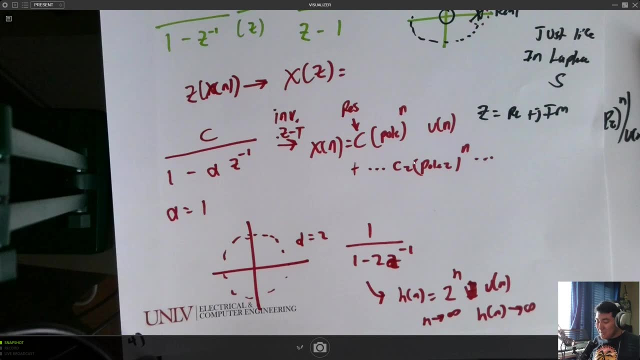 two to the n? u of n. You notice that if n goes to infinity, then h of n goes to infinity. That's unstable, It's well, it just blows up. So we want to look at the region, the convergence. 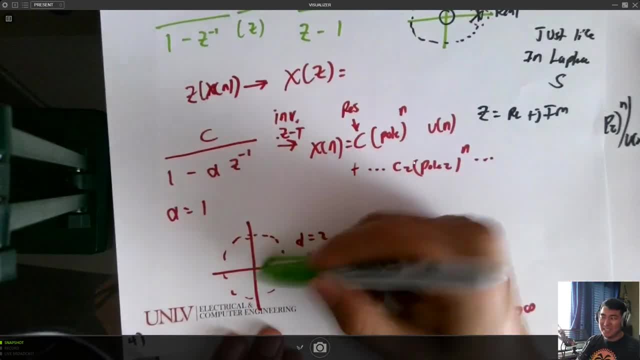 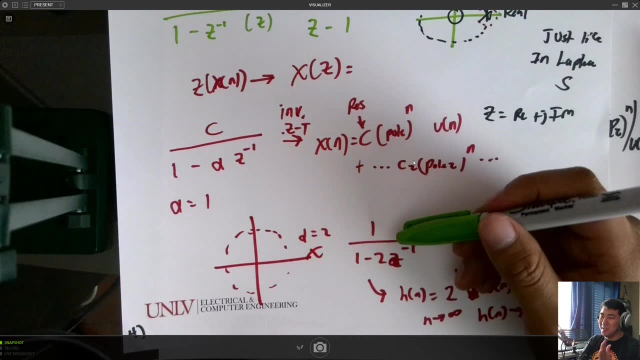 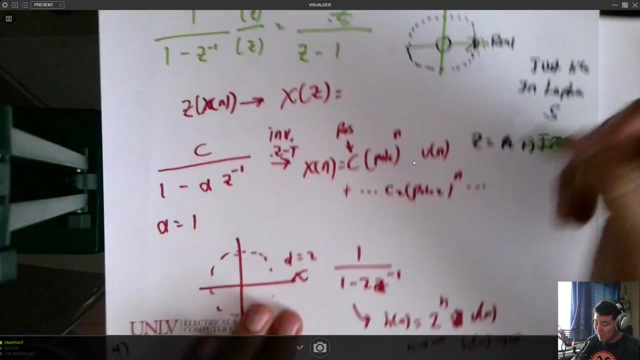 And that is well. the first thing is, all the poles have to be inside the unit circle and we have to look at the farthest pole, the farthest pole from the center, So everything outside that far pole. So if we wanted to look at this system, 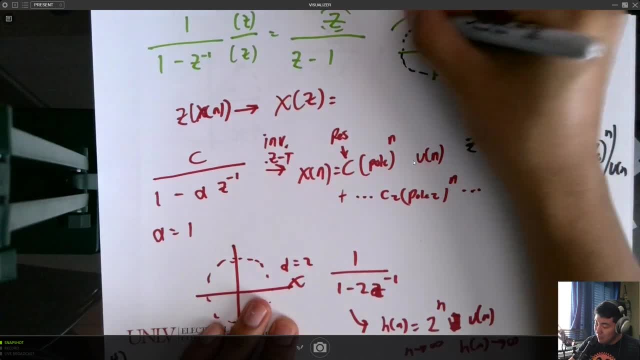 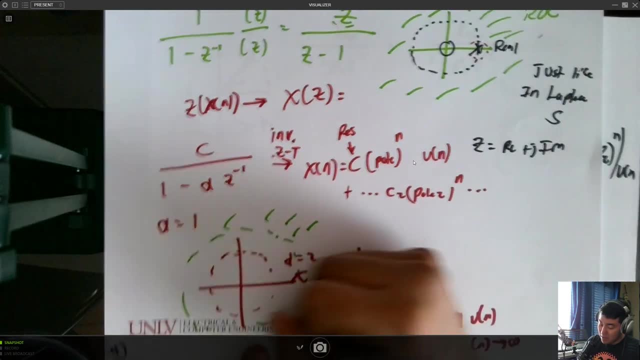 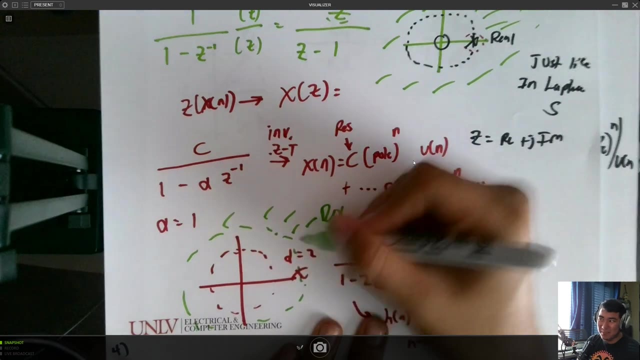 then the region of convergence is this whole system And then the region that converges. here you can do. you can do this if you wanted to. Oh, you got a big donut there, ROC. However, it's not stable. So this is a causal but not stable system. 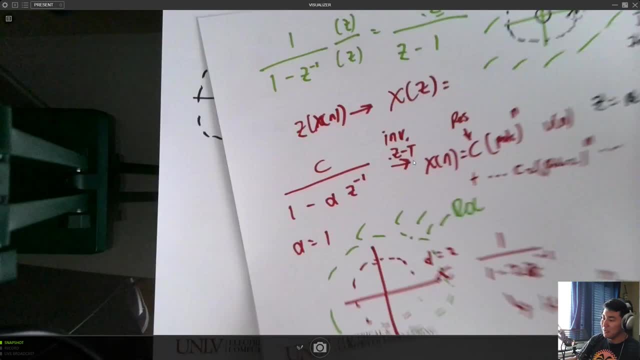 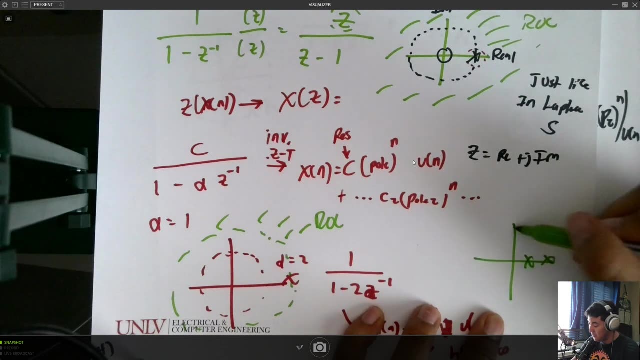 So it's not going to work. If you were to look at this example right here- actually, let's look at the system right here- If I had a pole here and a pole here, here's the unit circle. You know that it's a stable system, that all the poles are inside. 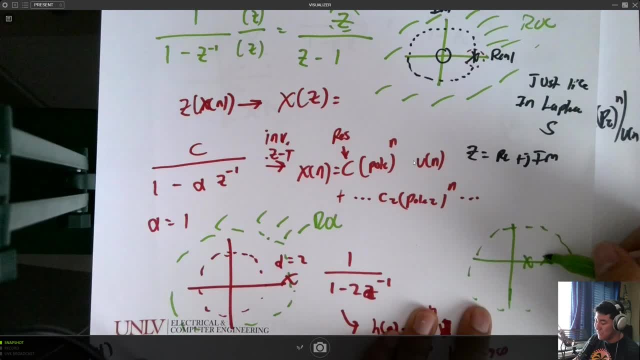 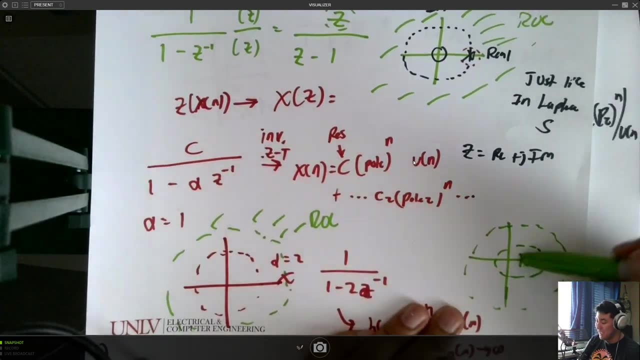 However, now we got to choose our region, the convergence- for it to be stable. We have to choose this so that we can have a stable system and a causal system too. We don't want any poles in our region of convergence. That's not good. 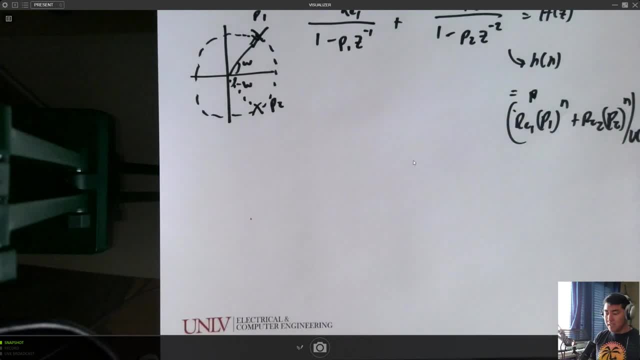 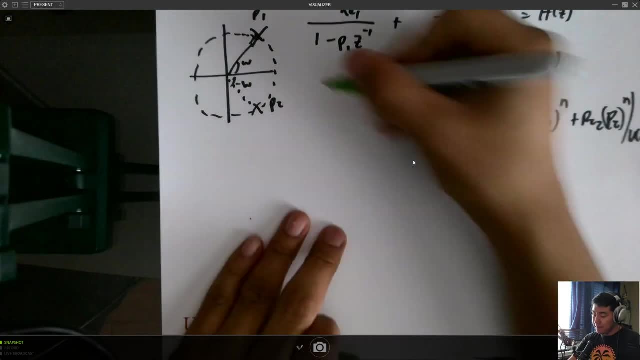 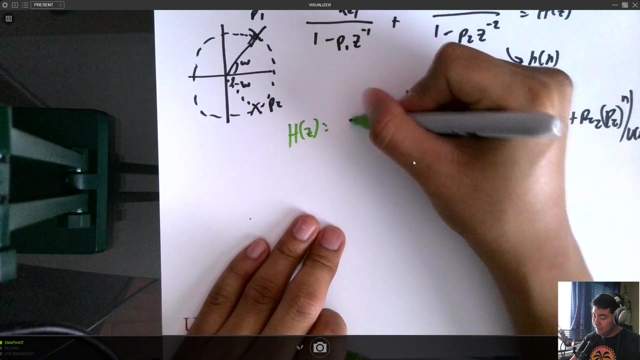 So it's a quick note I wanted to make there. So now you're saying: well, what do we do? Prove it to me, David. So H of Z is equal to well. I'm going to multiply this. Well, let's just assume these terms are one. 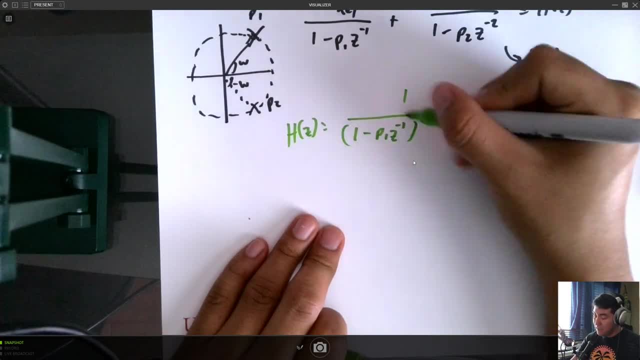 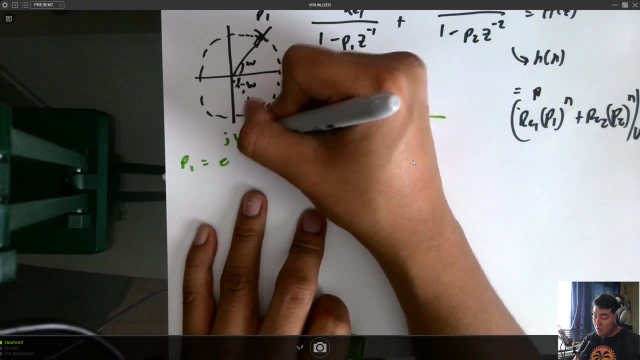 One minus P of one Z to the minus one, And I will tell you this right now. This is one. That means P of one is equal to E to the J omega, And P of two is equal to E to the minus J omega. 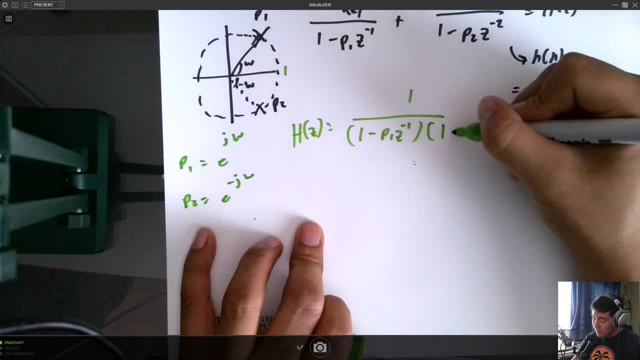 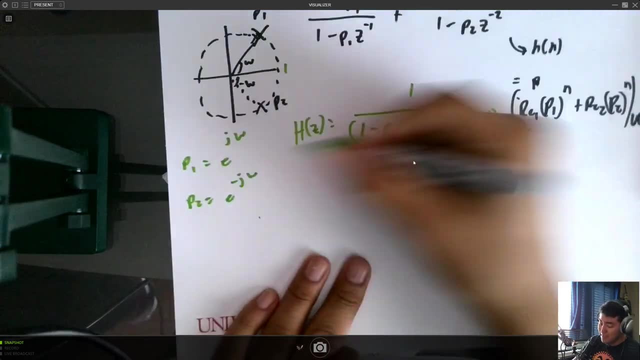 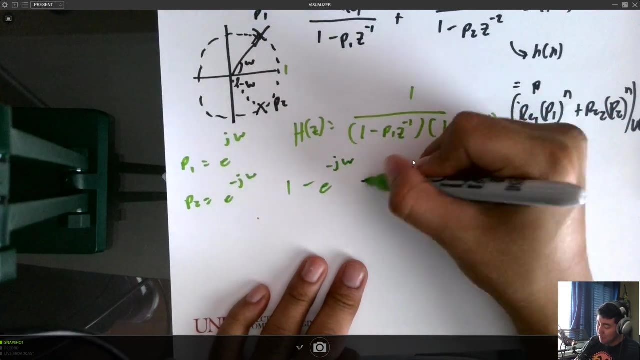 So that's the pole location. So this is one minus P, two Z to the minus one. There we go, If we want to multiply the bottom term. so let's do this: One minus E to the minus J omega, minus E to the positive J omega. 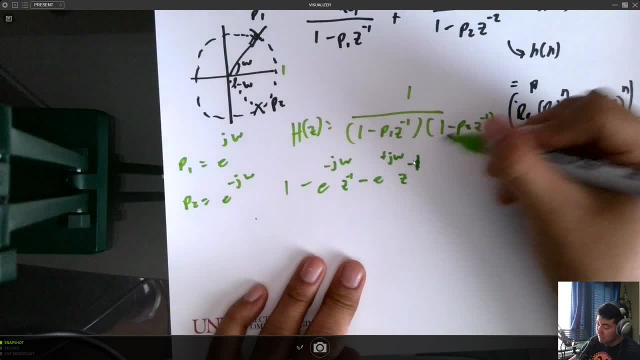 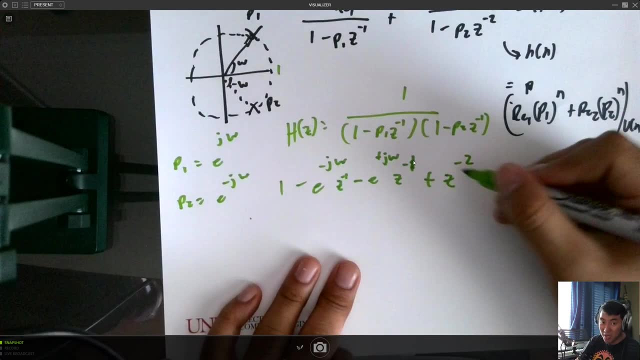 Oh, Z to the minus one, Z to the minus one, one plus. If you multiply this and this, you get one Z to the minus two. So that's that bottom denominator. But there's a rule, And you see that right here. 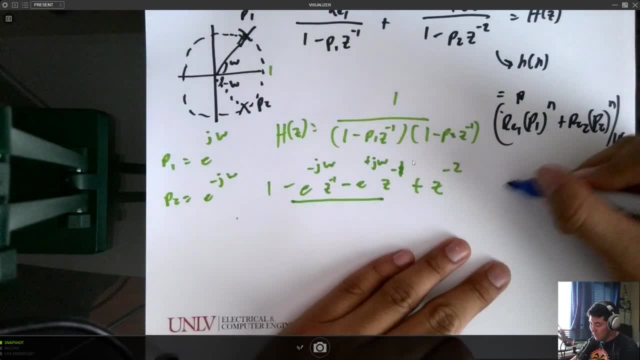 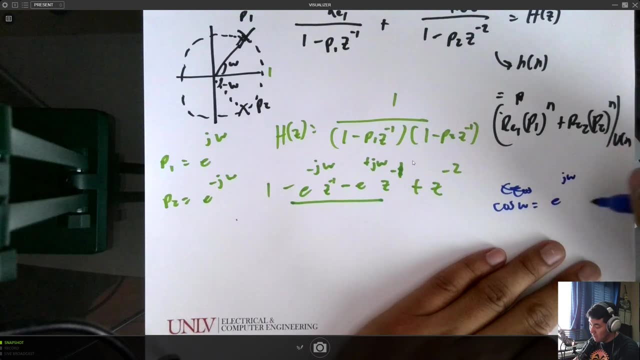 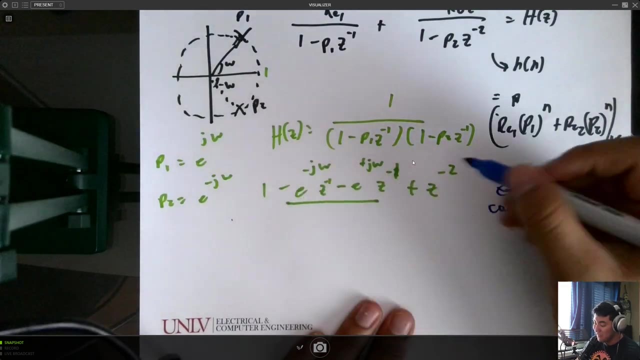 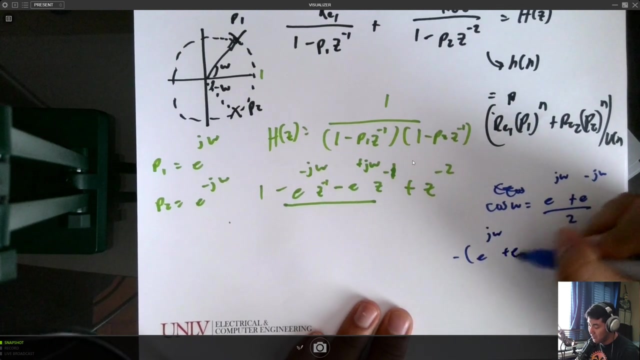 If we multiply, let's recall, cosine of cosine of omega is equal to E to the J omega plus E to the minus J omega divided by two. So if we multiplied well, E to the, let's do this: J omega plus E to the minus J omega by two. 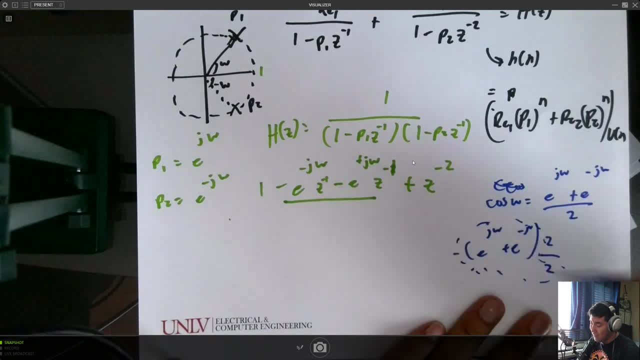 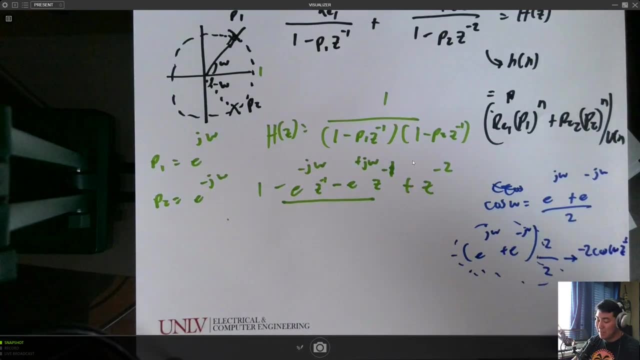 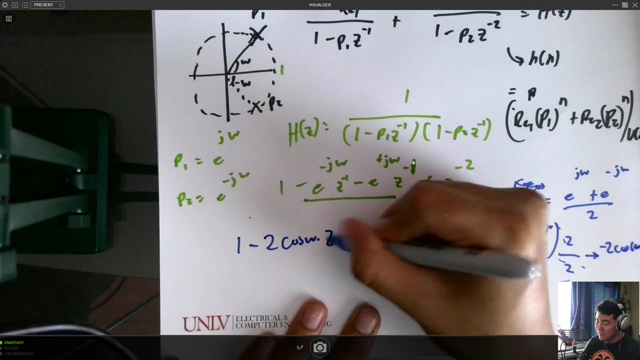 So we have this, And if we wanted to multiply this, then the resultant is minus two cosine omega Z to the minus one. So that means this whole term right here turns into one minus two cosine omega Z to the minus one, plus Z to the minus two. 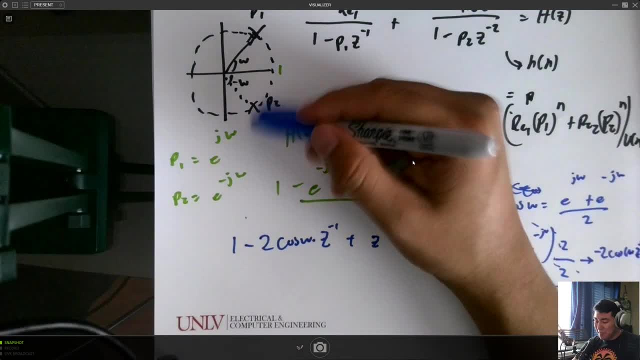 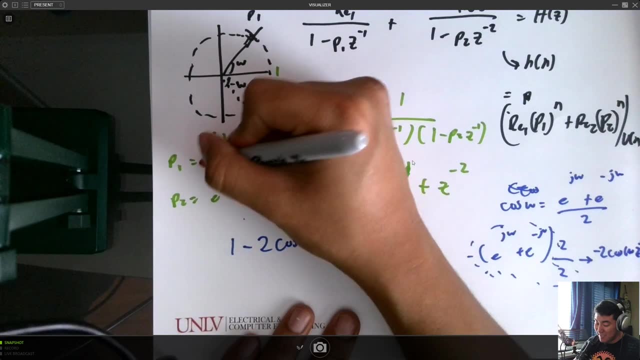 And now you're saying: OK, so we notice that the pole is at the unit circle, But what if it's not on the unit circle? So there's a term. If we put a pesky R term in here, you know R, R. 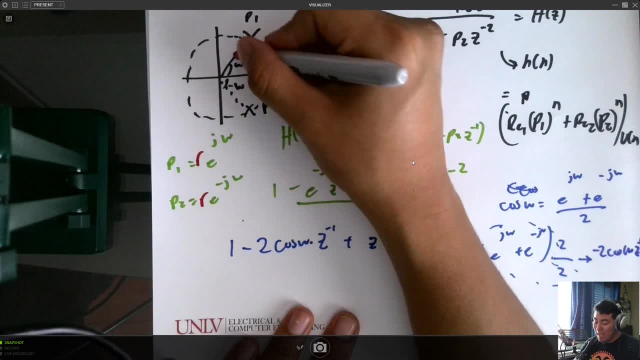 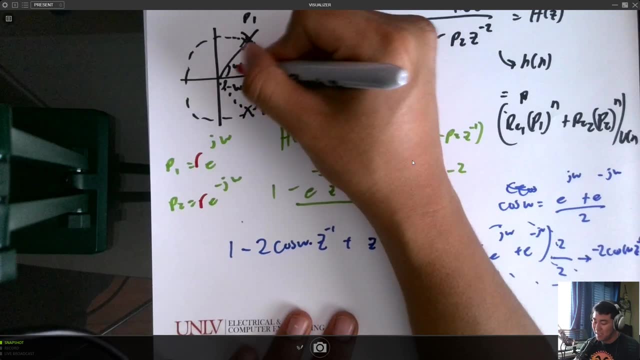 So that means, oh, if R is equal to well, half point five. that means the pole is going to be here at the distance, point five. So it's easier if you can see here: R, point five, And this E to the J, omega just spins it around the circle. 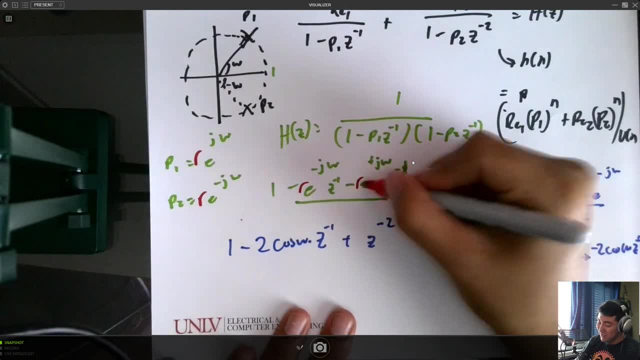 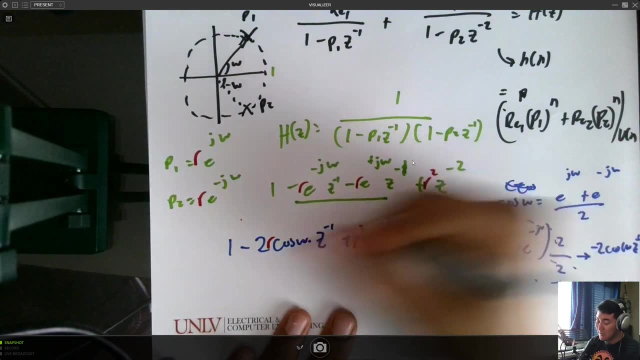 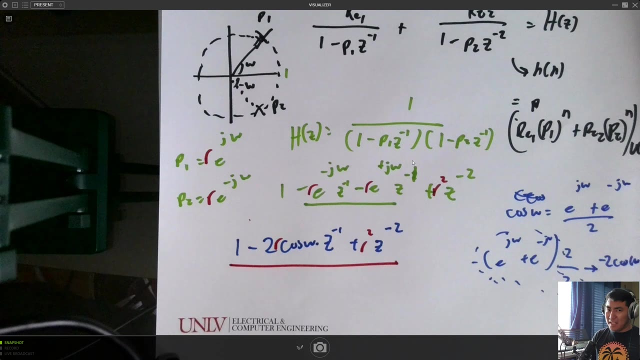 So we just put an R here, R here, R, R gets R squared. And yeah, we can just punch that R right there and R squared. So that's that little proof for how to get that nice resonating denominator. And now you're saying: well, 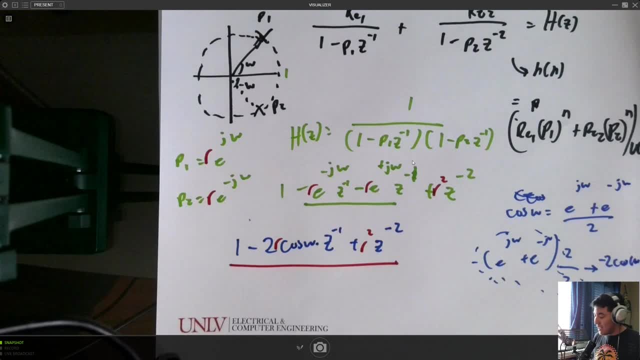 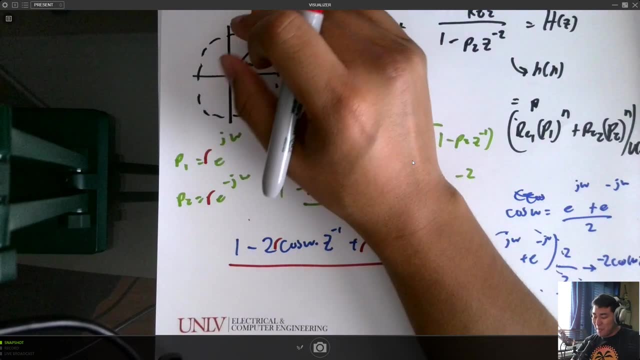 how do we do a PZ map, And you probably notice a mistake and that, well, this right here is not the real Z plane map that I want to draw, so this is not the answer. The answer is actually going to be something cool. 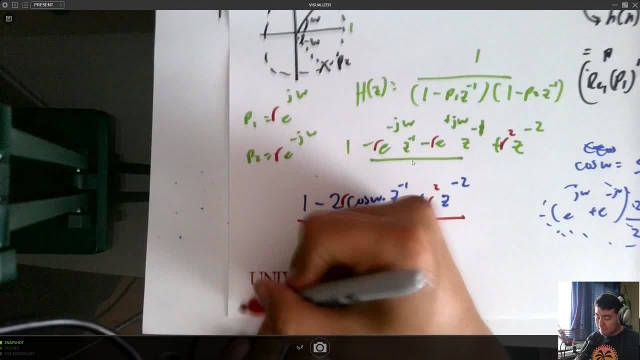 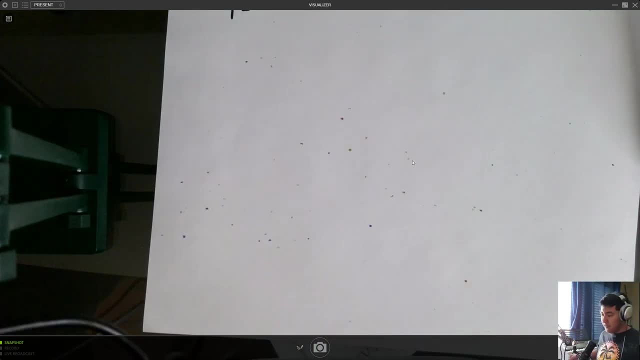 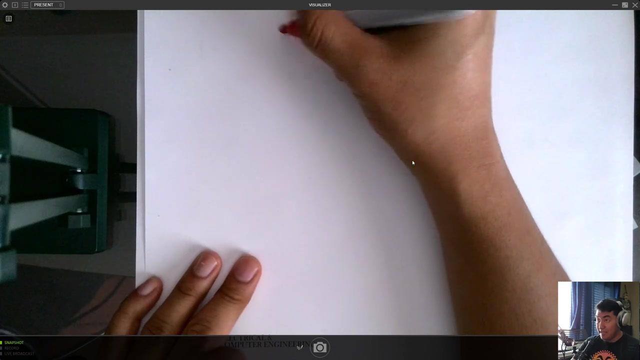 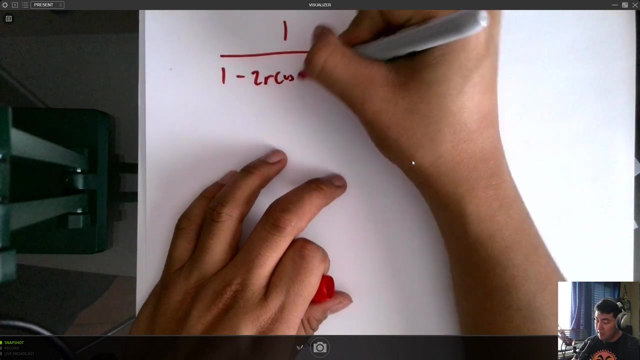 So I will show you here Five And we are at the 23 mark. So, and this is what you're going to do in your assignments and on the exam, If let's just pull this one out, One minus two R, cosine Z to the minus one plus R. 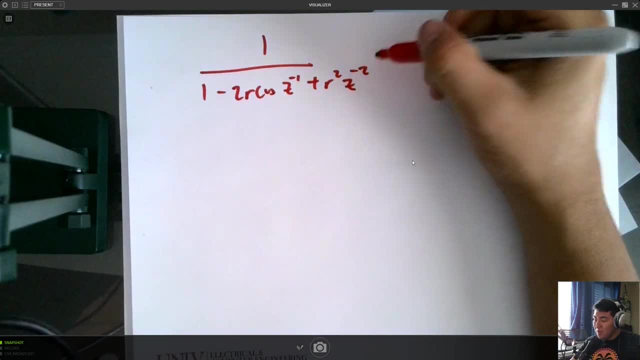 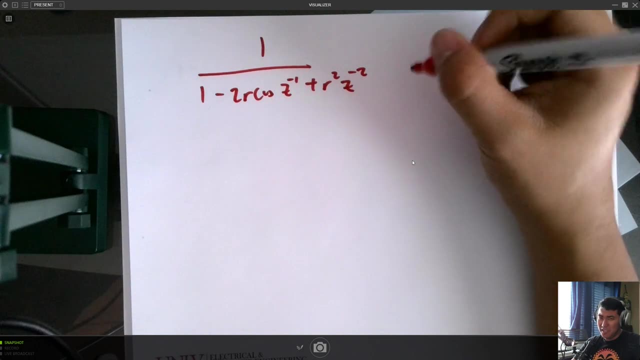 Square Z to the minus two. Where are the zeros and where the poles? And if you're going to say, oh, there's only two poles, Well you're wrong. There's actually two zeros. And you're saying, oh, where's that? 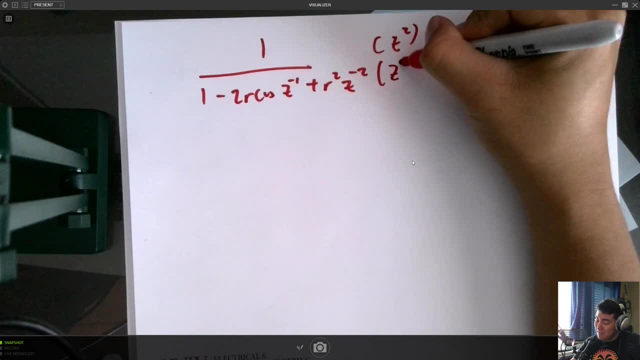 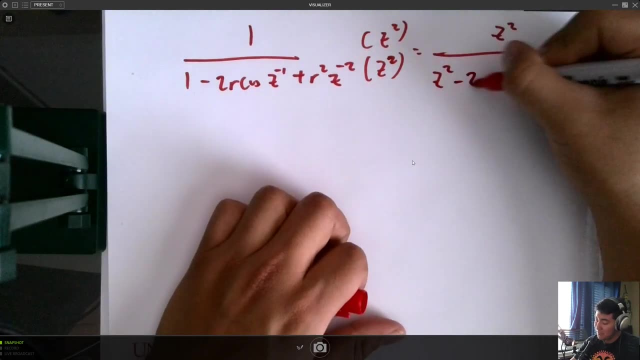 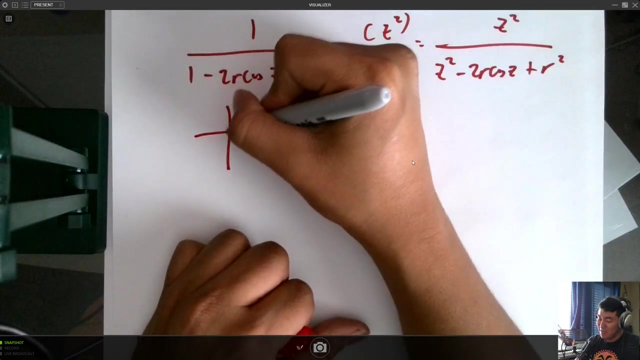 If we multiply top Z squared minus to the squared, Therefore we get Z squared, Z squared minus two R cosine, Z to the one power plus R squared, And now you can easily draw the system And that means you have two zeros here. 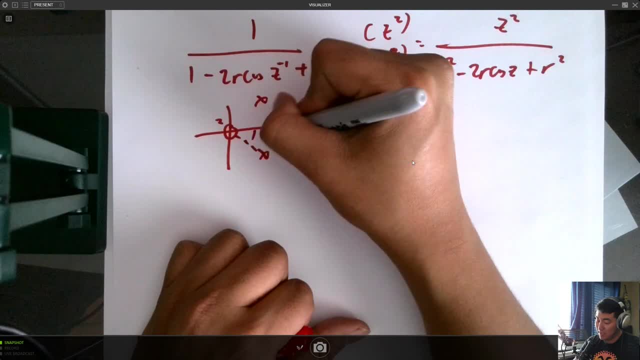 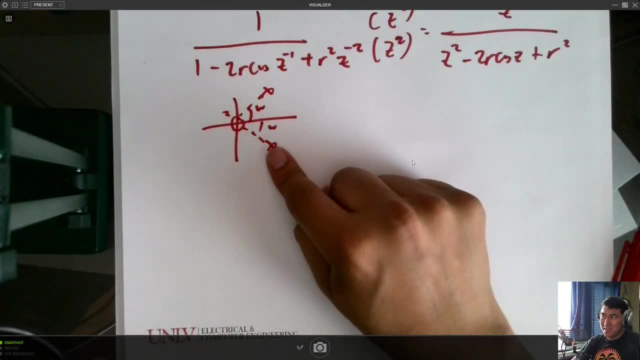 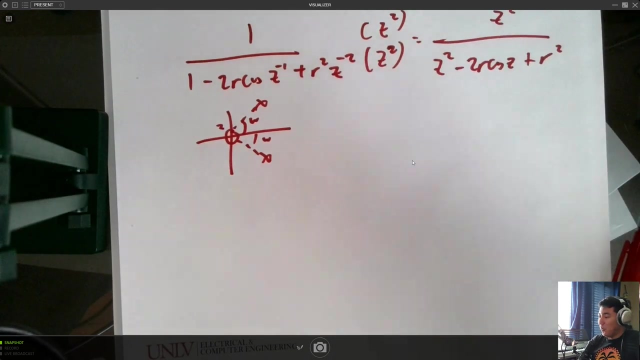 And then you have a pole here and a pole here, depending on your omega term. Really easy, right. So this is how you would draw your system. so if you go to an interview and they tell you: OK, draw me the the poles and the zeros of a resonator, and you just give them the poles, 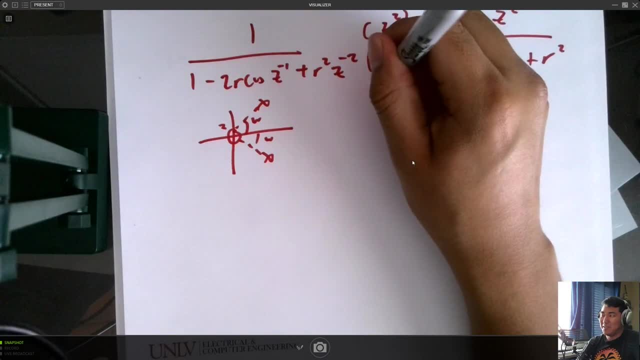 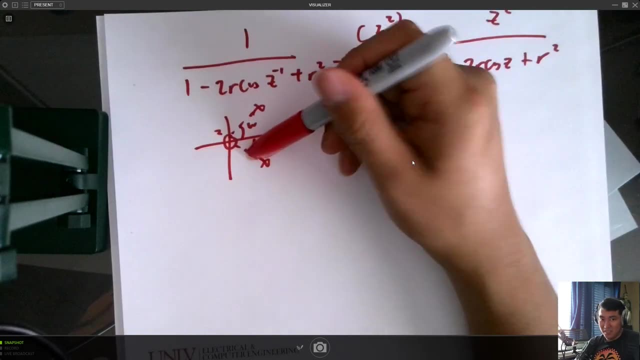 they will just turn you down right on the spot, because this is a really practical, really trivial stuff. So on the assignment I will be taken off a point if you don't put the zero. So I'm just warning you. But no, it's because this is a practical thing. 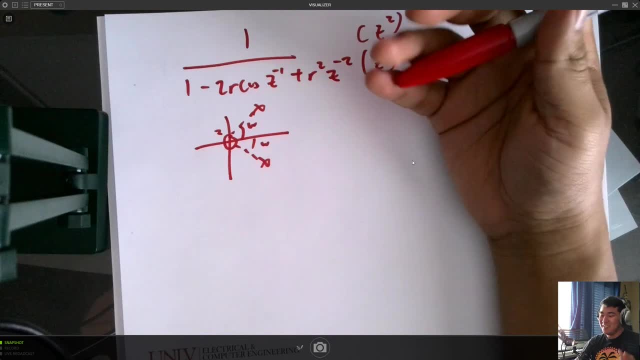 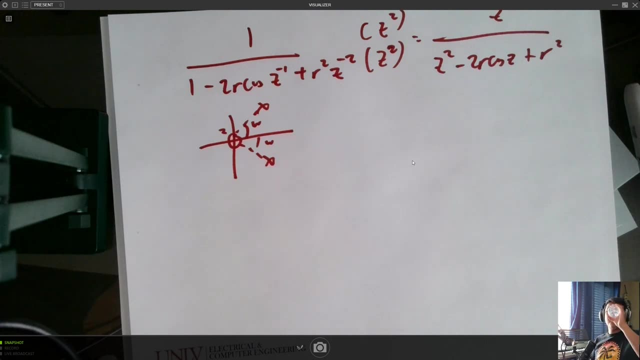 There's people in 722 who are like mixed signal design, who just don't really see the zeros. I'm like there's a zero on the thing. It doesn't affect your magnitude but it affects your face, So don't get it wrong. on the interviews: 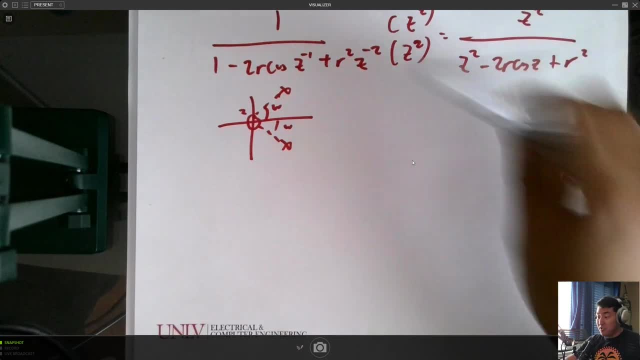 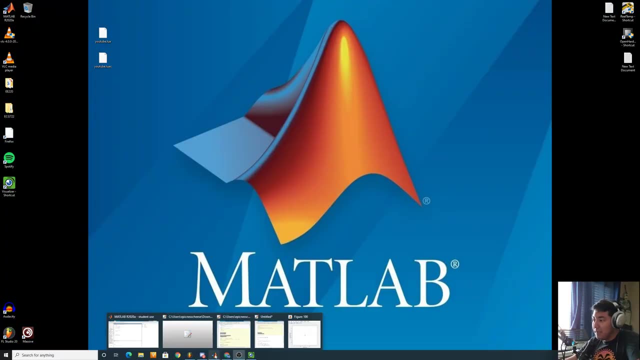 So now we're saying, OK, now what do we do? I want to show you an example On Matlab. So we go to Matlab and I already have some stuff done. I think this right here. Nope, it's right here. 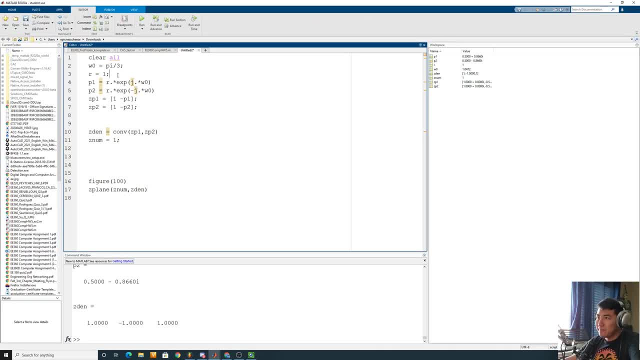 I've already whipped up some cool stuff to show you, so we're going to clear all stuff. We're going to have an omega knot of pi over three. This is what I chose, So we're going to expect to see the poles at an angle at pi over three. 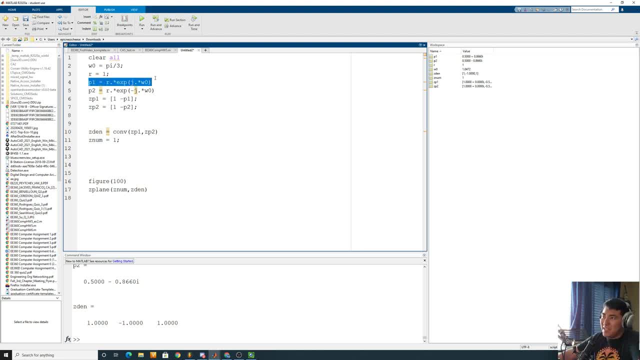 Radius of one pole locations here at positive j omega, The other ones at minus j omega. And then to get the Z terms, the pole locations got to do one minus p one. Don't forget this minus term, because that's the rule of Laplace. the Z transform 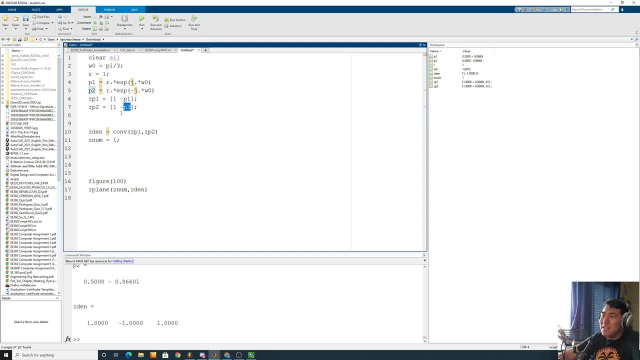 Sorry. And then the same thing with this guy To get the denominator. we just convolve them And then note we're just doing a really simple resonator, So we're just going to put a term of one there. So we wanted to draw the Z plane. 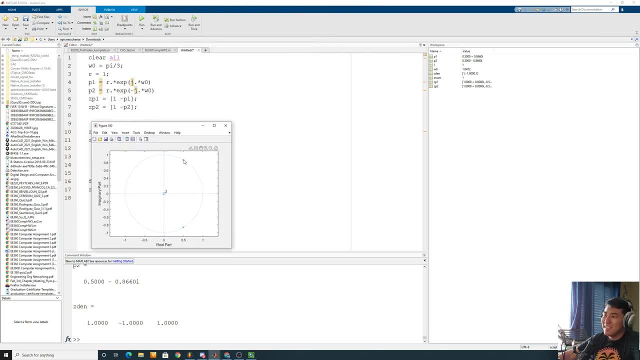 So let's look at that Boom. does that look right? Look at that, That thing right there is at pi over three, And if you don't believe me, let's just do pi over four. You understand what's going on. 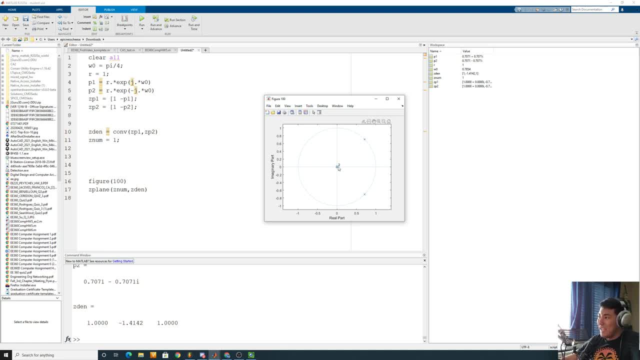 See, as if you create an angle from here to here, you see that pi over four or pi over two, wherever you want, that's how it works. And then you're saying: OK, David, now tell me what that R value does. 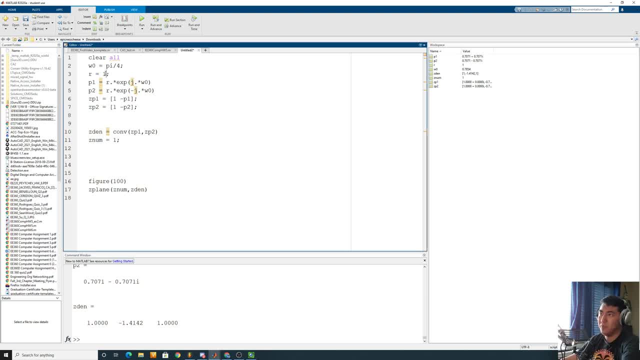 And that's the reason why I edited your assignment, so that you understand what's going on. hopefully clicks on your brains and you're like: oh, now I can do systems. So let's just change it to point five, because it's the easiest one to see. 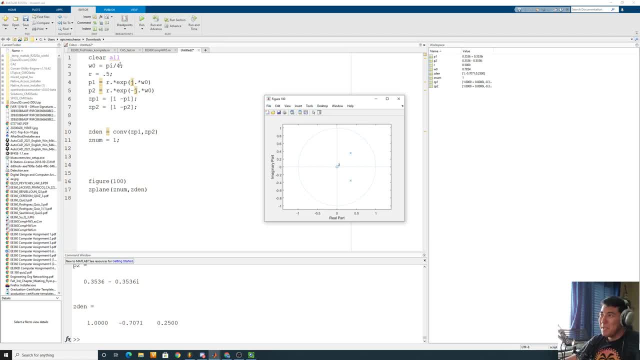 And you're like, oh, but you're like I can't see if it's Point five, man, All right, Then let's just choose a really small angle in the small angle Which is like one hundred, And you're like, ah, there it is, you see. so that's why we do these systems. 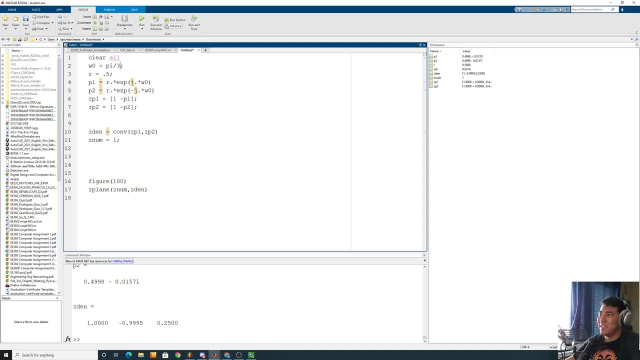 Is it making sense? everyone, Hopefully it is. And now you're saying, well, what do we do now? What's the magnitude response, or what do we get from these systems? So I'm going to try to show you guys what's going on. 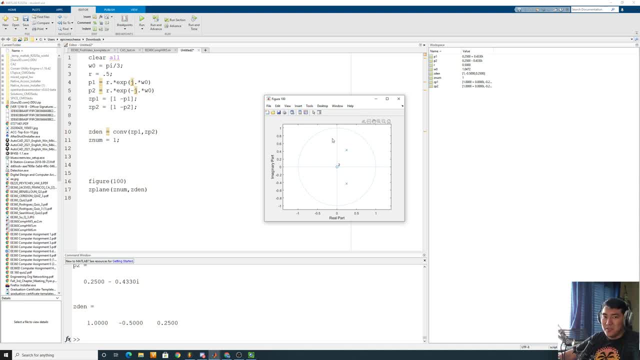 So we're going to try and figure out the magnitude response. So, for engineers, we like to look at the actual unit, the unit circle, and this is actually leading to the Fourier transform of the system. This is what we want. It's a spectrum. 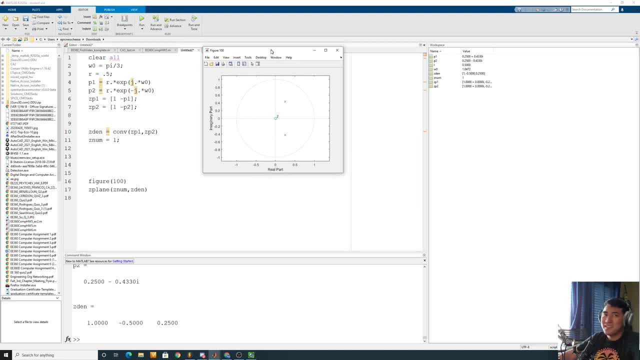 It's the Bode plots, It's what you always see in your circuits classes. So we want to analyze the system at every point and just look at the value. So I whipped up a little thing right here and let's pull it up right here. 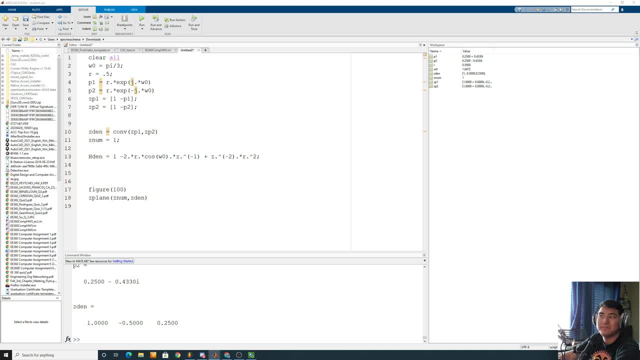 H then, and there we go, And HZ, And there we go. So this right here is one divided by well, whatever resonating terms I had there, There's radius Z to the minus one. You can also do Z squared. 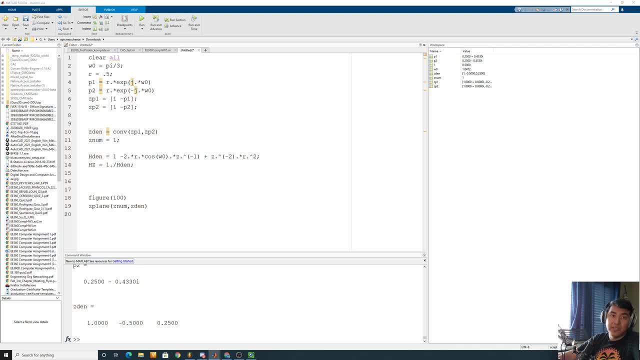 You can do that, but, however, I'm going to show you the governing equation. This right. Here's your governing equation that you need to know. As long as you do this, then you're fine. I saw someone like: oh, they put the real. 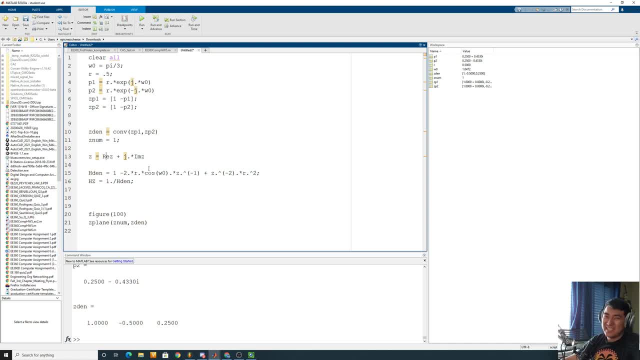 part, like alpha and betas in their things and like they separated the imaginaries and the real part. you can do that, but that's a lot of work. Don't do that. MATLAB does a lot of stuff for you, So you can literally leave your terms like this and MATLAB will take care of that. 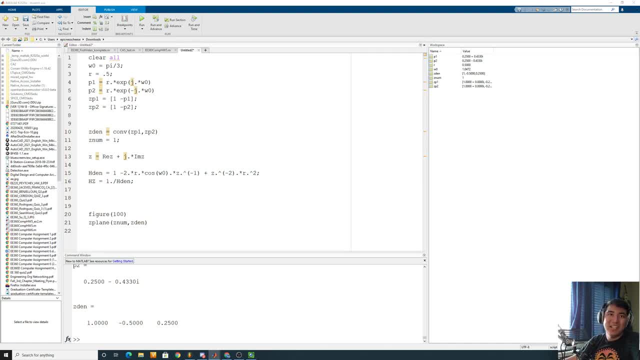 for you. So, Just like what we did on the previous small stuff, previous stuff that we've done if we wanted to map this on a unit circle. so we're going to just look at minus two to two. minus two to two- mesh grid. 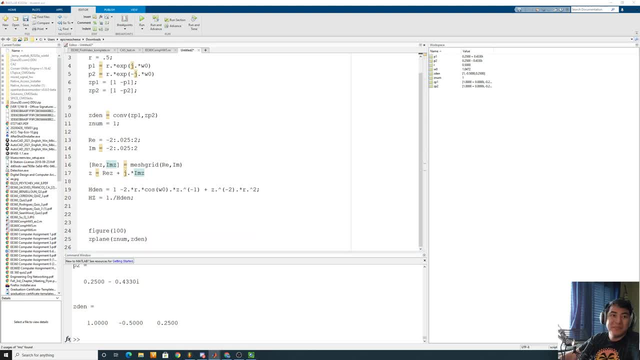 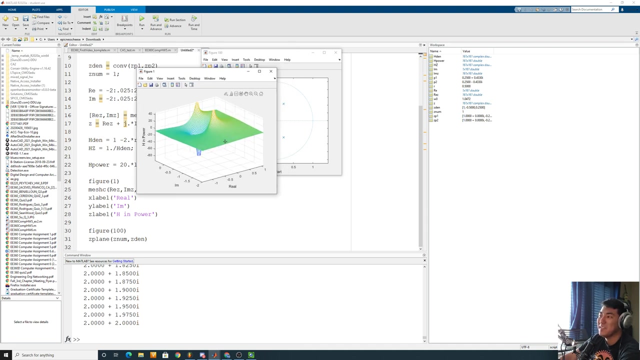 It's the same stuff And we're going to analyze this system and let's look at this right here. Here we go. So we're just going to look at what the system does, Boom, And you're like whoa David, and you can clearly see that we have two. 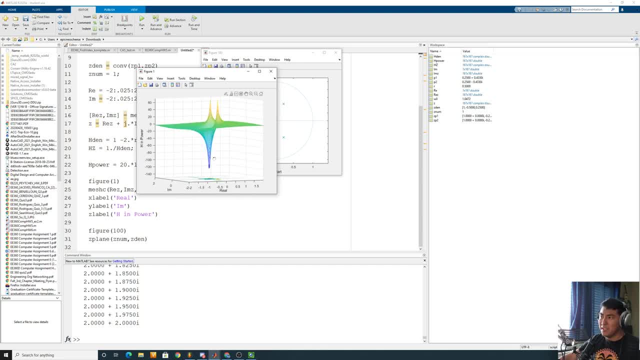 poles, poles and a zero that dominates, a huge zero, because there's two zeros there And you're like, ah, that's making sense. but you're like I can't see that, David, and I'm going to say, yeah, I don't blame you. 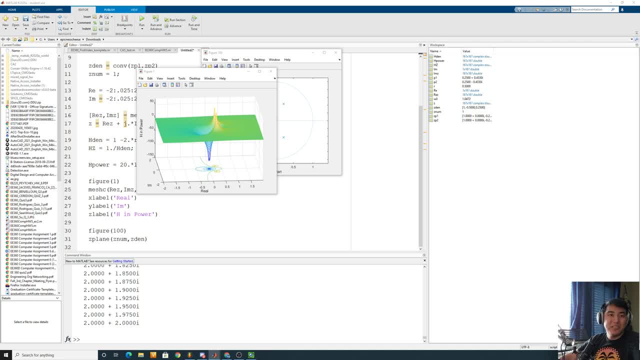 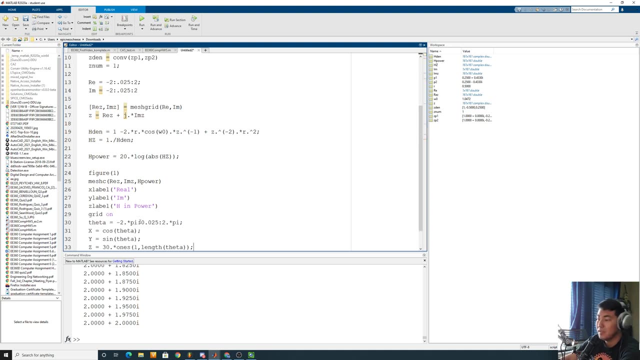 So what I did? I whipped up something pretty cool. You can do this if you want, but you don't have to recommend not to do this. No, that doesn't actually do anything. Should have plotted that other point. Let's just plot this guy right here. 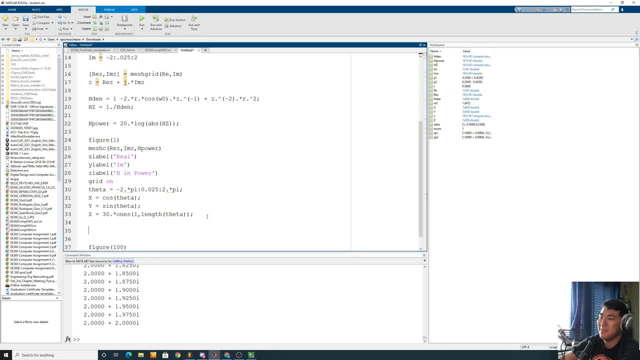 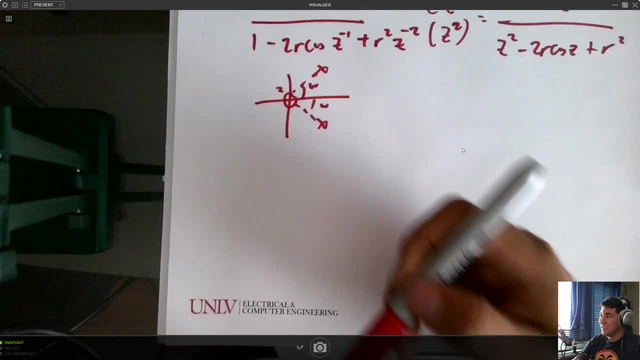 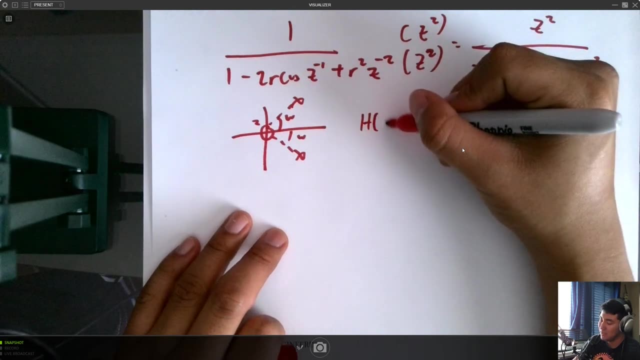 I'll show you something cooler. So the other thing I wanted to show you is: OK, what if we wanted to do a magnitude response of this system? So we wanted to look at H of, I think, J, omega. So we're looking at when the real part of Z is equal to zero. 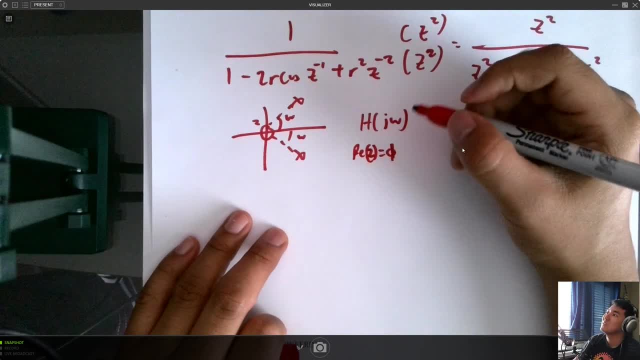 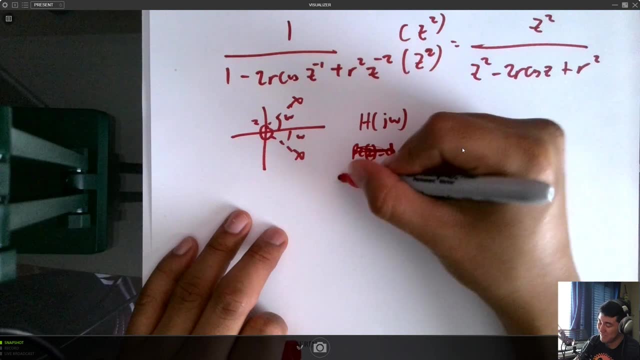 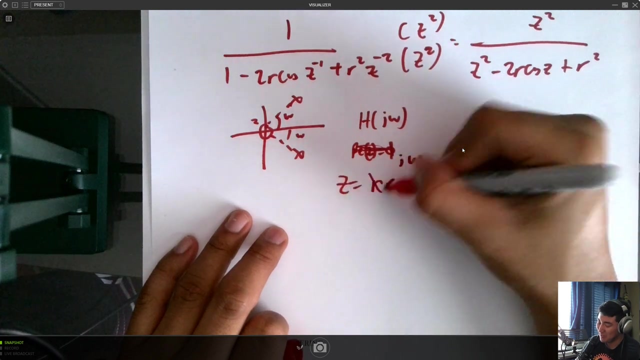 It's going to be on the unit circle, It's just going to equal all one. No, no, no, Sorry. If Z is equal to RE, to the J, something omega, then we're just going to look at when R is equal to one. 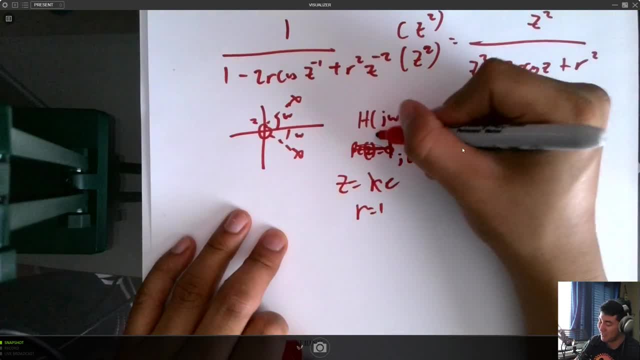 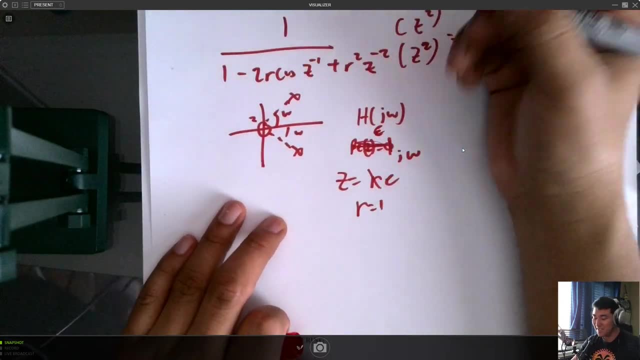 So we're just going to look just at that unit circle. So J omega. E to the J omega. There you go, That's what I forgot. E to the J omega. Let me replace all these Z to the minus ones with J omegas. 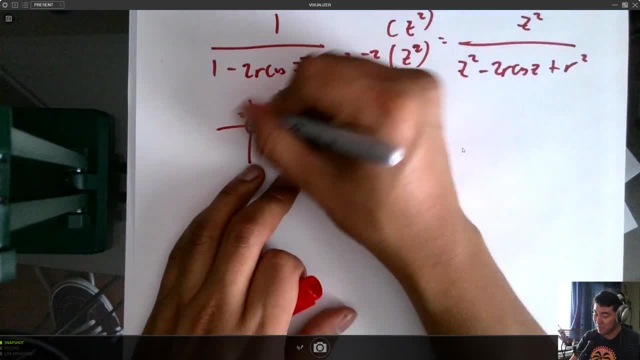 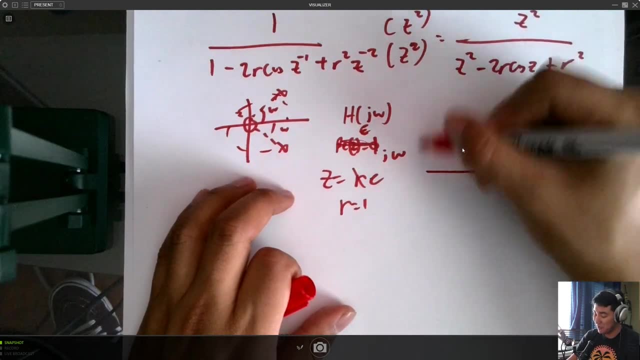 And now we're just literally looking at the unit circle and we're plotting that And you're saying, OK, how do we do that? So one thing I'm going to show you is if we were to look at, well you know, 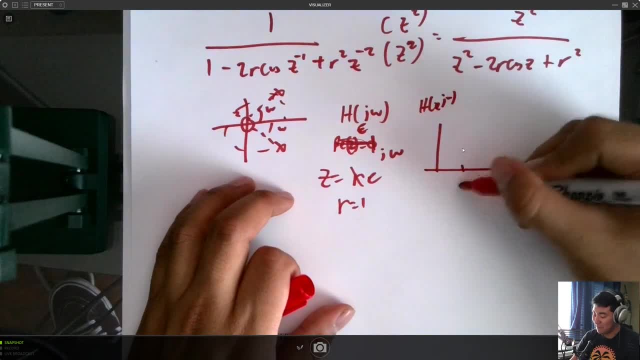 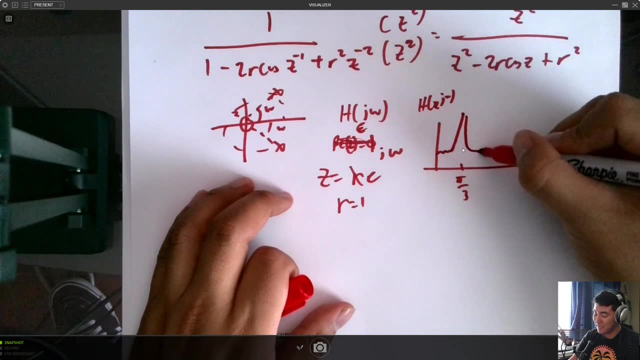 the H, E to the J, omega at pi over three. if we were to look at this like: oh yeah, we're going to have some signal, Oh gosh, you're probably going to see something like this, And then consequently, on the other side, minus pi over three. 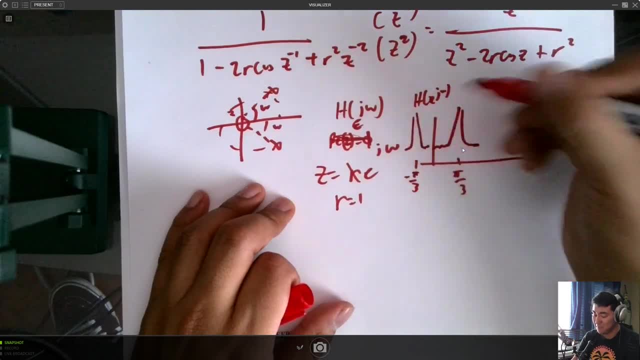 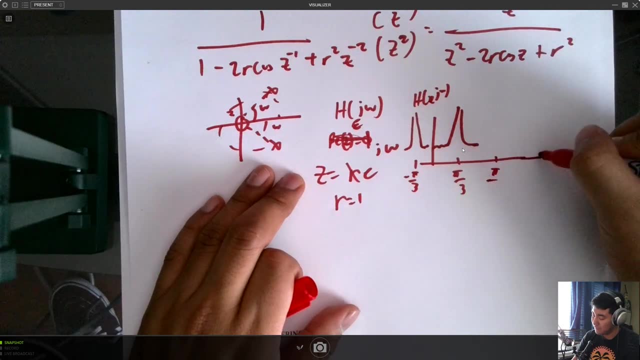 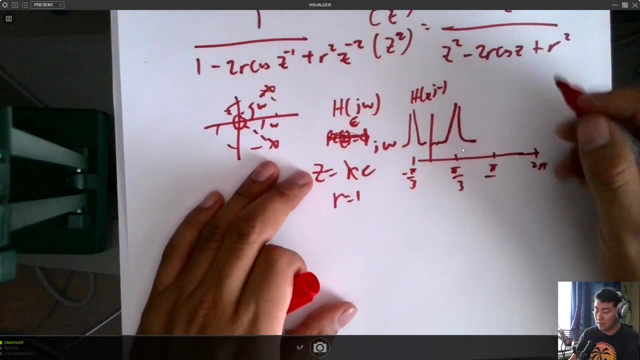 you're going to be like oh, and then, oh, you're going to probably see something like that. And then there's another rule I want to tell you to pi, And this is an advanced like DSP classes of 480.. Let's tell you, tell you about this, is that? 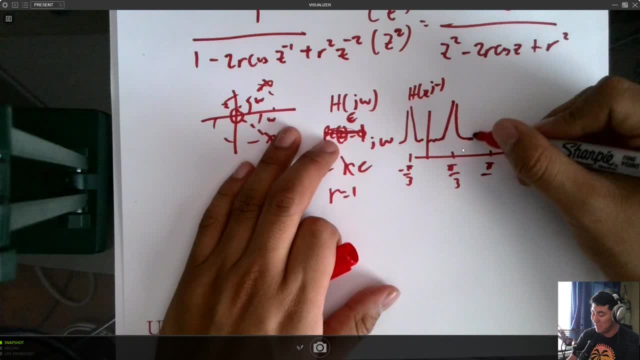 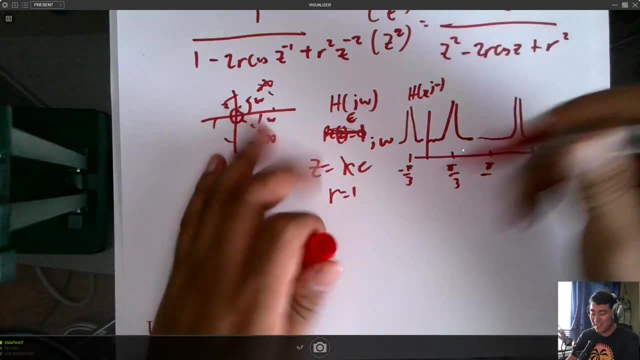 the spectrum repeats for discrete systems. So we were to go into here. we'll probably see another peak like oh, yep, Oh and boom. So you'll probably see this in your diagram. So what I want to show you is the following: 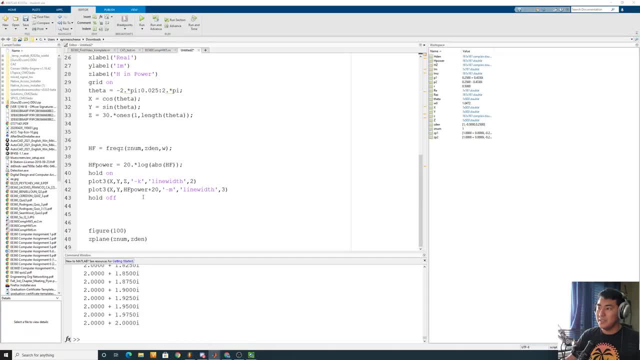 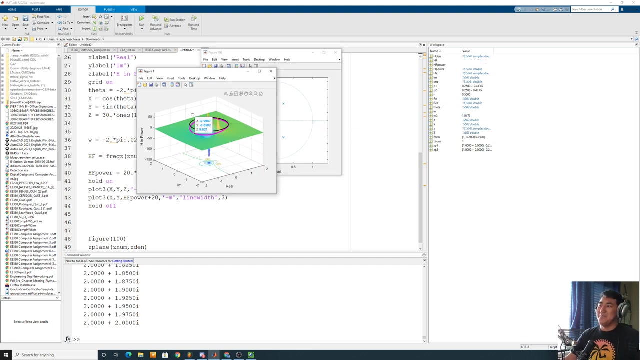 If we were to go to here. so we're using the Freqs Z Run that untitled. Oh, that's because I forgot W Boom. Oh, that's where it came from. So what I wanted to show you was: I drew this black circle right there. 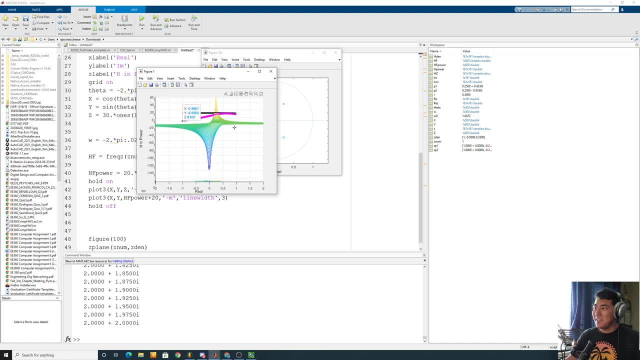 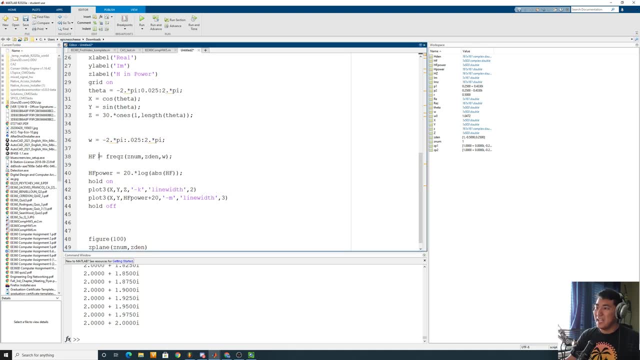 to show you that that's a unit circle. But you see that magenta thing right there. Well, that's supposed to represent the magnitude response itself. So actually I actually put a DC gain in there. Let me see if I can take that off. 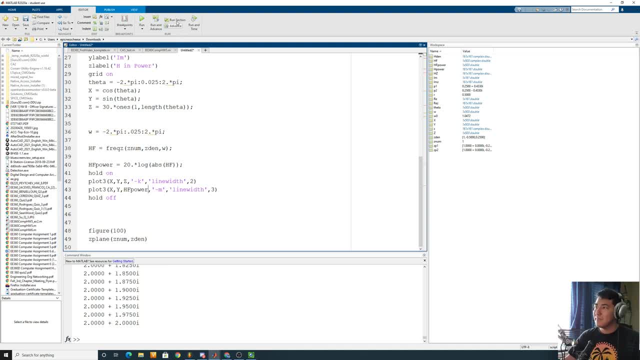 Oh, there, it is DC gain. You see that pink line. That's exactly what you'll see, And I will show you another plot too, Figure 101.. H- No, no, no Plot. H F. 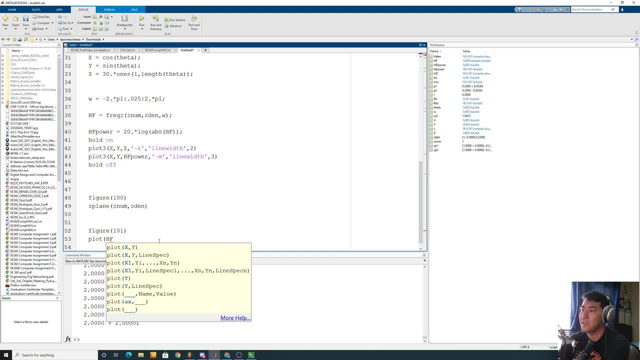 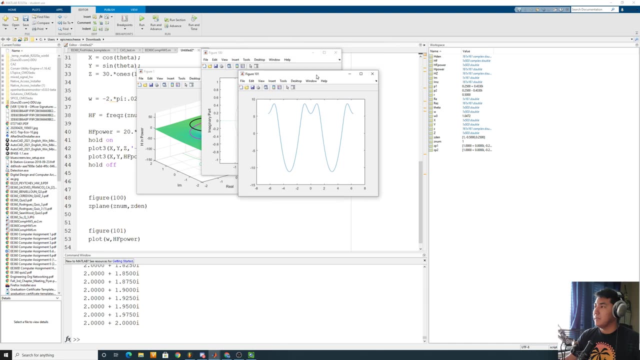 No, no, no. Freqs: H F Power Plot: H F Power. There you go, Omega. There you go, There you go. So that's what our system is actually looking like for this guy right here. 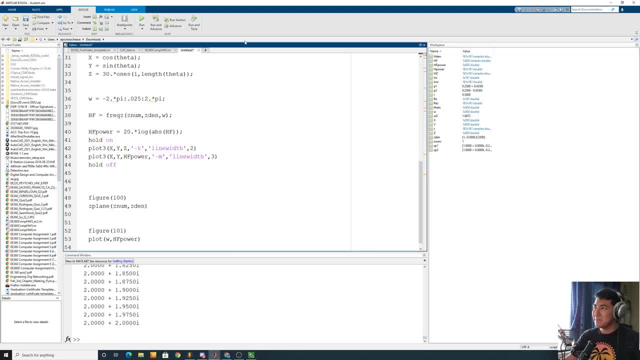 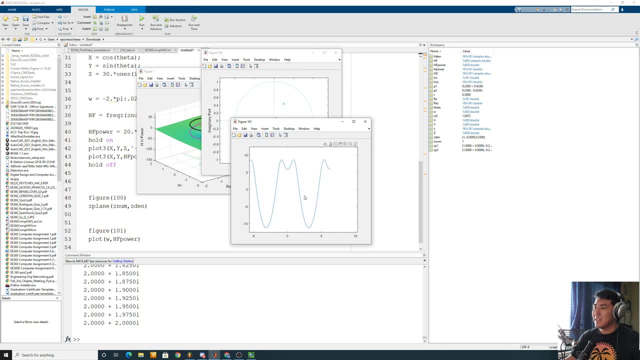 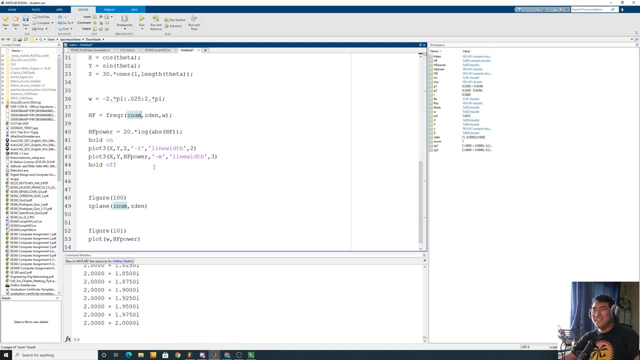 Actually that looks right. Hold up, Okay. Okay, Looks right, I think. H F Power Log of this Yep Not that bad, Okay. But the point is now you understand what's going on with these systems. 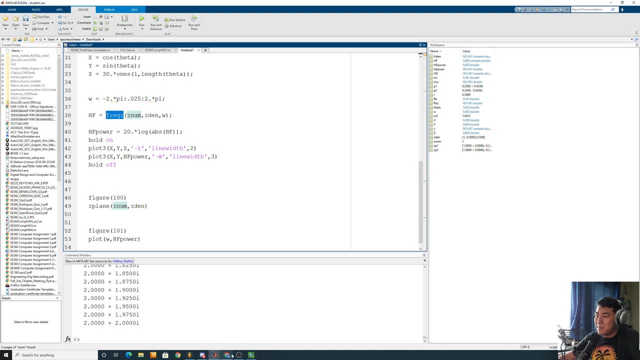 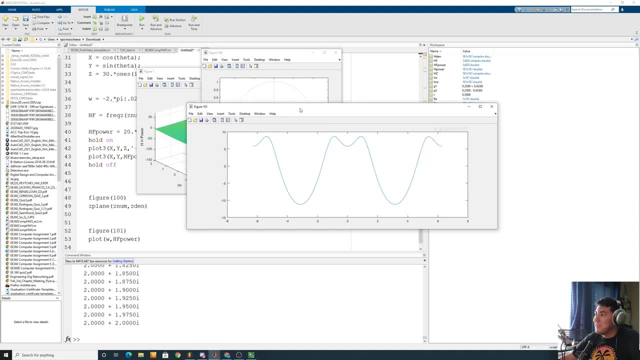 It's basically well if we were to look at the frequency response. the frequency response should look like: well, if we were to squish this, if I wanted to, if I grab this guy right here, you can see that. 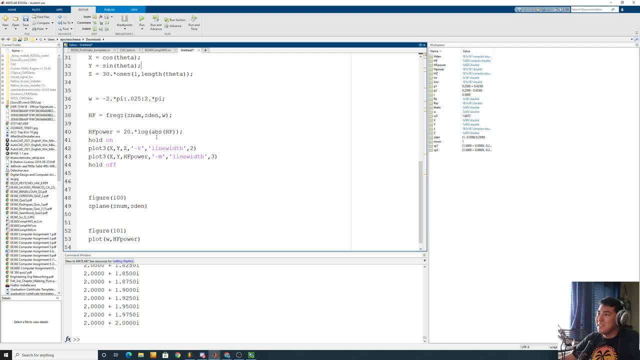 Why does it not look like that? It's okay, Let's clear all. Let's do pi over 4.. I have a great idea. What if we just make our system actually unstable? 0.9.. There you go, Oh, there you go. 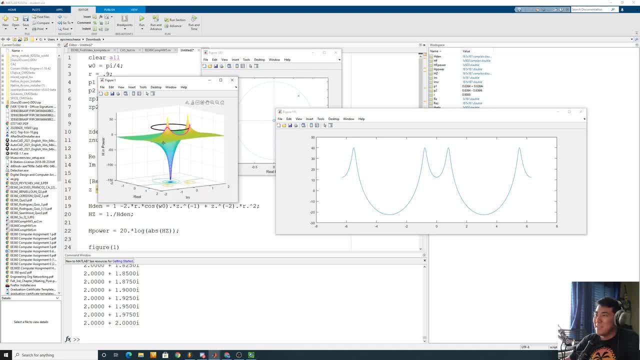 Now you have distinct peaks. There you go Actually. yeah, you can see that better, See how, Oh, you got these little peaks Right there. That's exactly what we're going to see. So here's actually at the frequency where the frequency is both zero or DC. 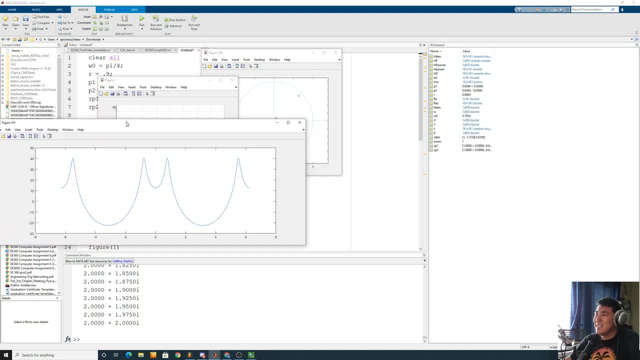 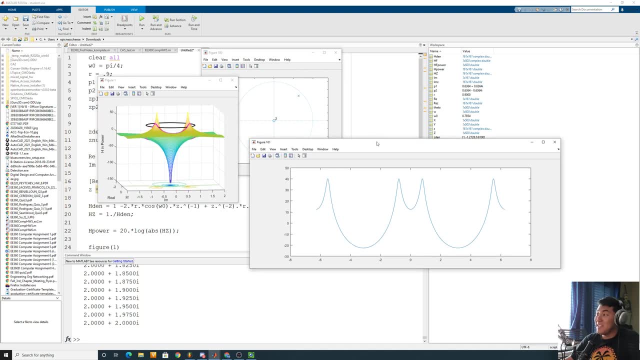 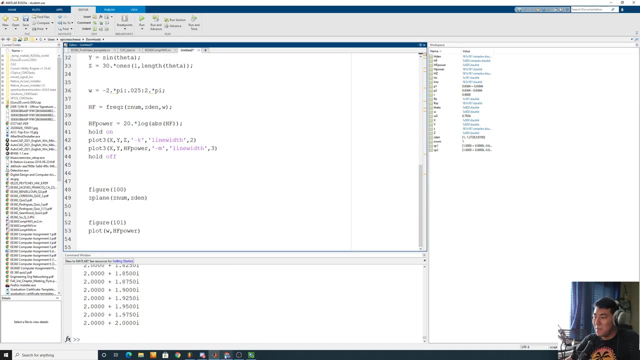 You can see these peaks. Ah, I see Kind of looks like the Batman symbol. So that's what I wanted to show you. So this looks like this and you're doing it right. So what else do we got to go over. 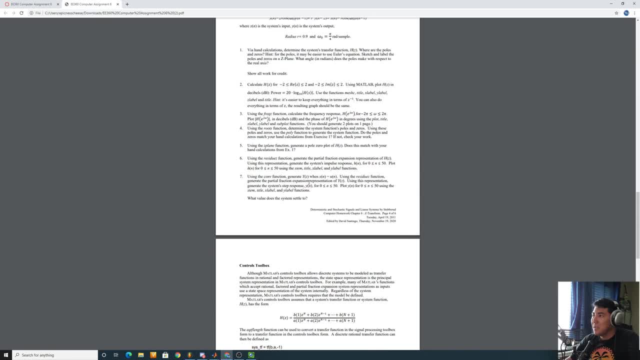 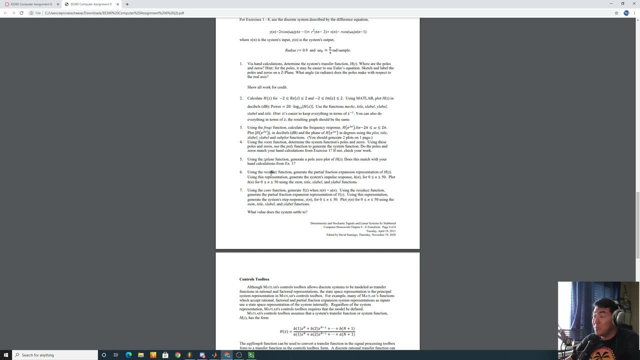 Yeah, Yeah. All this is basically the same. Can you understand these systems? Z plane: you know exactly what's going on. The residues: you know how to get that using the residue theorem. I've already showed you by hand calcs. 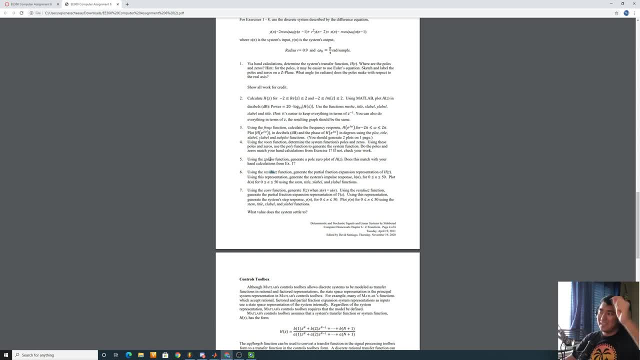 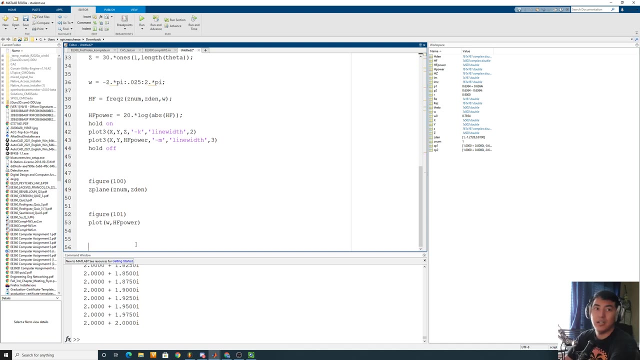 And because it's a resonator, you will see it resonate. So basically the same thing. So you already know the residue times, the pole location to the nth power. You have to use the residue theorem. So actually, let's just show you the residue of this guy. 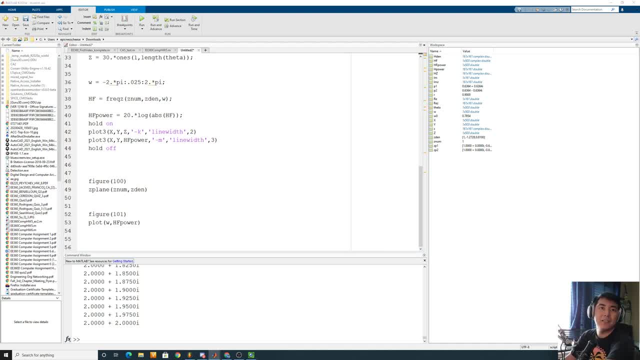 I will show you that right here. Yeah, I'll just show you right here. R P K- Actually, let's not do that. R Z P, Z K Z. residues of Z, Z, num Z. then There we go, We see that. 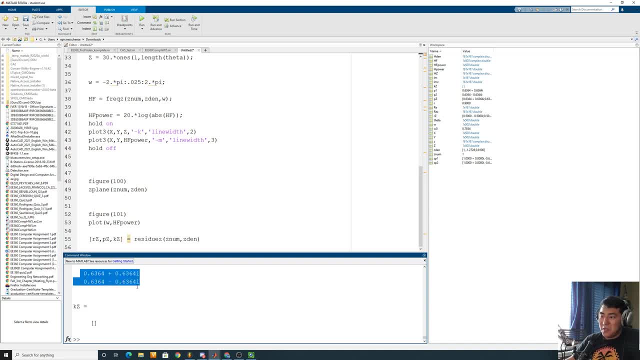 Well, we get this term right here and this term right here. So if we were to put that into: well, our numbers, Well, we plot this number and we plot this number, Here's our residue, And then we put this to the power of that. 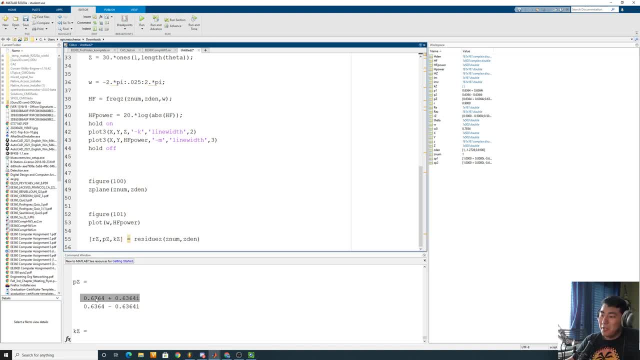 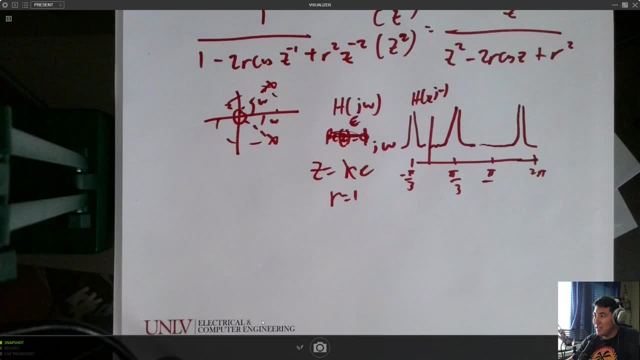 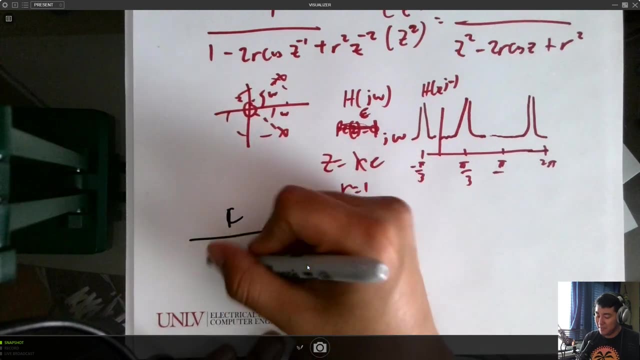 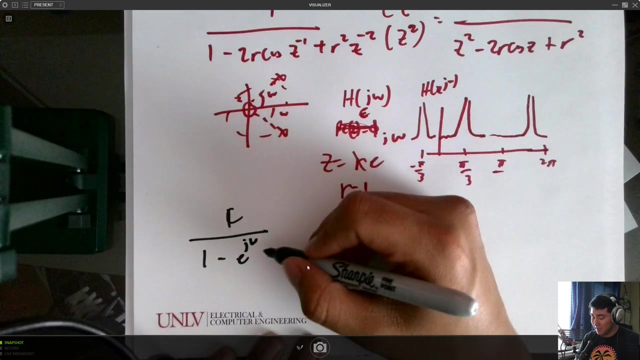 Then we should get that. But I'll tell you right now the pole locations. I'll show you on a piece of paper. If you get this situation, if you get, I don't know, Some constant C divided by one minus E to the J Omega. 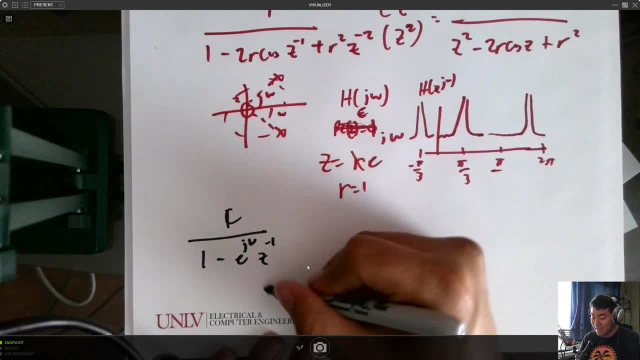 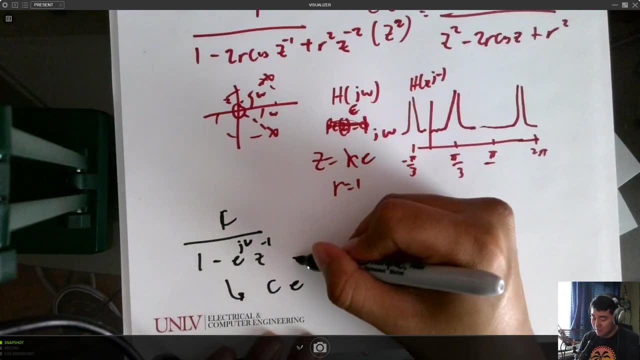 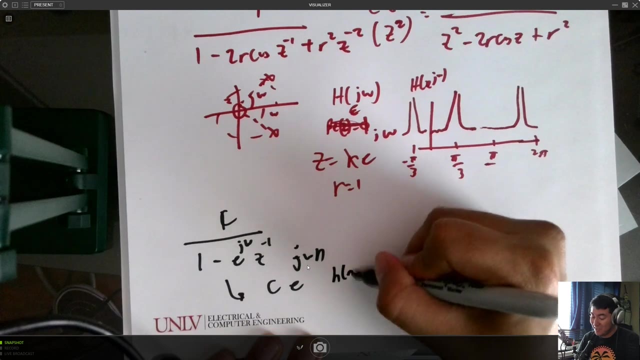 Yeah, I think we can do that Z to the minus one, Then your residue of that is going to be well, whatever value C you get there. E to the well sorry, J, Omega, And there you go, And that's in the H domain, the end domain. 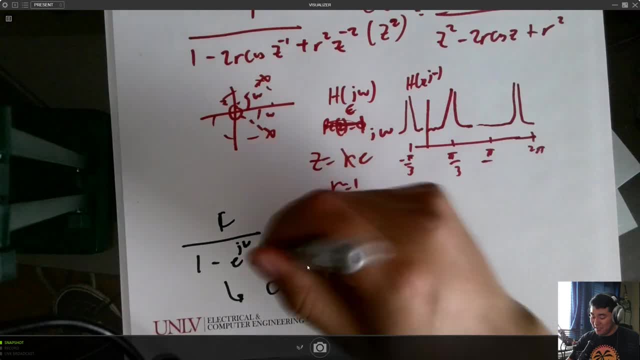 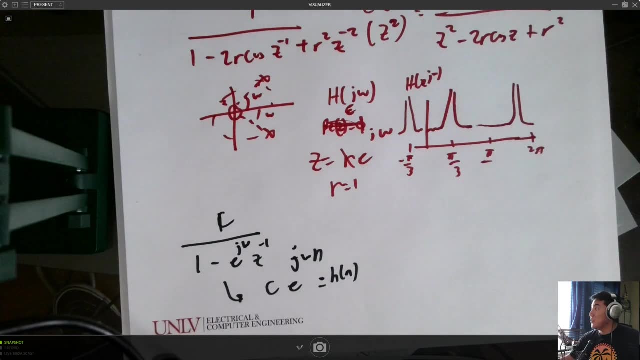 So that's basically how you would solve for that one. You will have another term that pops up, You'll have the complex conjugate And that actually heads up the imaginary values to hopefully help you solve that system. So that's how you would do that. 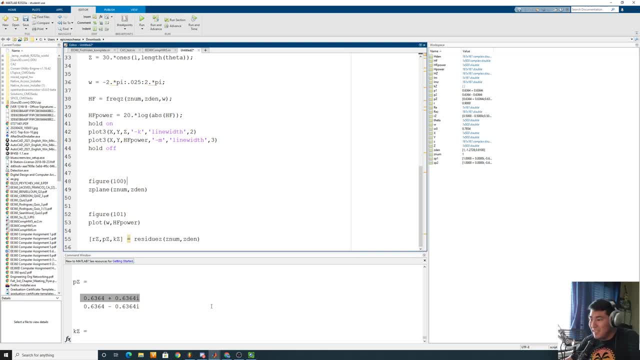 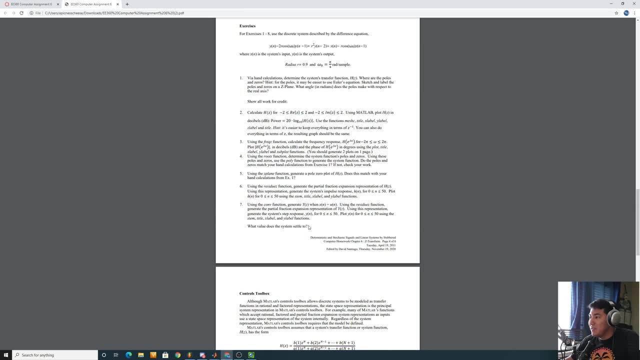 Yeah, I'm just showing you a couple of things. There we go. And then the same thing with the step function. So generate Y of Z When X of N is equal to U of N. So you already know what the unit step is. 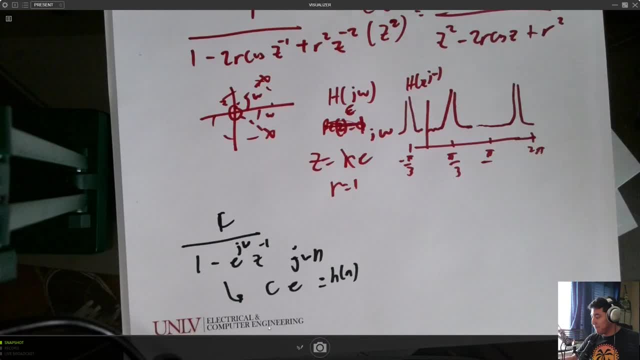 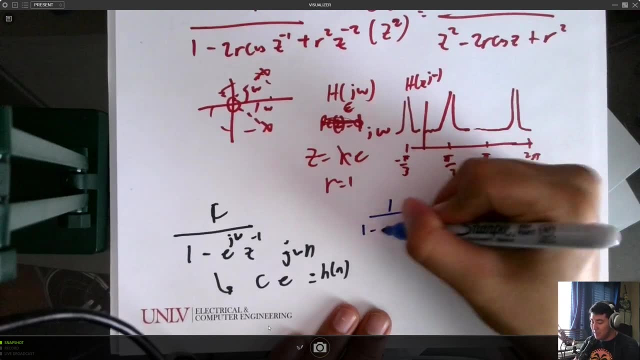 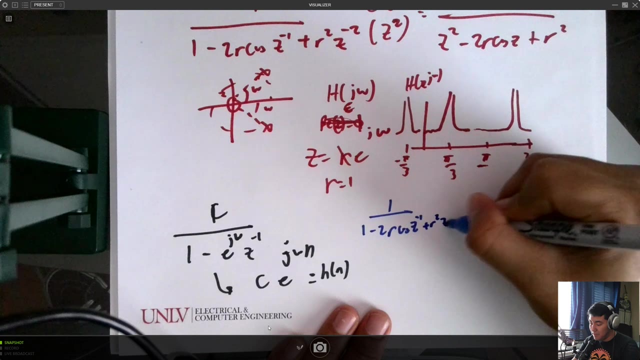 I'll show you that right here. I'll show you on a piece of paper. If you took your system, one of one minus two, R cosine minus one plus R, squared Z to the minus two, And you multiply this by well one. 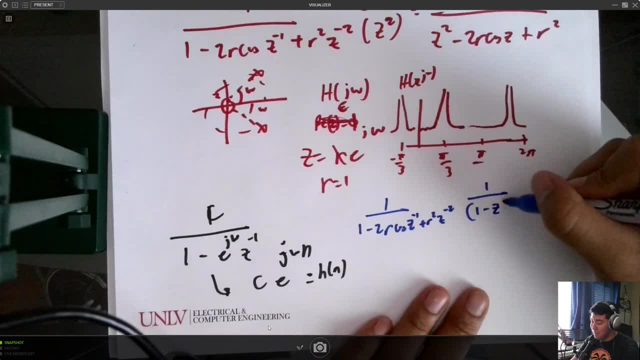 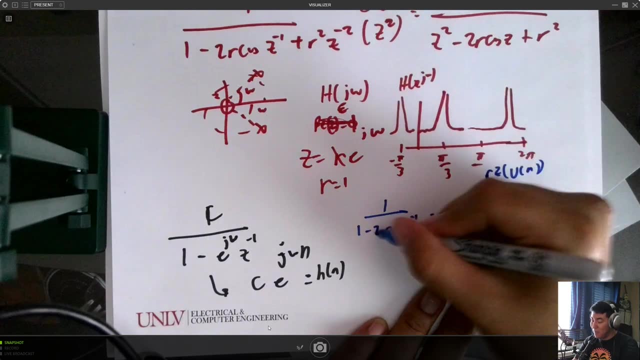 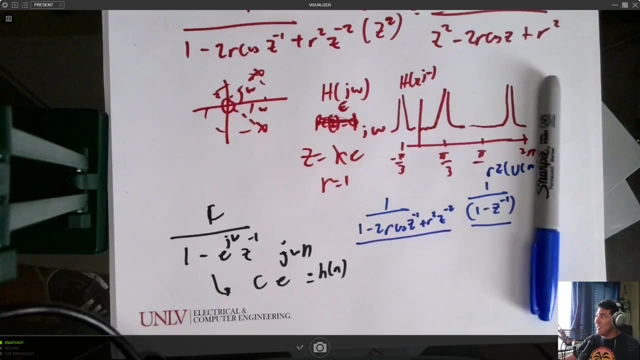 One minus U to the minus one, Because this is right, here is the unit step, unit step in the Z domain. If you convolve this with this and you get your new denominator, and then you can do the same thing, the same process. 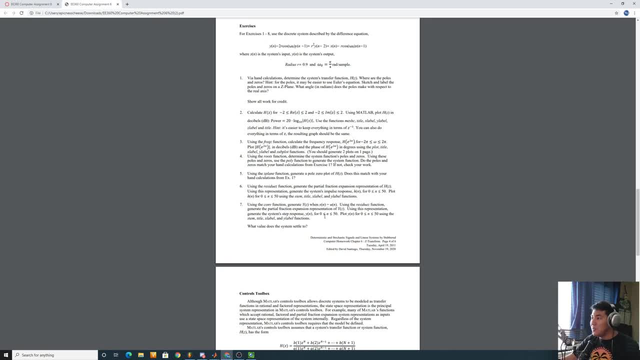 You know, let's go back to the assignment. Use the residue stuff using the residue function. Now you can get your points And then you should notice it should settle to a value. You should see a value, a gain value. So hopefully that can help you around. 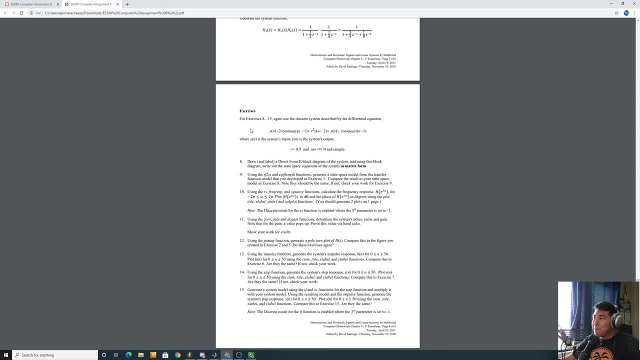 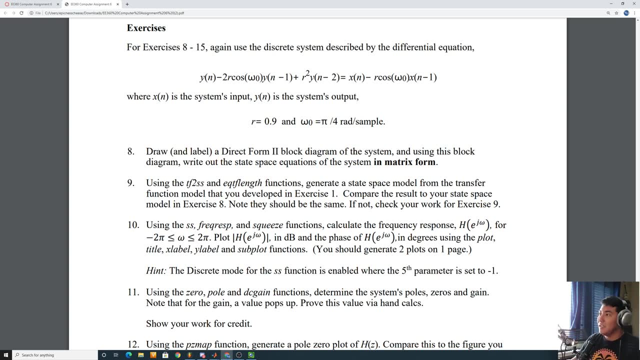 So the next thing I want to show you is this part: right here I'm just breezing through all this stuff to hopefully make sure you guys understand what's going on. So draw and label a direct form to block. So let's do this. 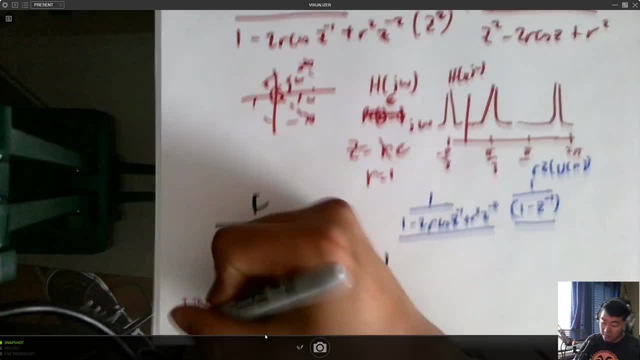 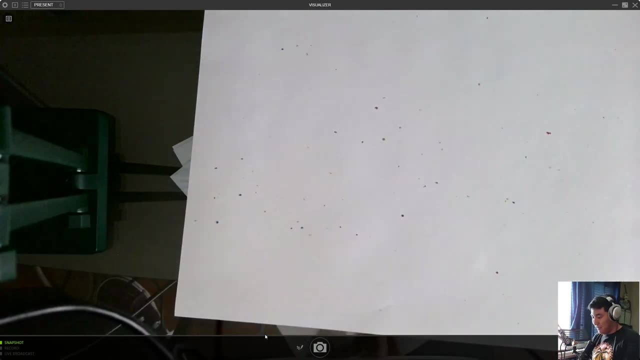 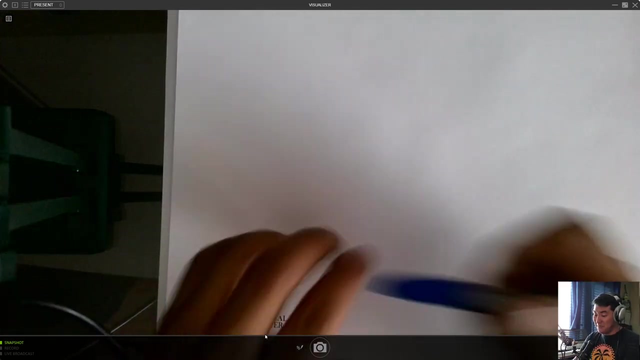 Hopefully this video is not too long. I'm trying to make sure it's not too long Because the last one took like a long time to publish And I'll just show you a really quick example. Make sure everyone's doing their own work. 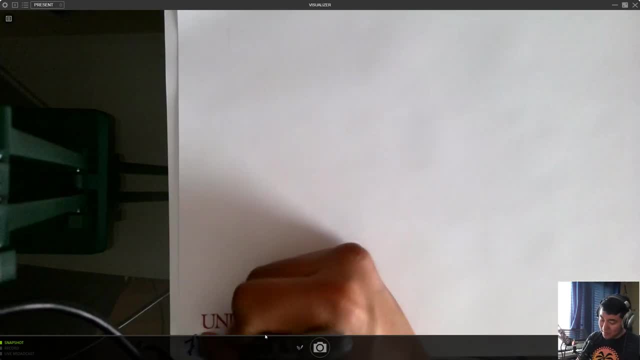 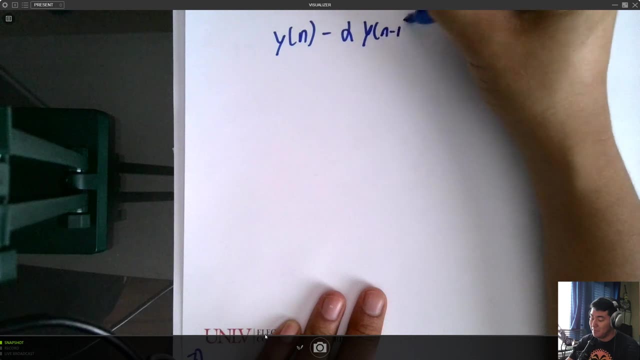 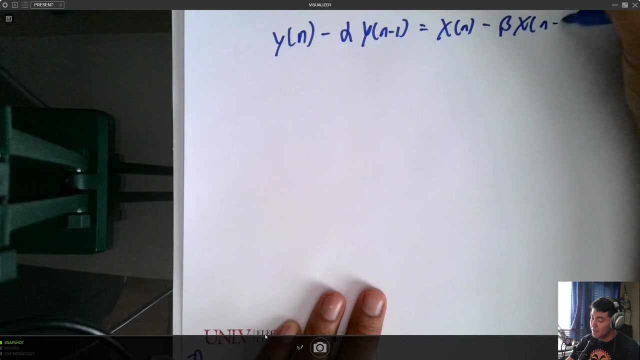 Seven. there we go. So if I had some system, Y of N minus, I don't know, Alpha of Y of N minus one is equal to X of N minus beta Minus, beta Minus one. That if we were taking this to the Z, transform the rule is well. 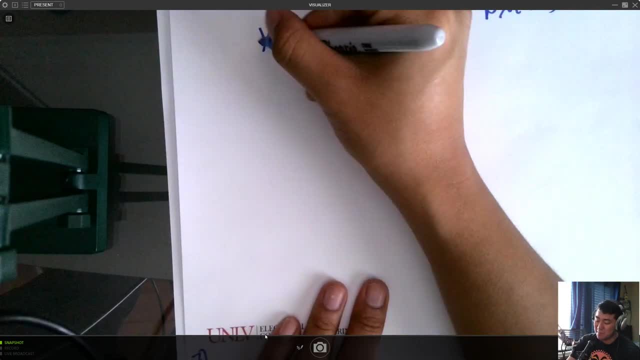 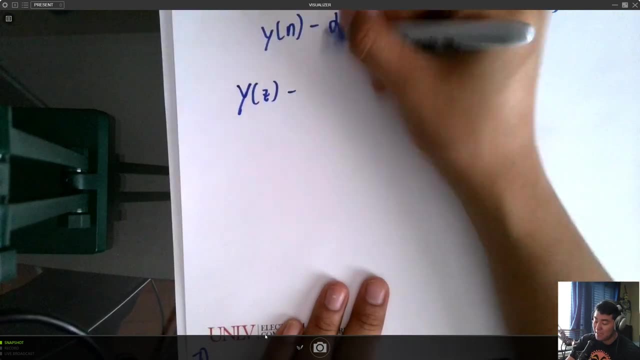 you just look at the delays. if there's a delay, you put a Z. So this right here, Y of N, the Z transform is going to be Y of Z minus Alpha. Well, if you take this to the Z transform, 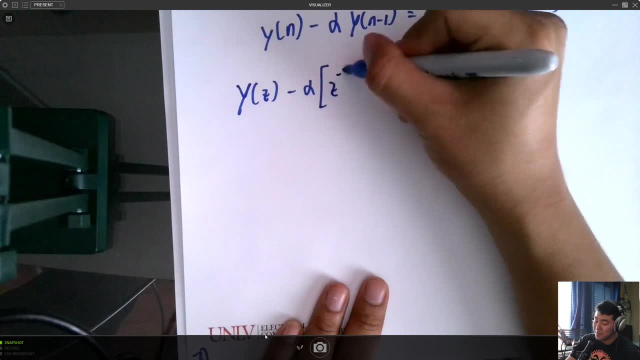 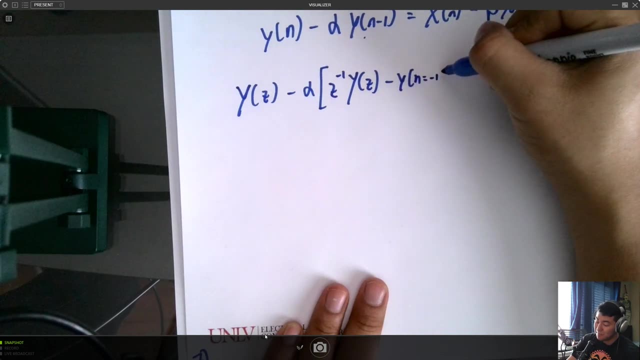 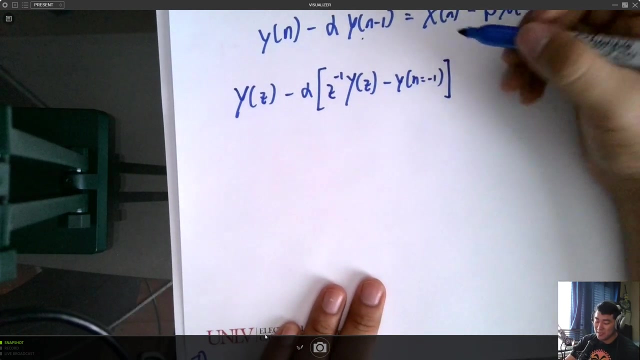 you actually notice that this actually comes up with a value of Z to the minus one. Y of Z minus a condition of N is equal to minus one. I think that's it. So we're looking at a previous value, But this is for saving your states, or what's your previous state? 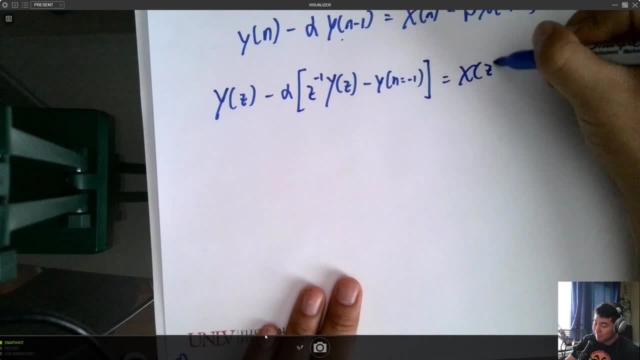 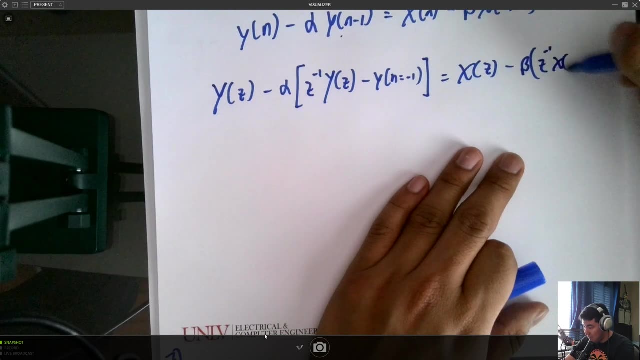 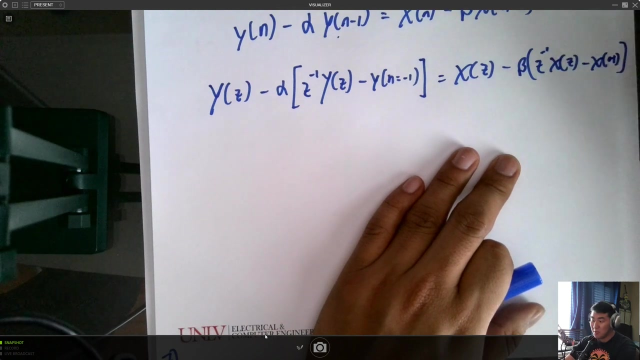 There are many numbers in your system: X of Z minus B, And the same thing applies with the ZX terms minus X of minus one. But for now we're going to assume that Y of N is equal to minus, one is equal to zero. 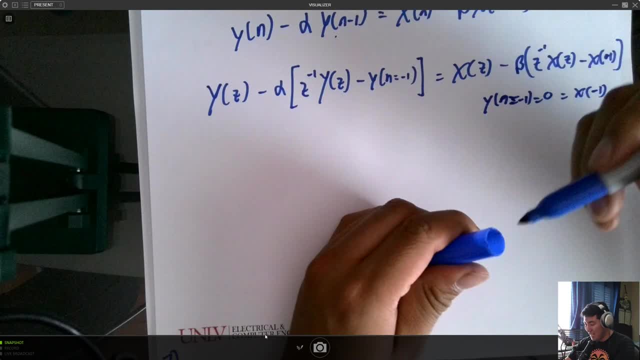 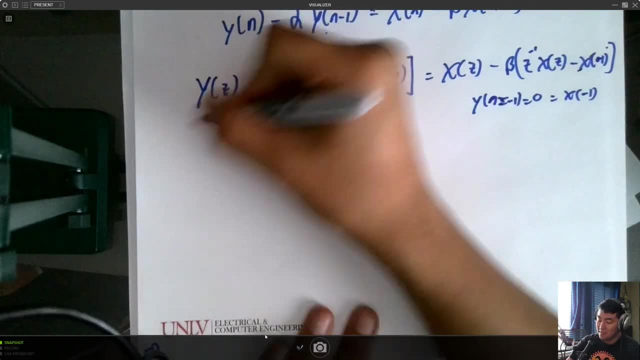 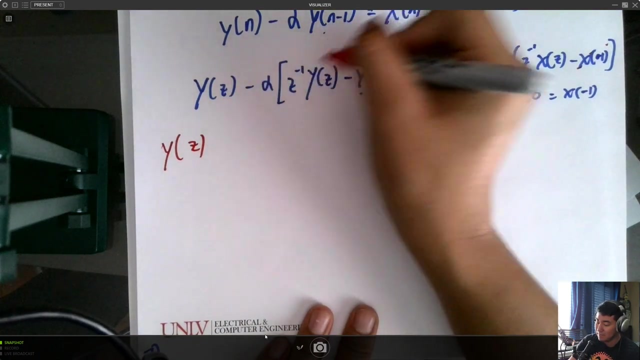 So we're going to assume that it's a clean system. We don't need to worry about this system right here. We don't need to worry about this. So if we were to just factor out all the Zs or the Ys, Y of Z, get one minus Alpha. 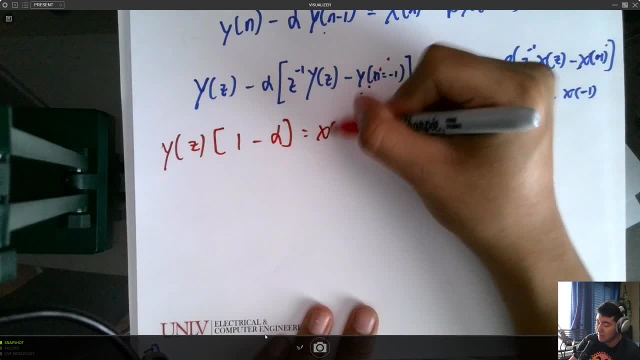 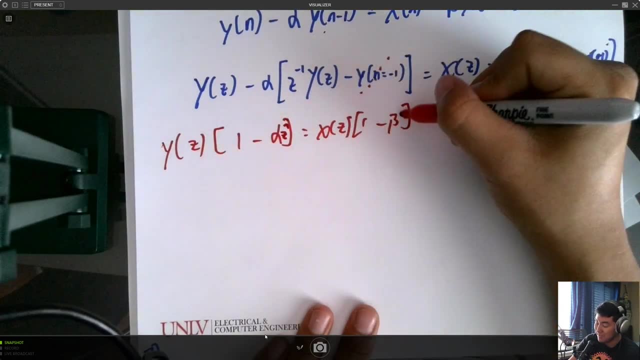 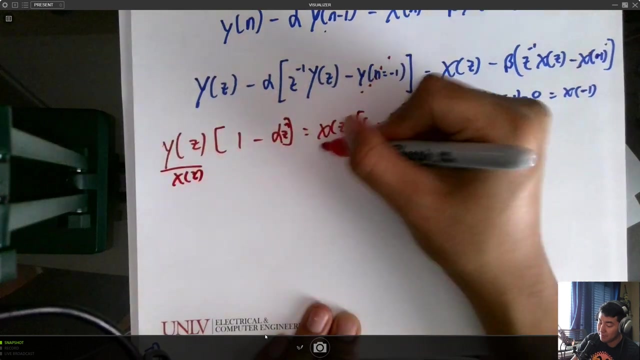 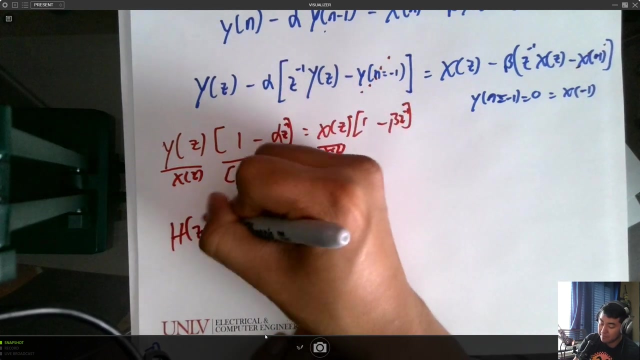 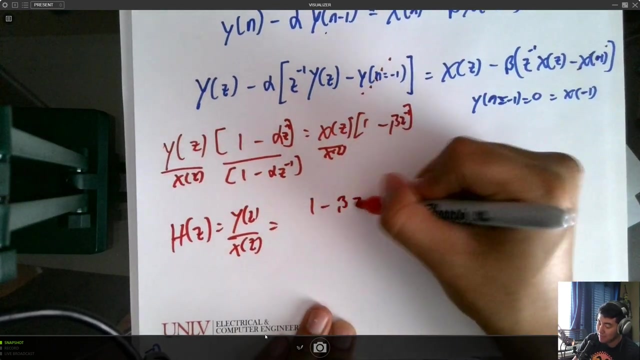 And And X of Z. One minus beta, Z minus one minus one. Then if we were to divide this by X of Z, X of Z, divide this by one minus Alpha to the Z minus one and H of Z, It's going to equal one minus beta Z to the minus one. 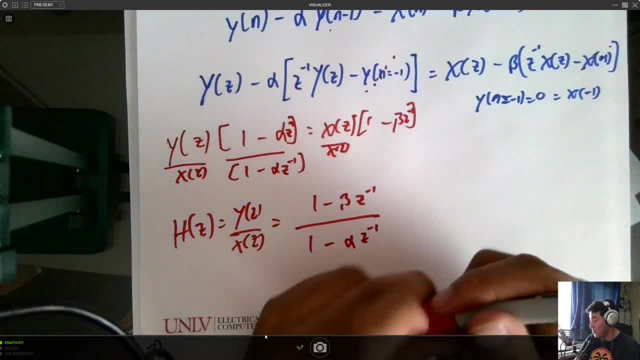 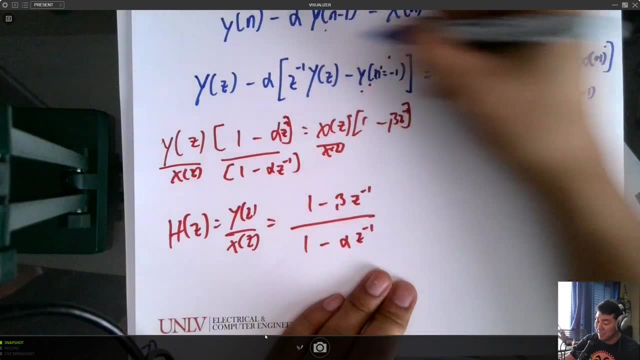 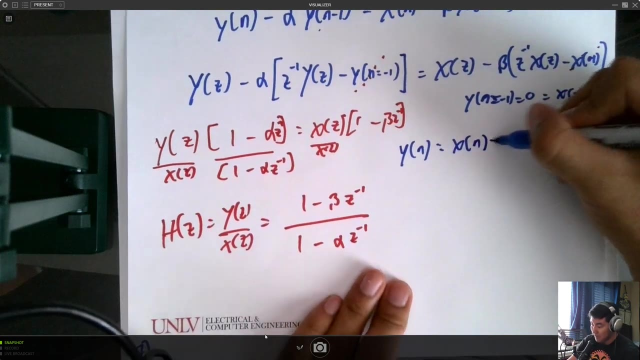 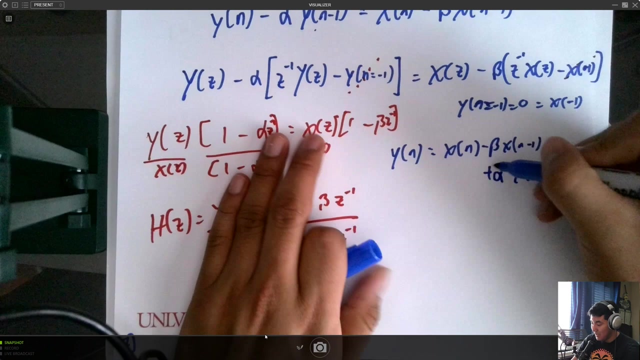 One minus Alpha, Z to the minus one. If we wanted to draw a quick block diagram, really quick block diagram, This is the transfer function of that. But if you wanted to get a quick block diagram, We can do X of N minus beta, X of N minus one plus Alpha, Y of N minus one. 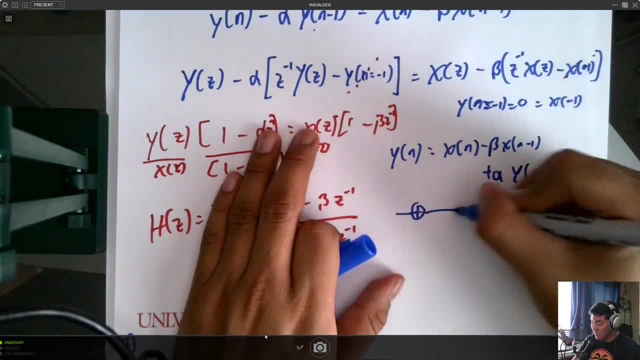 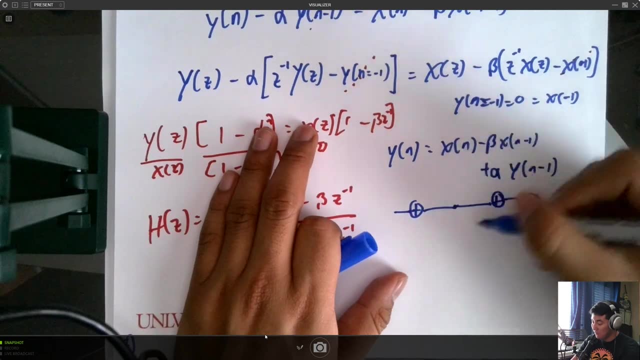 We notice that we have one delay block. if we were to do a transpose direct, Probably not transpose direct form two block. We have our input directly going into our output And we have two delays or not one delay. We have a positive Alpha. 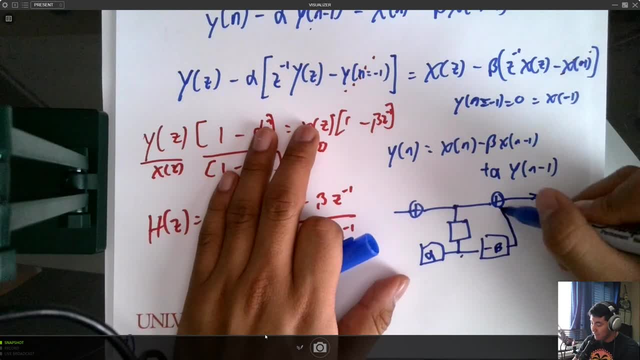 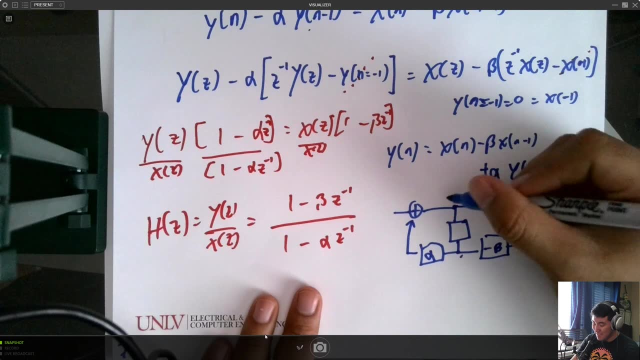 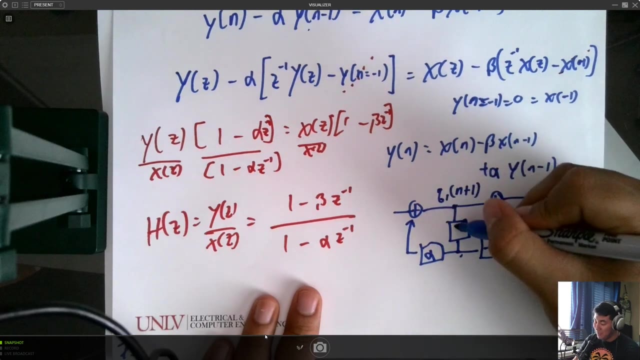 And we have a negative beta. So for your assignment you'll notice that. well, for the state space systems, Here's a hint. I will give it to you: Q of N, Of N plus one, into a Z to the minus one block. 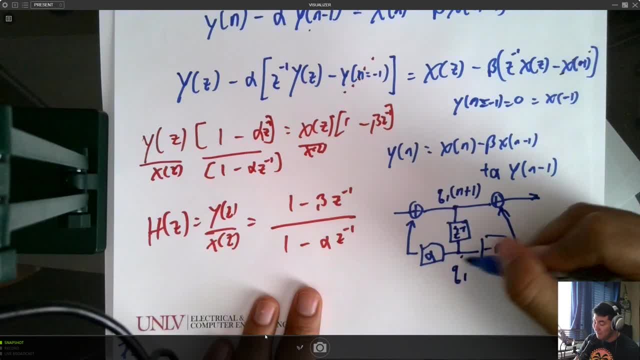 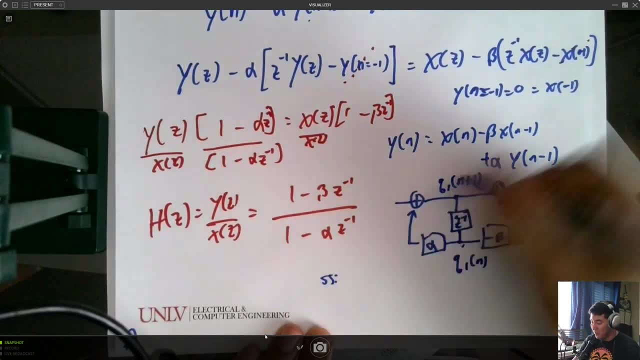 A delay is that it's going to turn into Q of one of N For your next state space systems or state space equations. Well, you're going to solve for the next state. So Q of one of N plus one is equal to the input. 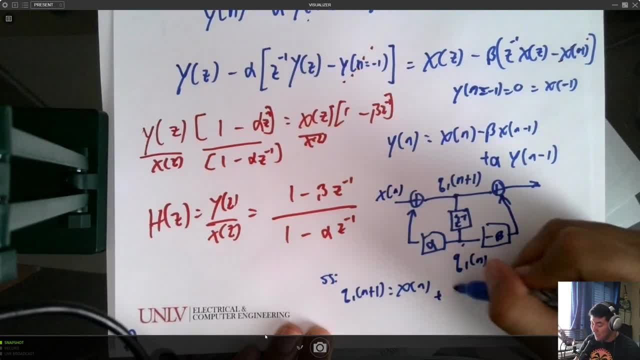 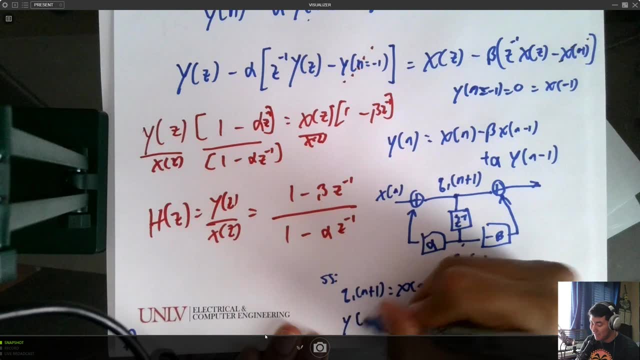 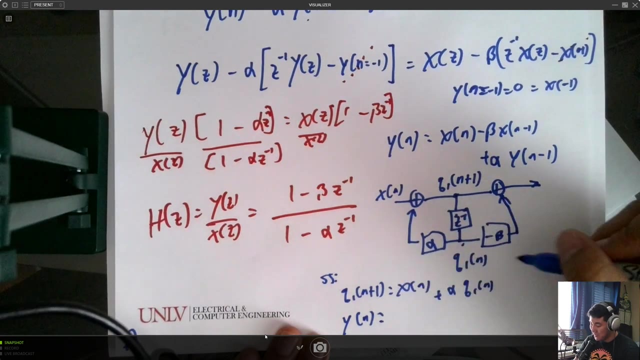 Don't forget that Plus Alpha of Q of one- And then you're going to look at your output- Y of N is equal to. well, whatever states here minus whatever is that there. So just to save on time, because this is right there, 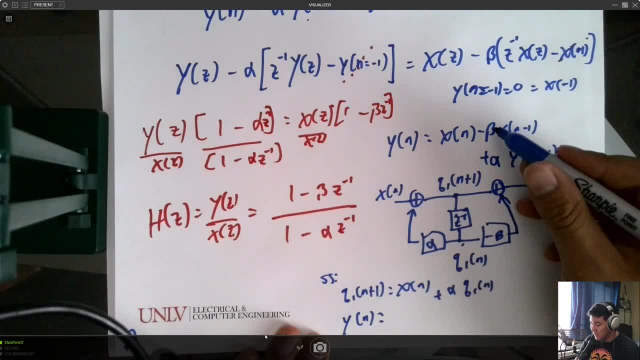 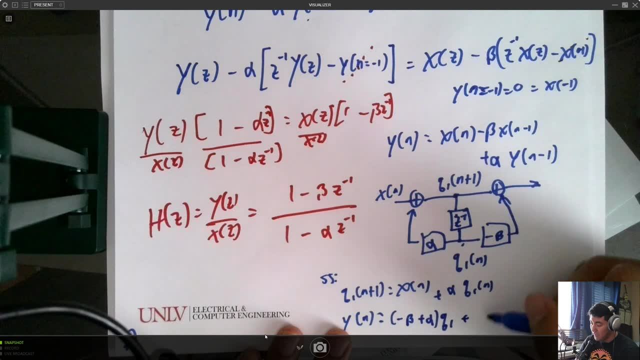 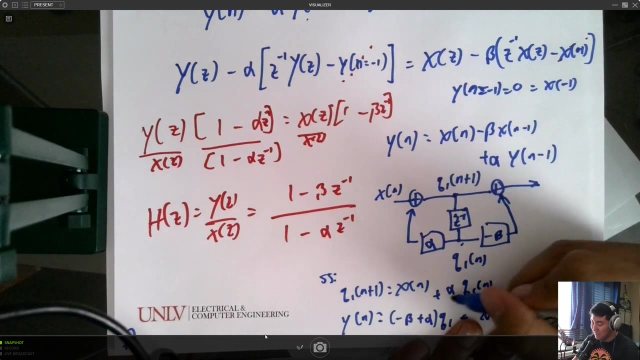 I look at. usually this one's a positive term, but that's okay. Minus B, plus Alpha Q of one, plus X of N. If you wanted to do your block diagrams, you notice that, well, A is going to be this little vector. 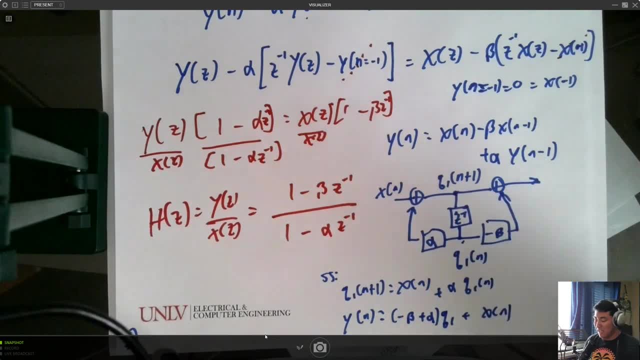 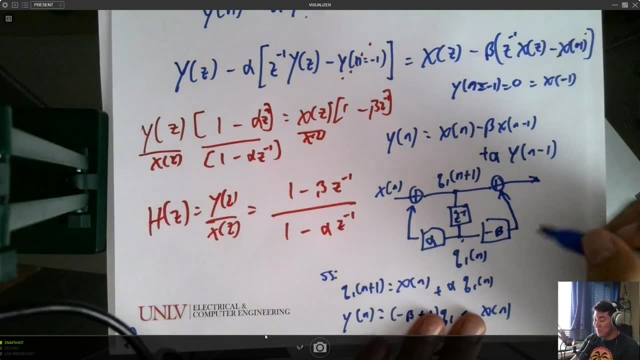 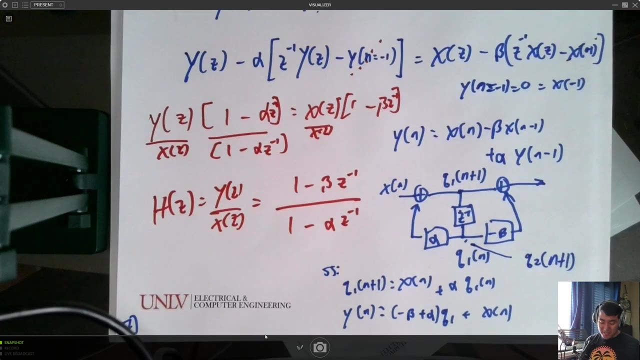 But the whole point is, this is the stuff you will have to do for a second order, differential or difference equation. You'll notice that you have to set this term to Q of two, of N plus one, and do that same process. How to check if your work's correct? 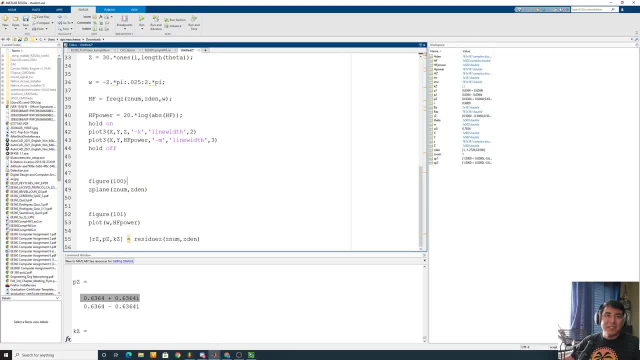 Well, you can go to MATLAB and let's see if I can show you this right here. Um, let's show you this. actually, Let's just briefly show you what's going on. Here we go. A couple of things I need to show you. 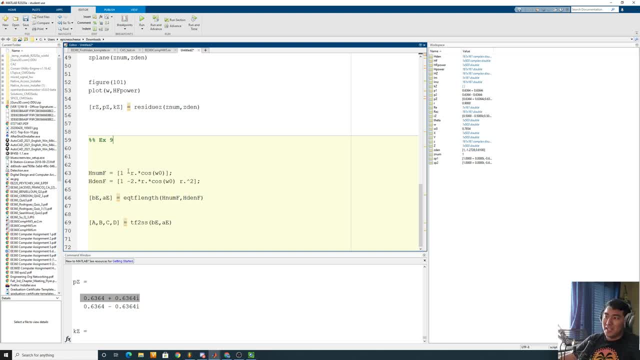 So this right here is probably what you're going to be seeing on your assignment. You'll see that, oh, here's this and here's your numerator And I look similar to your assignment, Here's your denominator, And then you're going to do EQTF: length of that system. 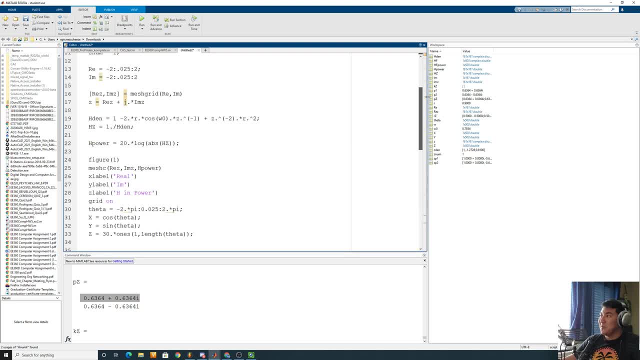 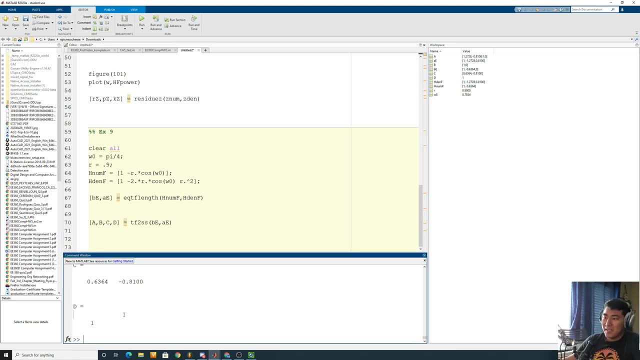 So you know what I'm going to do. I will do the following: Oh yeah, let's clear. all Get rid of that residue And there you go. So this is what you're going to be seeing, And note your hand calcs won't be matching this, but you got to prove that to yourself. 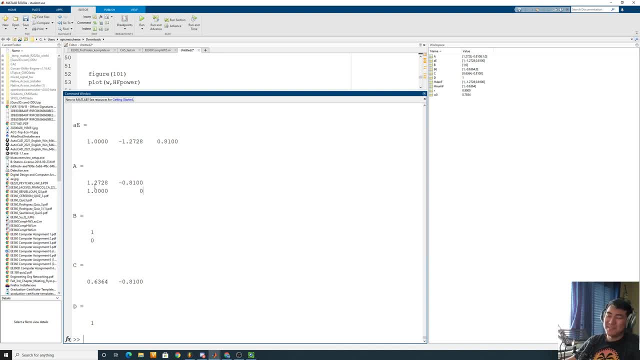 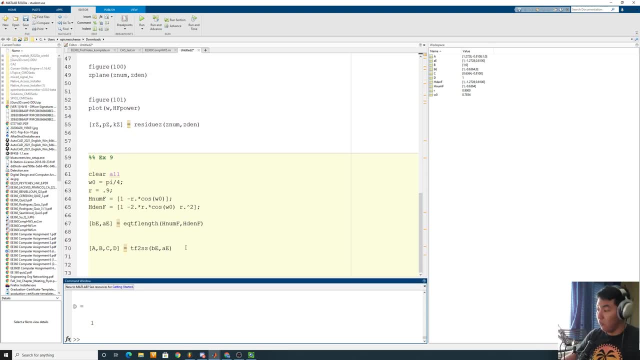 So can you do this? Are you able to do this? If you're not getting these numbers, then you mess up somewhere. So make sure you're able to do that. And I'll get to one more point, because this is going to be on the exam. 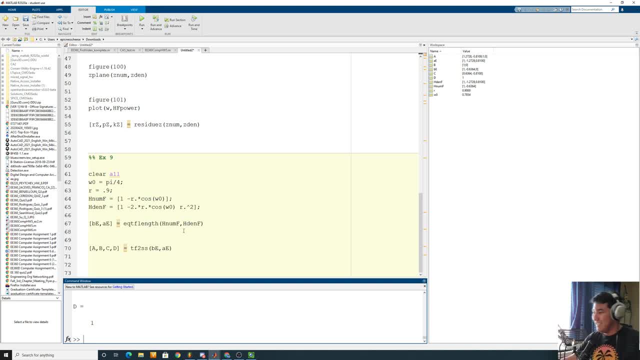 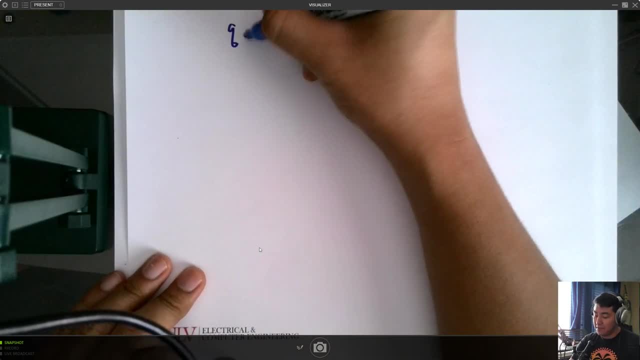 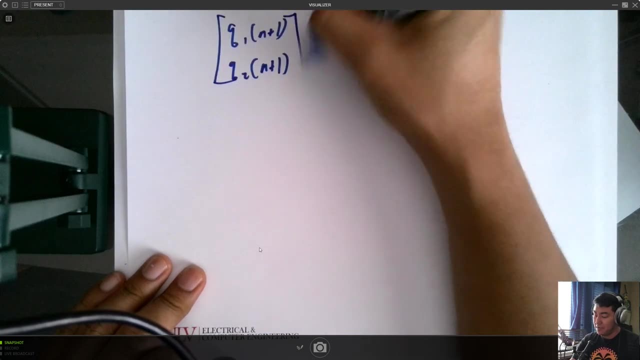 And you already know the proof to it. It's in the Laplace domain. I'll show you right here. So you're going to see something where you're going to have Q of one and plus one, Q of two and plus one. This is kind of your solution. 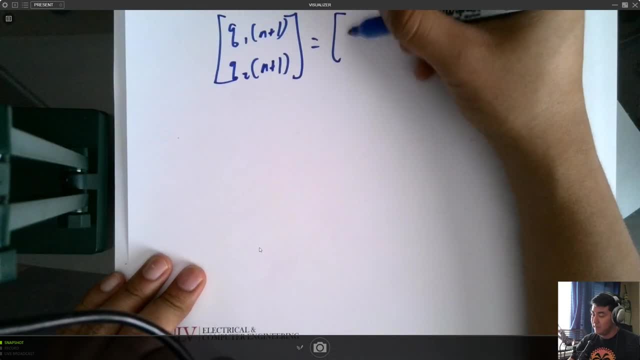 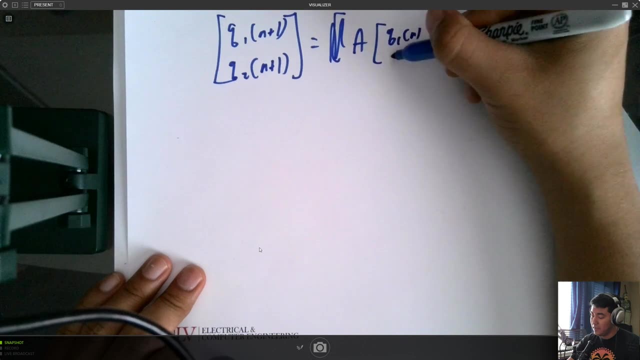 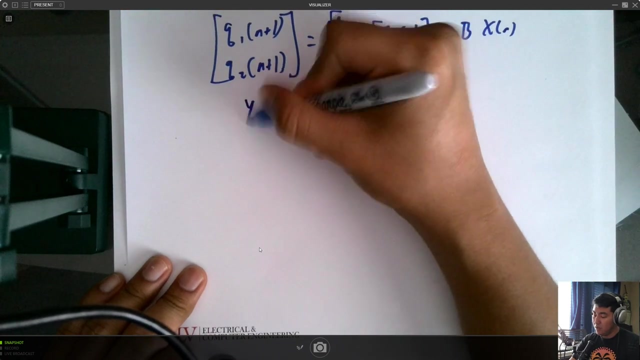 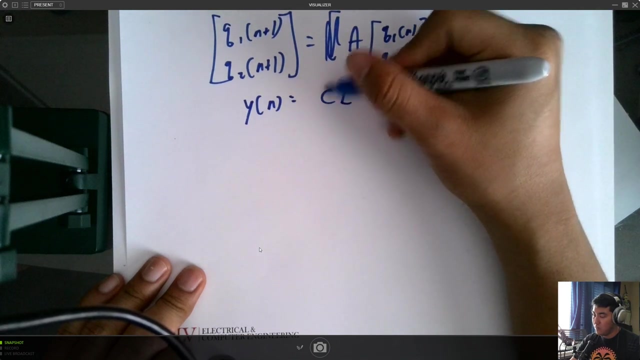 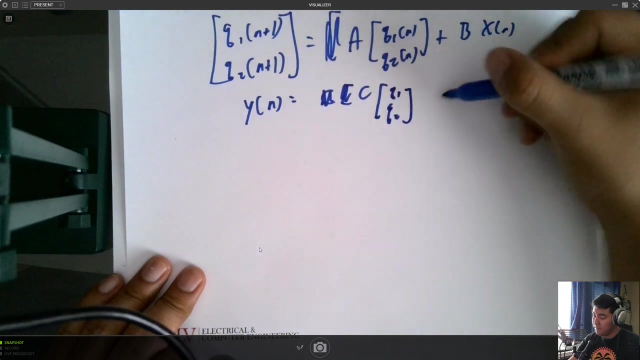 It's going to equal to some alpha, whatever alpha of Q of one of N, Q of two of N, plus beta X of N, then Y of N is equal to C of some Nazi, That's C, C of Q, one, Q, two plus D of X of N. 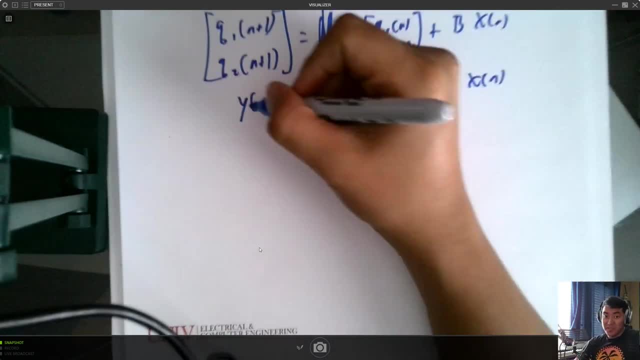 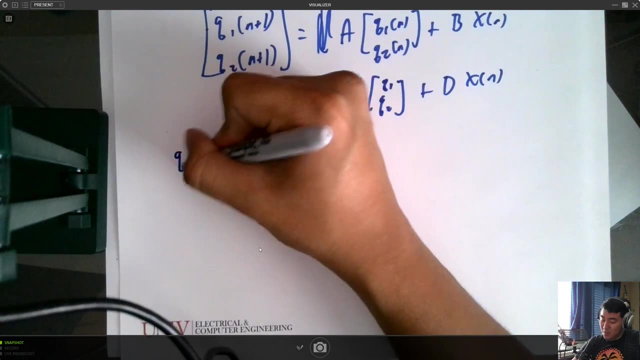 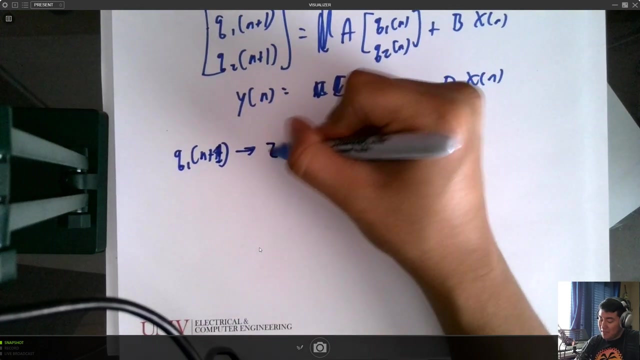 This is a two by two. So if you were to do this system, you note that if you were to go into the Z domain, Q of one of N plus one, one Z domain is going to have Z to the minus one Q. 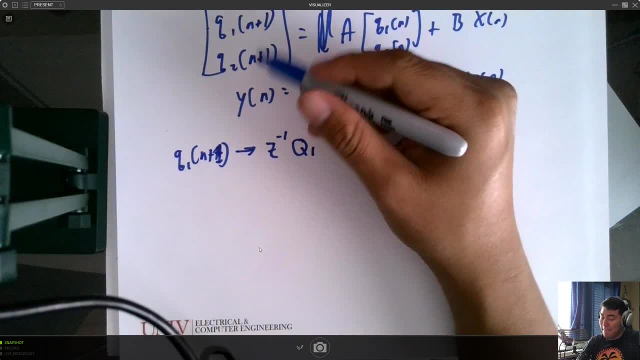 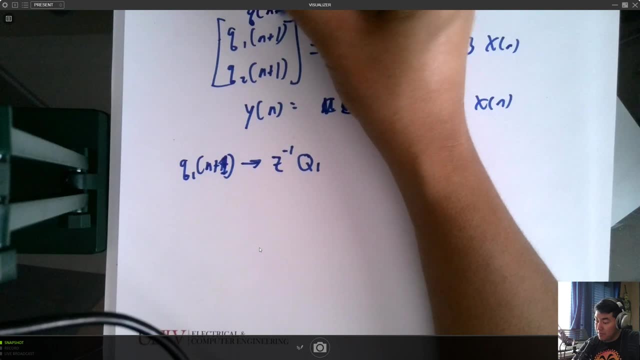 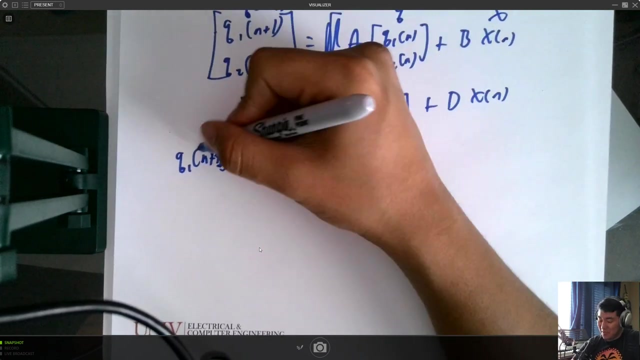 Let's call it Q. Yeah, let's just do that Q of one. So let's just call this one Q, Q, Q, dot or Q of N plus one X, And so basically, what I'm trying to say is this whole thing, this whole Q is going to turn into this. 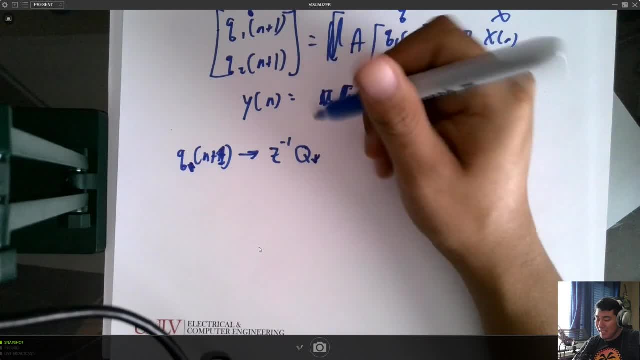 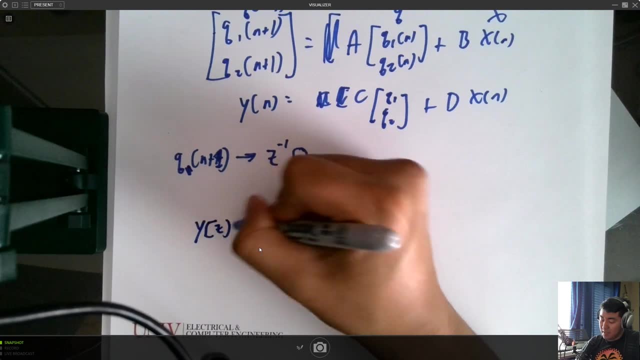 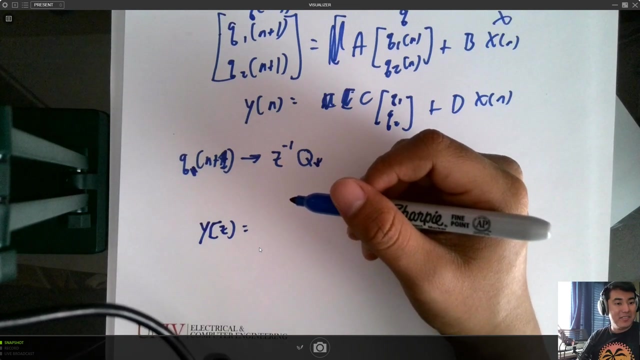 So you can prove the same theory And I think you'll get eventually to an equation where it's going to be Y of Z is going to equal. I think we just check what I have here just to help you, And you probably will see this on the exam. 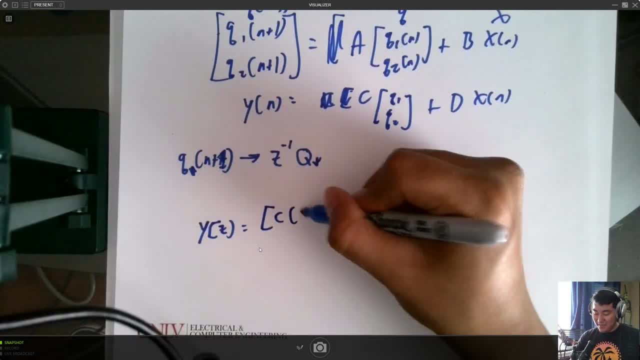 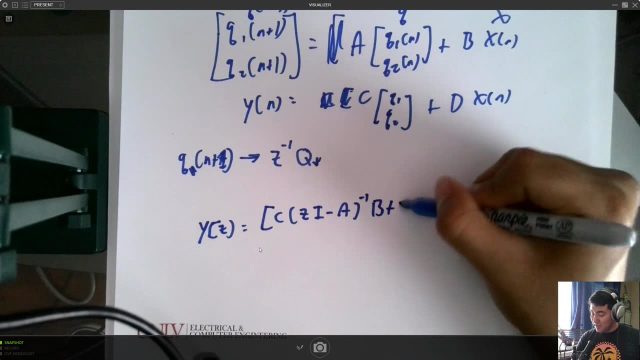 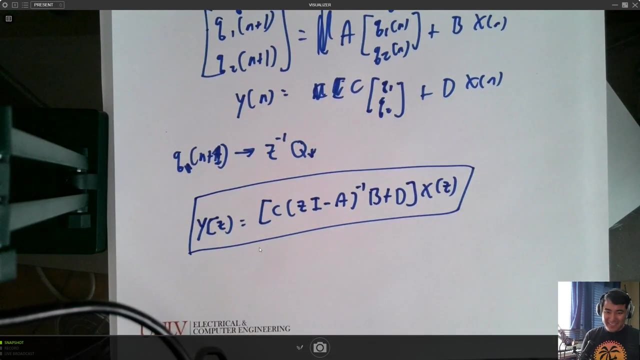 So you'll see the following: C of Z, I minus a minus one, B plus the X of Z. So try to prove this on your own. And you've already seen it. It's in the lost domain. It's the same thing. 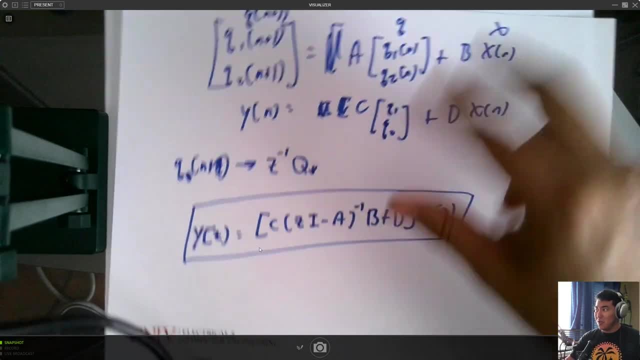 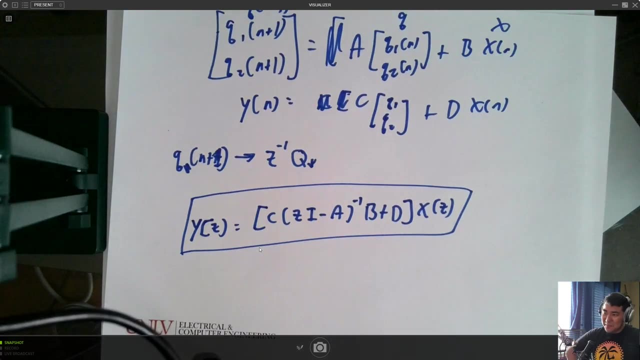 But if you can do from here to here- you know you got your alphas, your betas- Make sure you do that, Make sure you show your alphas and your betas. Can you do it? I just use the transfer function. 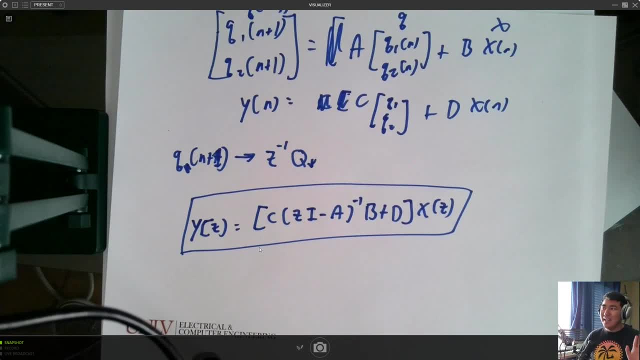 No, don't use the transfer function, Don't use TF to SS. Don't do that, Or you will do that for showing your work like proving your work. But the whole point is, can you do it by hand? If you can do it by hand, and you can do this, and then you can find H of N. 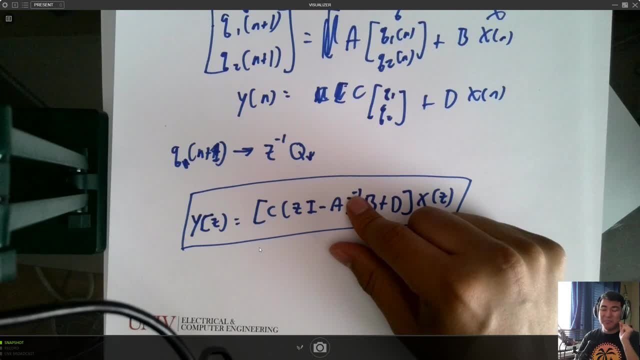 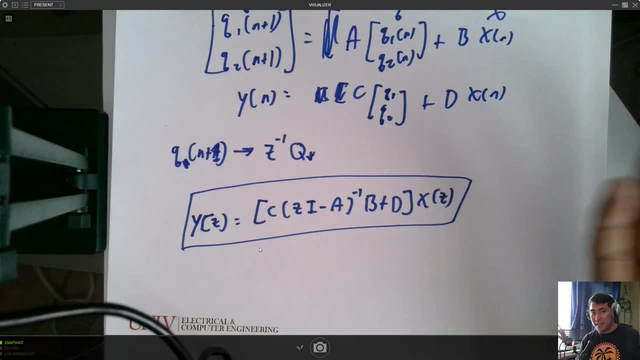 This right here will give you your residues. Can you find the residues by partial fraction expansion? You're done. That's the final. Well, kind of the final, It's your next exam. So if you're able to do this on your own to a point where like, oh you know. 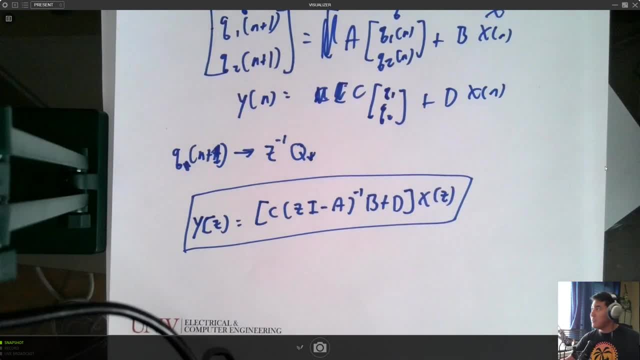 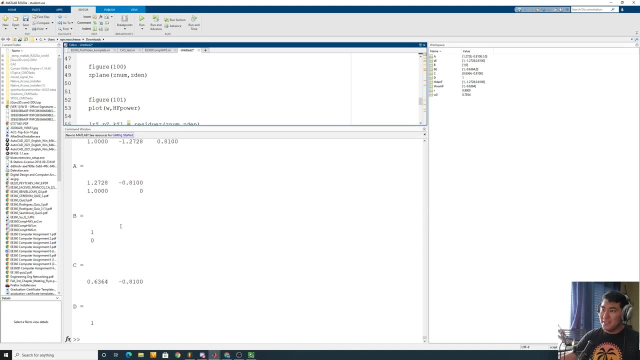 alphas, you know your I's, C's, B's and D's, then you can solve for anything you want. So right here, let me show you this. So that's your system, right there. And now you're saying: OK, David, now we have a system. 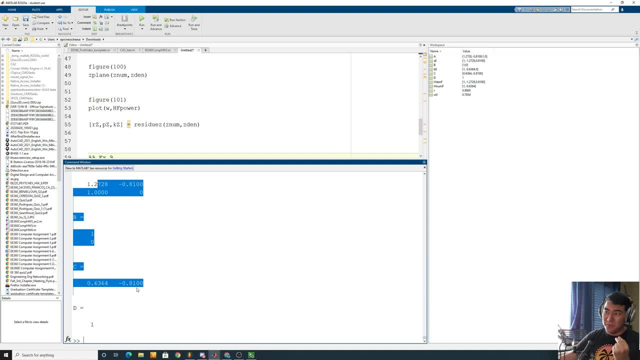 Now you know that this is your, what you're the answer you're looking for. You better know how to do this and you better know how to get the actual transfer function from these coefficients. Can you do it? If you can't do this- and yeah, you're not going to have a fun time- 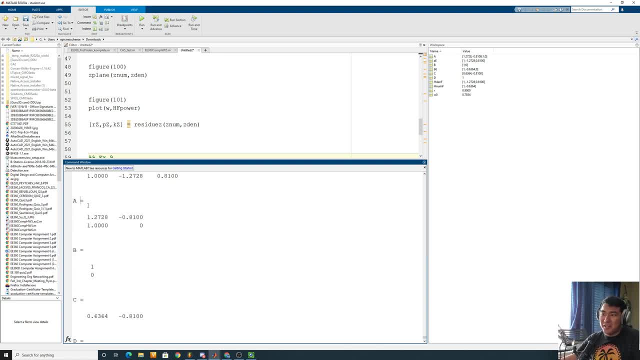 on your exam. so make sure, try to do this on your own. A, B, C, D. If you can find H of N from these coefficients, from these numbers, from this equation, then you're set, you're golden for this class. 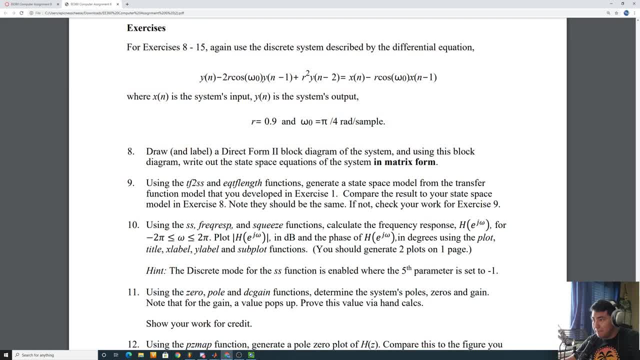 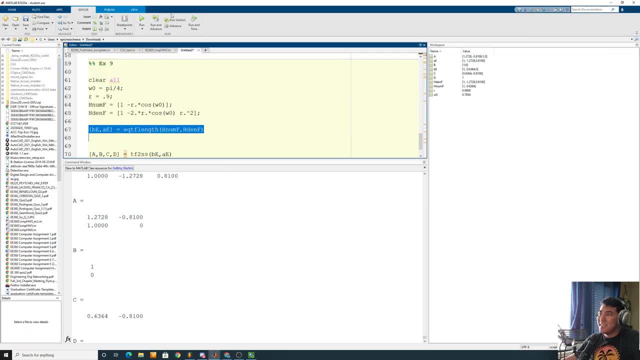 And let's try to do a little bit of your assignment. Oh, I should probably show you what this does. So this basically does At nine. well, it just turns it into some coefficients. If this were Z squared, Z minus C, one zero. 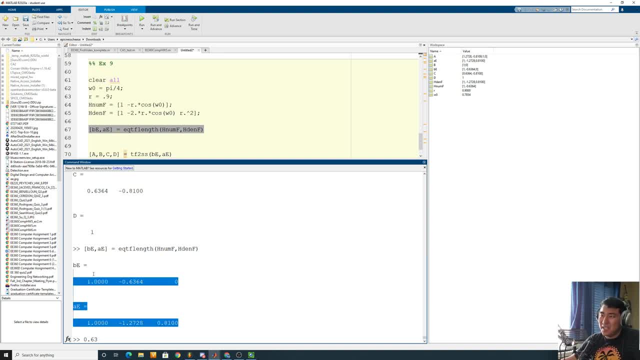 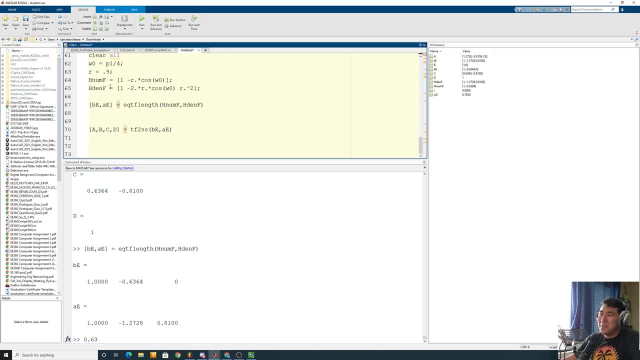 And it basically just shows you the polls. Don't worry, this is not that bad. You can use this to prove that, oh, you've done a good job, But yeah, don't worry. Actually, what it basically does is like: oh, it just doesn't assume. it's like this: 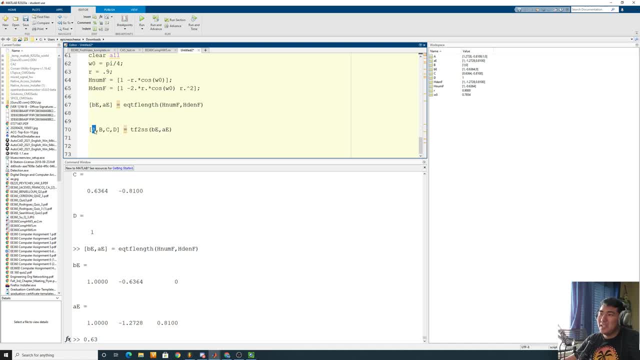 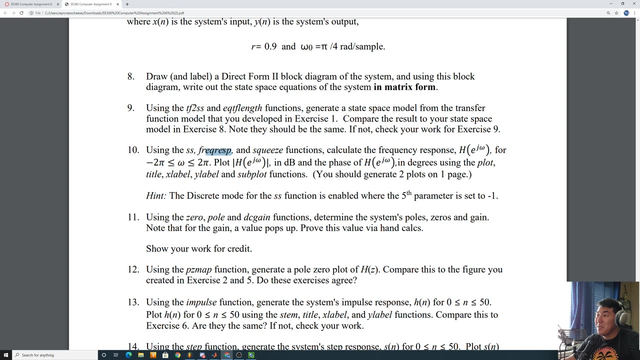 So it takes this and takes to this, and it's easy to Put it in the A, B, C, D domain. So that's that. Oh, that's a different assignment. Let's try to do the next part. This is all the same. 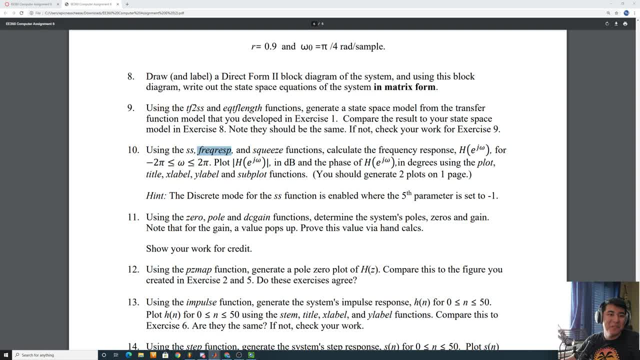 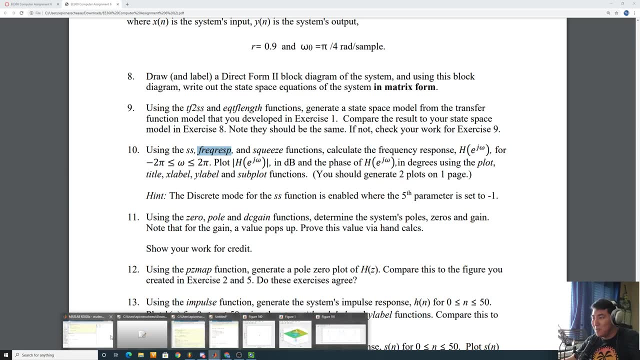 Ah, I think I need to show you one thing, but I don't know if it's going to be a problem. Let me see We go Rocking system. So there's one thing I got to show you, And this is something you have to be aware of. 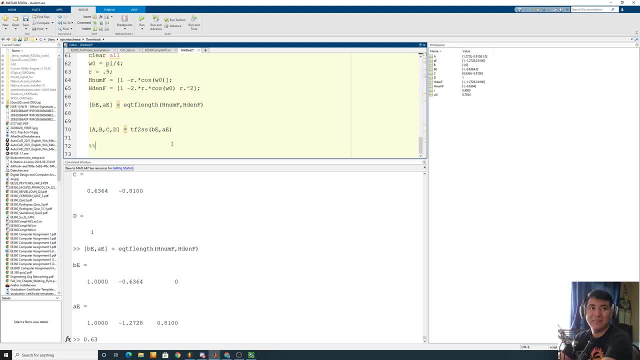 If you're trying to find your system, like, okay, my, let's actually just copy it from here. So if you were going to take some system and you're like, okay, now let's turn it into a system using the state space. 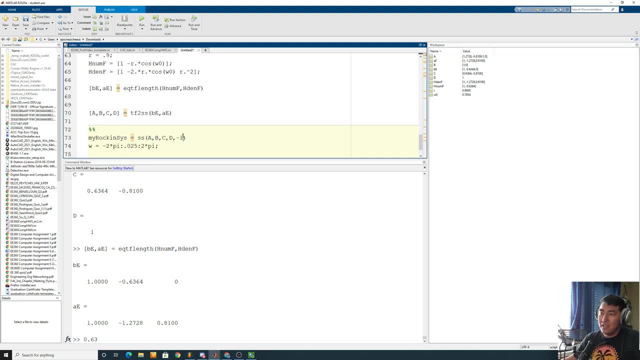 equation like the state space function ABCD. If you were to not put this right there, that turns it into an analog system. and then your system is like: oh gosh, it doesn't work. to turn it into the discrete domain. to turn on the discrete mode. 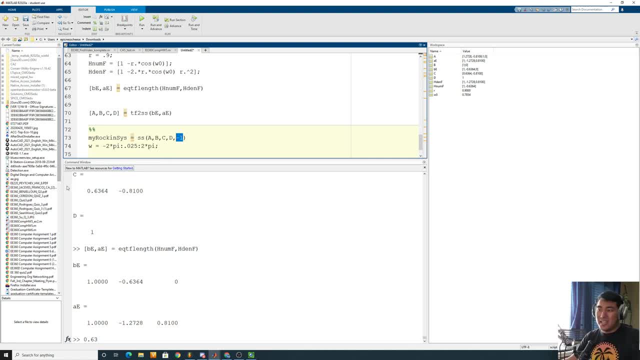 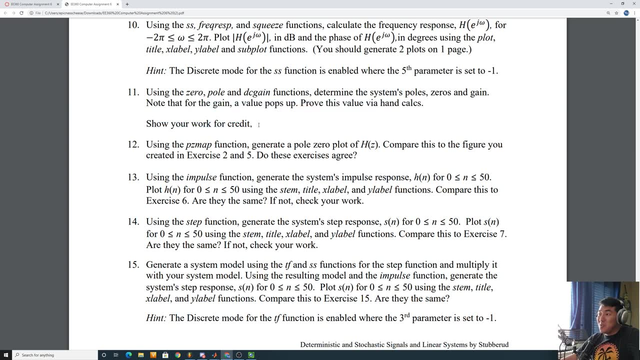 You put this minus one there. So that's how you would approach that, And I think, after doing that, everything's the same- How to show your work for this one. Well, you'll see that a DC game pops up, So let me show you one thing. 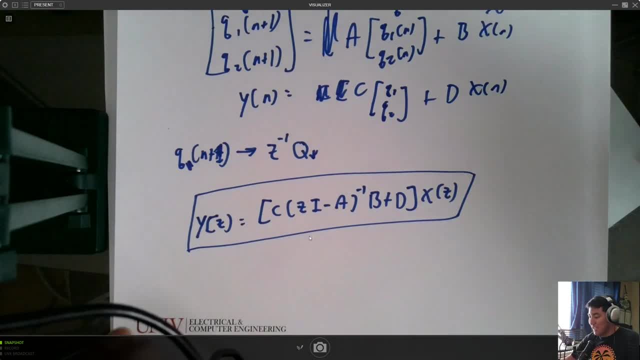 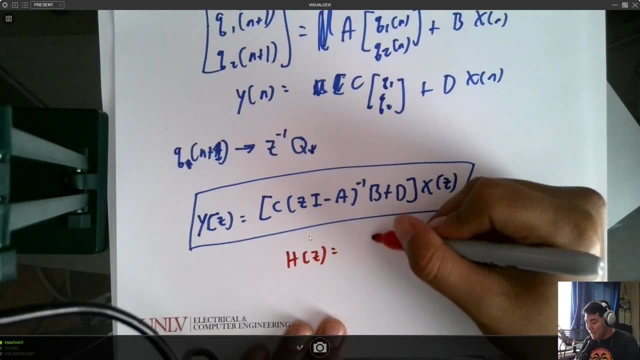 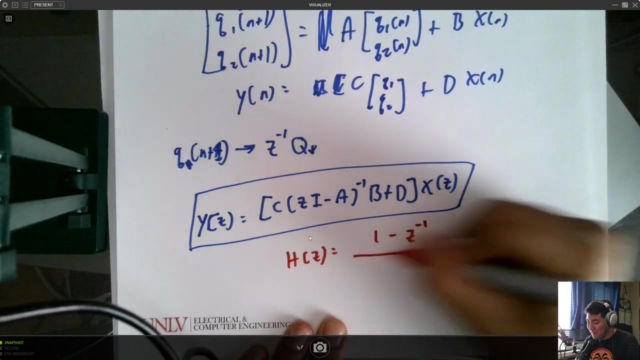 I'm going to wrap everything up in one big video and we can start with. I don't know, let's just do: H of Z is equal to what I want to do. One minus Z to the minus one, one minus two Z to the minus one, Z to the minus two. 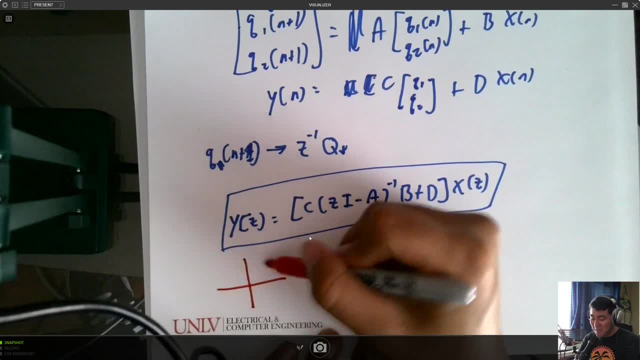 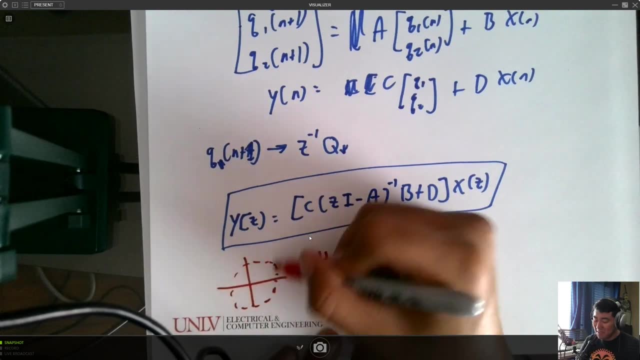 So, on the unit circle, you've probably probably heard me say DC. what's DC? or frequency? The unit circle is something we can, like you know, change our frequency. So if we were at, F is equal to you know some point here. 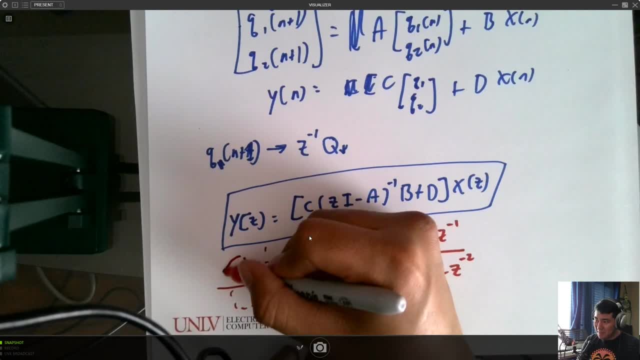 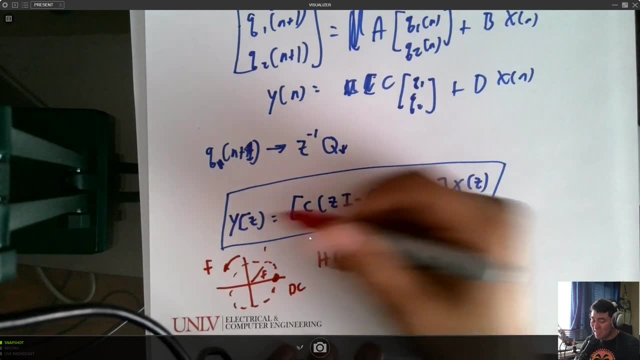 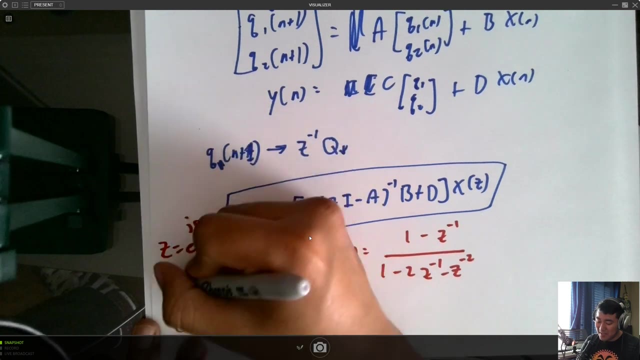 we can go to, like you know, our highest frequency here. So F increases as we spin around the circle. But if we go to this point right here, that's our DC value. So that means that's where Z is equal to E, to the J, zero. 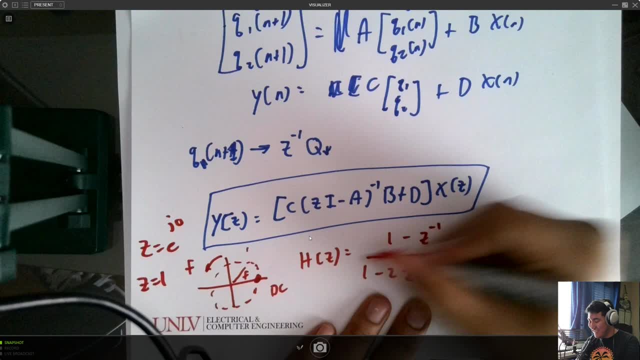 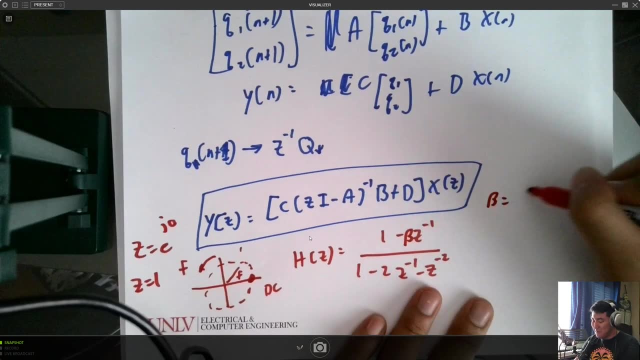 Z is equal to one. So all you got to do is: well, you're going to probably suppose this is a B term right there, and suppose B is equal to point two or something like that. Then if you were to do: oh, if Z is equal to one. 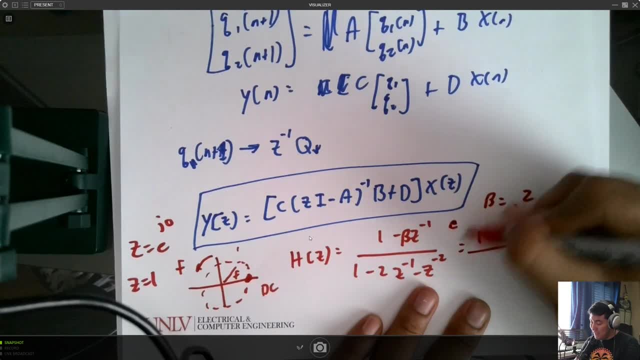 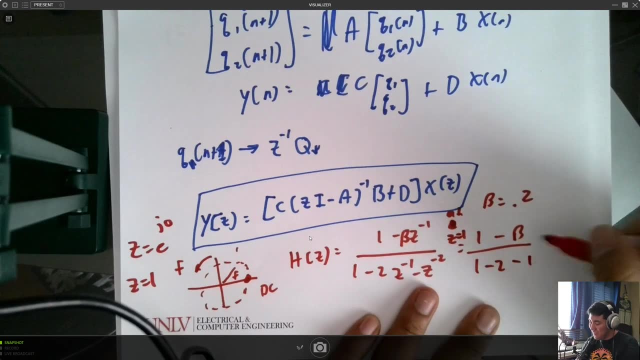 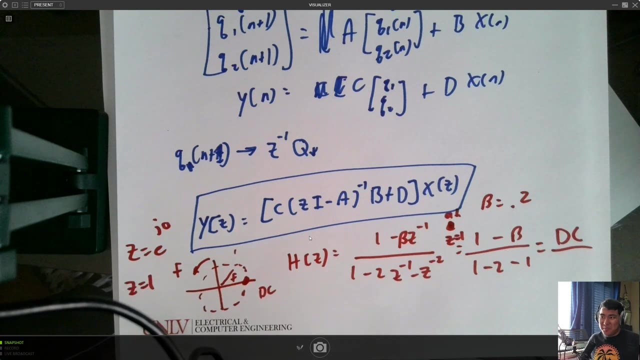 then that means one minus B at at Z is equal to one. one minus two minus one, And then you get some DC gain. So that's basically what your system does. If you turn on your system, what's the response? What does it do at DC? 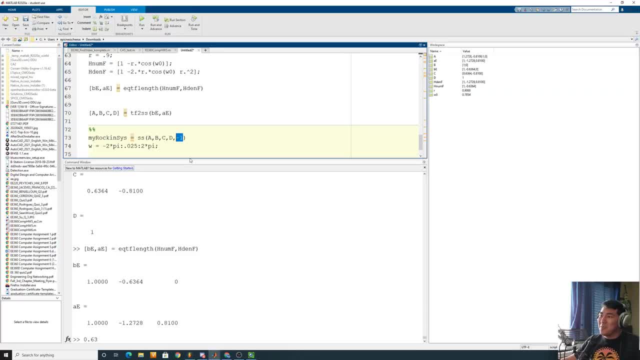 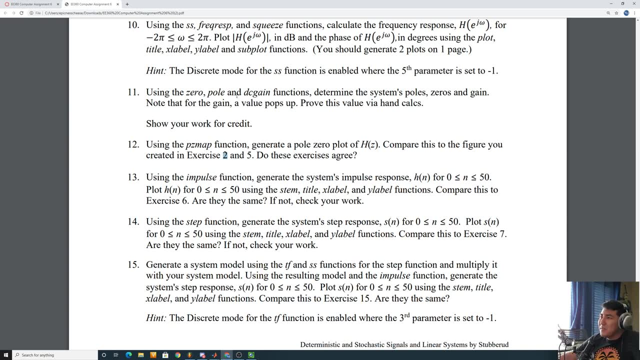 So that's your DC gain. So that should hopefully get you going with what's going on. Are you understanding what's going on? No, it's OK, There's go. I'm trying to see if there's any trouble for this. 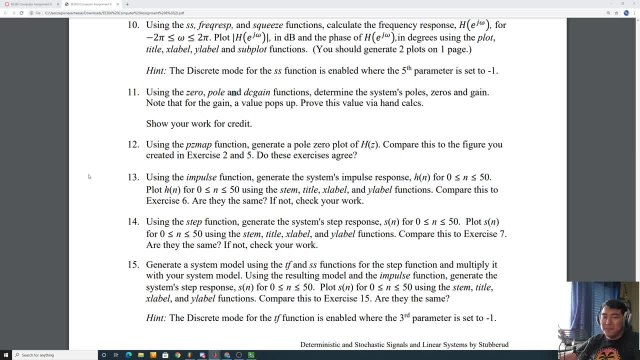 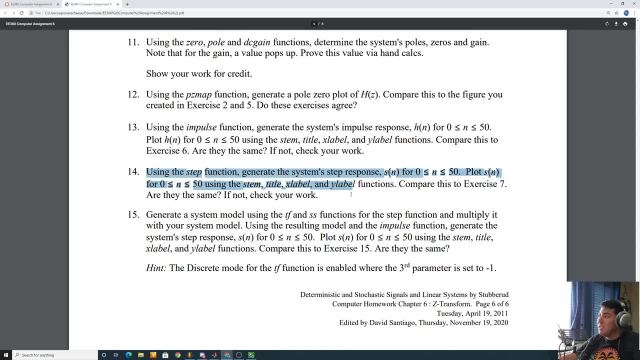 And yeah, it's all the same assignment. If you understand the previous assignment, then this assignment should be really, you know, straightforward. you know the step function, That's really easy. The impulse and check. Yeah, it's all the same. 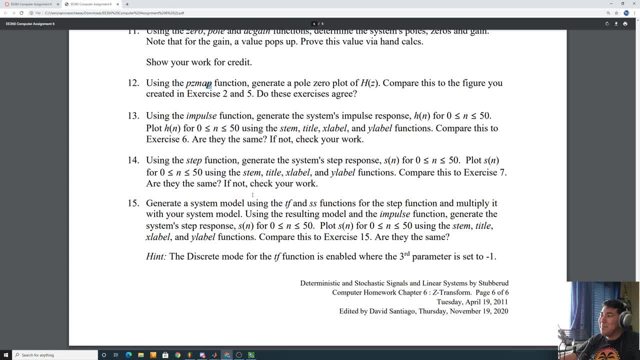 It's all really not that bad. Do you understand what's going on with PZMap? This right here might be a little. well, it's not that confusing. if you understand what's going on, you know you're convolving or multiplying your unit step. 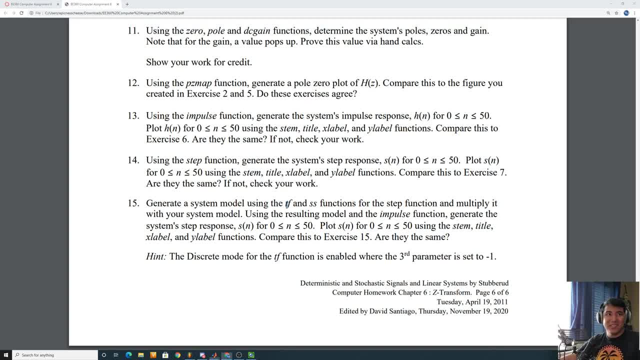 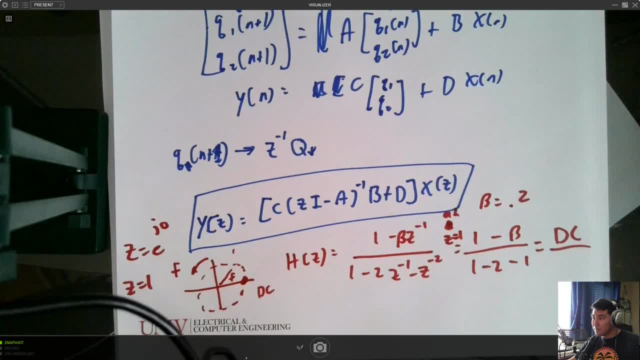 to your actual system. you already know how to do that from the previous assignment. All you do is well, you look at the numerators. you know that. Well, let me just show you one last thing. If you were to do, 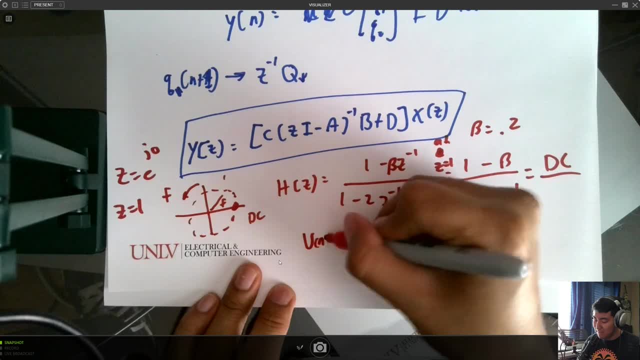 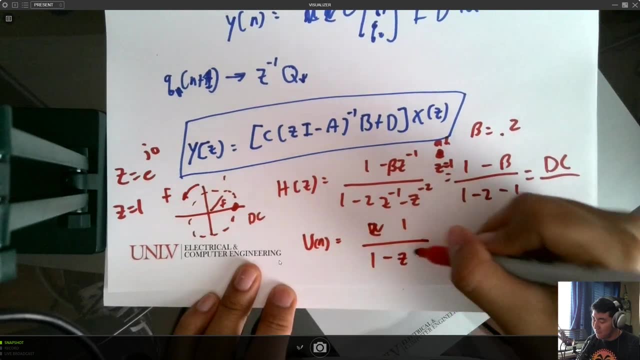 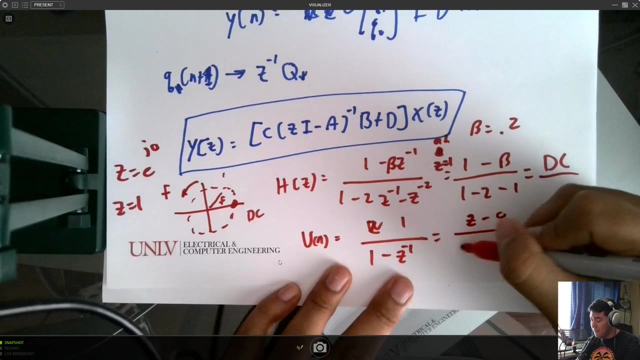 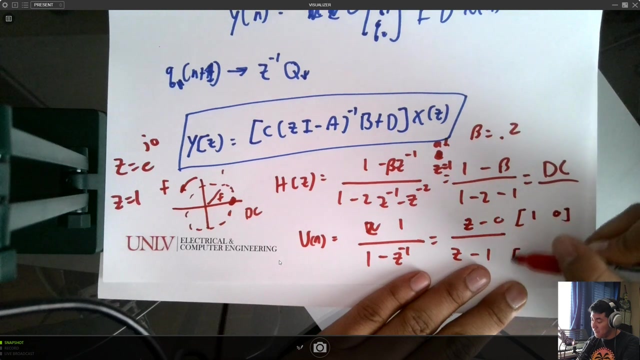 the unit step, unit step of n is going to be- well, you already know this, one minus z to the minus one, which is also equal to z minus zero, z minus one. So if you put these in vectors, one zero, one minus one. 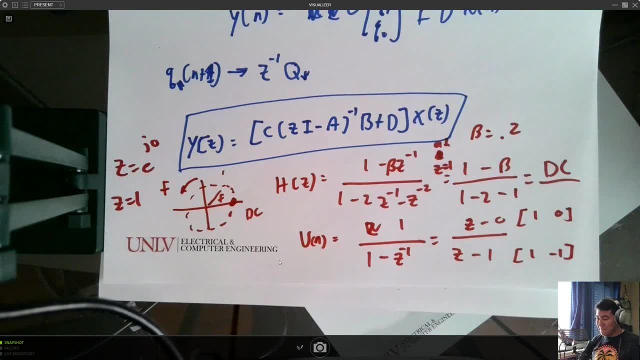 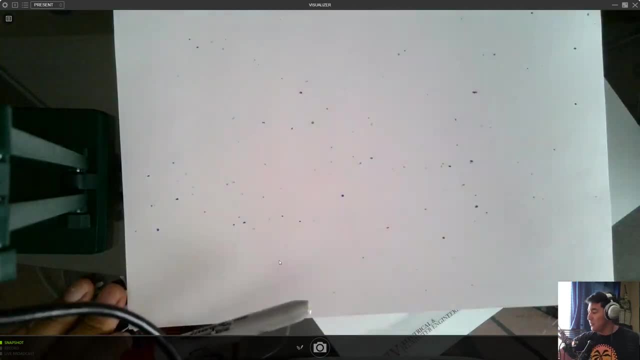 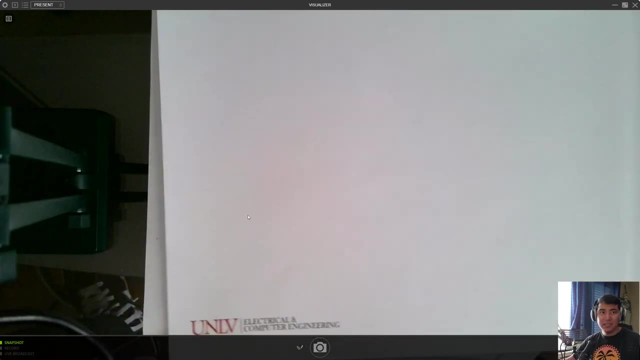 Now you can solve for your system using the transfer function, If you were to use. okay, let's just show you a little demonstration. Hopefully everyone knows how to do this. I don't know. It's okay, man, So let me just show you actually. 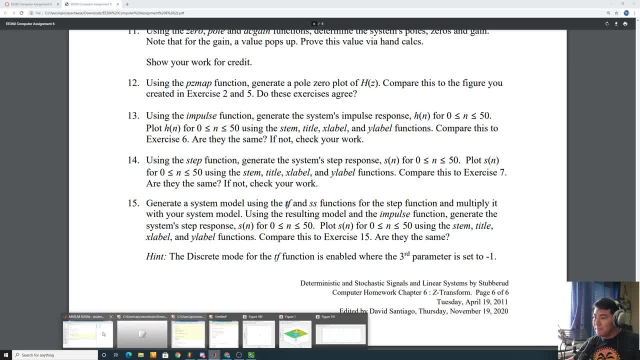 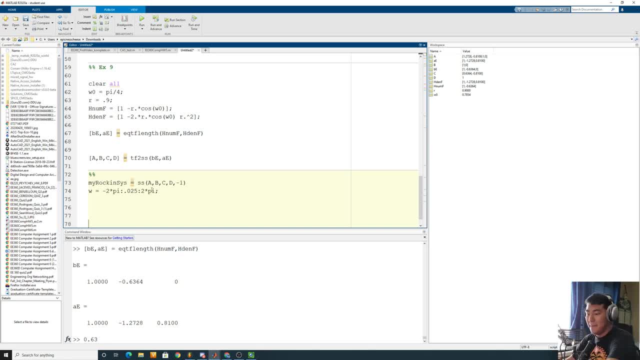 Let's just show you right here. There we go. I'm almost at the hour. Okay, If we were to go into z domain, that's it. And now you can use your transfer function. Let me show you that And you can multiply this. 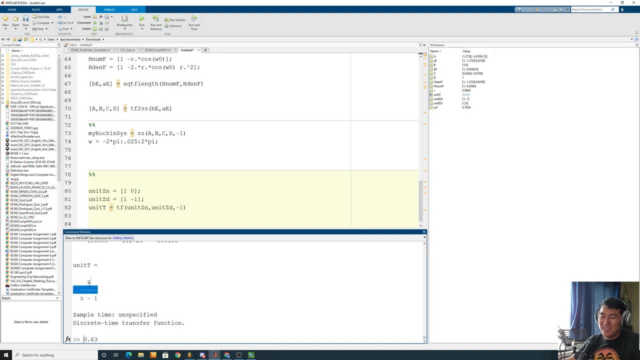 So don't forget that. And then You can't multiply this directly. You need to turn this into the space State based representations, Turn this into a state space. You know, using the SS function, just punching this system into SS. 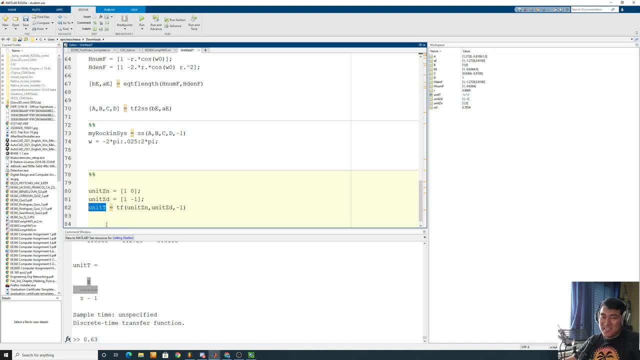 And then you're done. Multiply whatever system you created with whatever this system is, And then do the impulse and you're done. So really simple assignment. This is as much as I can show you And hopefully, Yeah, this should be a really easy assignment. 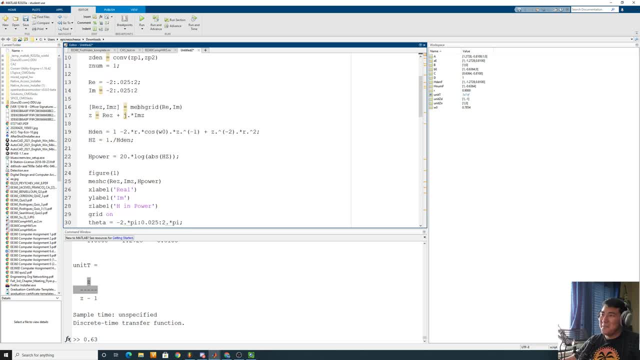 Number one should be just like: yeah, the first half is all just breeze. The only problem you might have is probably example nine, but it's not that bad. Honestly, just draw your system. You already know how to check your answers. 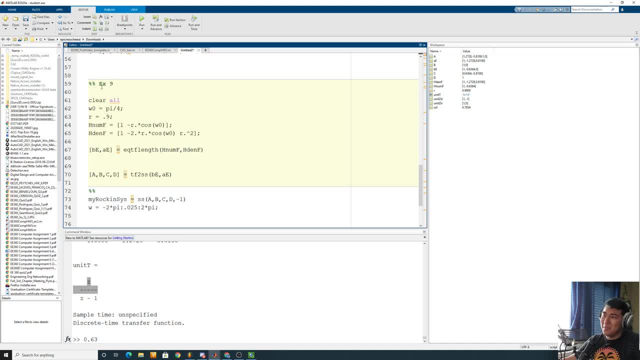 That's with this, So make sure you get it right. We'll be checking. the credit goes to number nine and number one. If you can do those, then you're set for an exam, And Yeah, that's basically it. So. 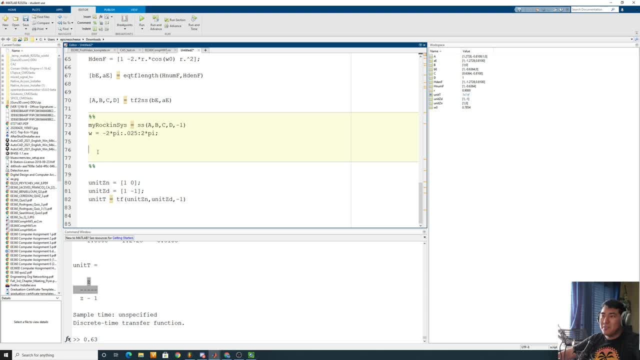 I don't know if I'll be making other other videos after this. I think this is probably going to be the last one. Wanted to show you some other cool stuff such as Well, I can show you one last thing. This is probably if you want to go into a systems design. 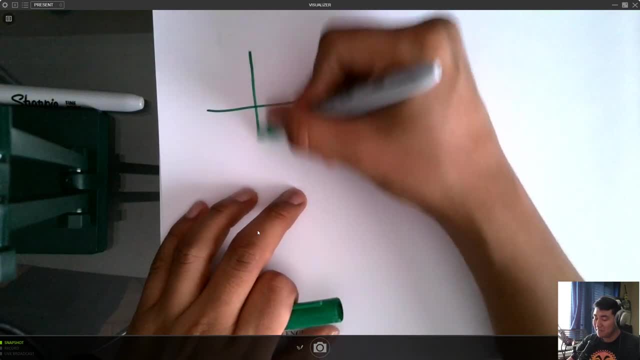 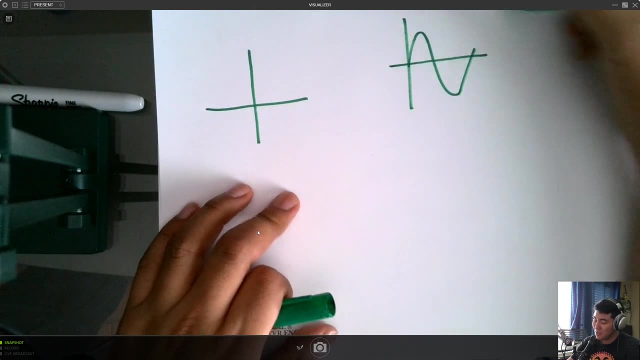 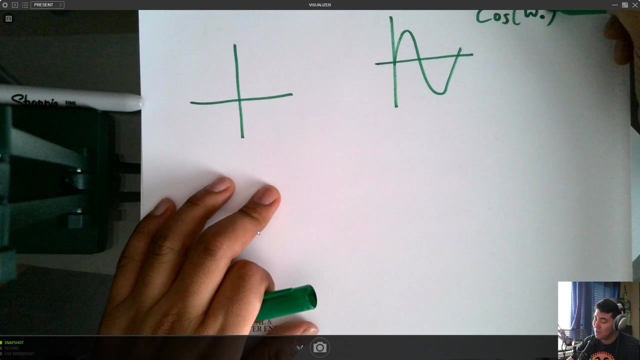 And you're probably saying, well, OK, David, so what do I want to do? So suppose I had some, you know some signal right here. like you know, it's a cosine signal, cosine function, cosine of, let's just say, omega naught, and it's just, you know, spinning in a circle. 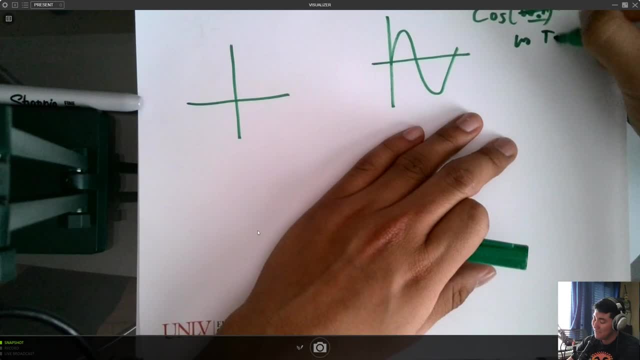 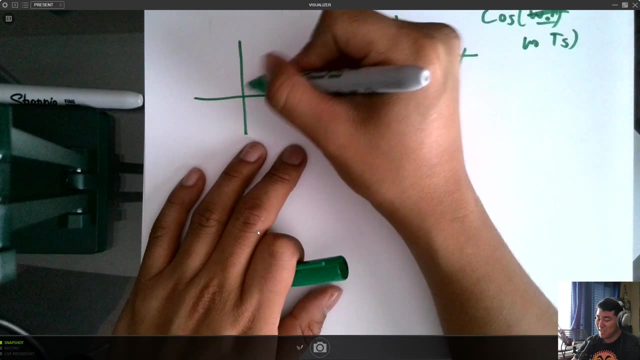 Actually they can not of T of S because what I'm going to call it. So if you wanted to take this and transform it into the Z transform, you're going to notice that well, it's going to have some resonating frequency. 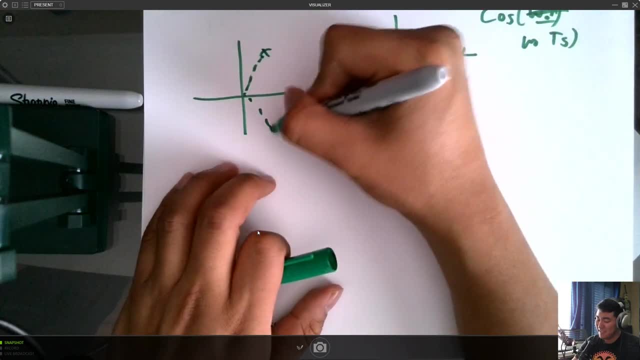 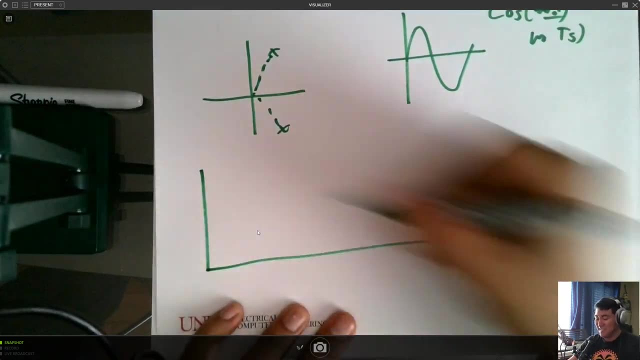 It's going to start resonating frequency, However complex conjugate. it's going to have to have some type of phase. But that's as much as I can show you. Actually, what I really wanted to show you was the Fourier transform. 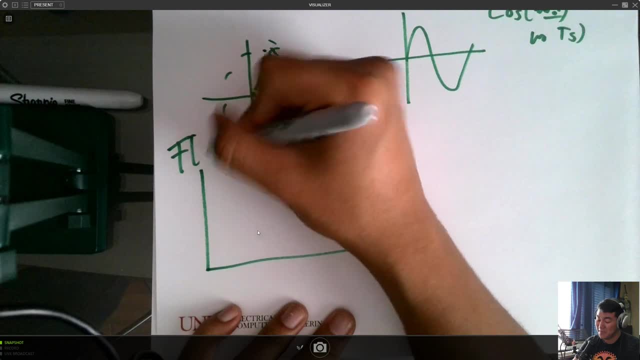 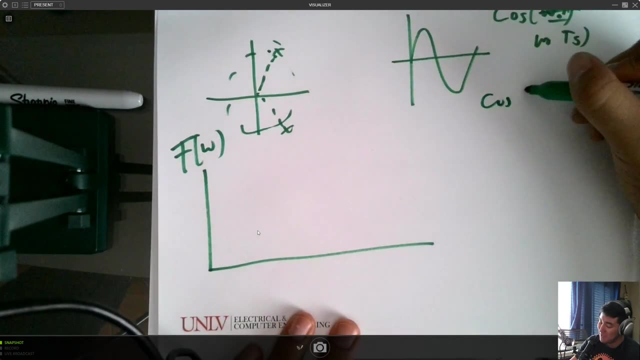 That's the whole point of what I wanted to get to you: The Fourier transform of your system. This is where all the crazy engineers go crazy. If you wanted to do cosine of omega, not T, OK, I'll call it actually two pi f t, because that's how I'm used. 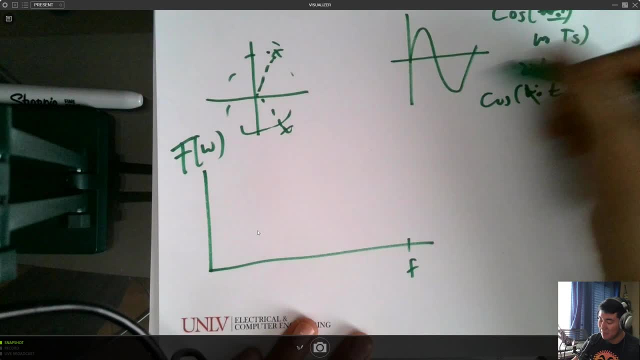 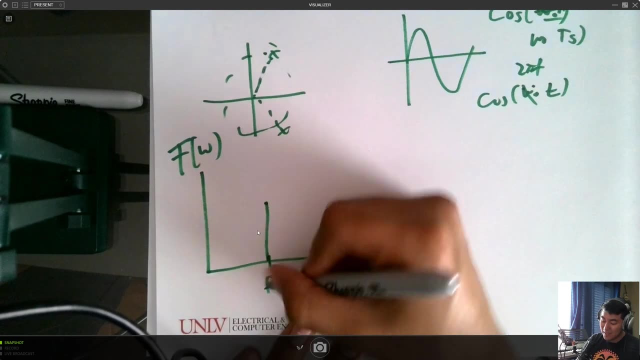 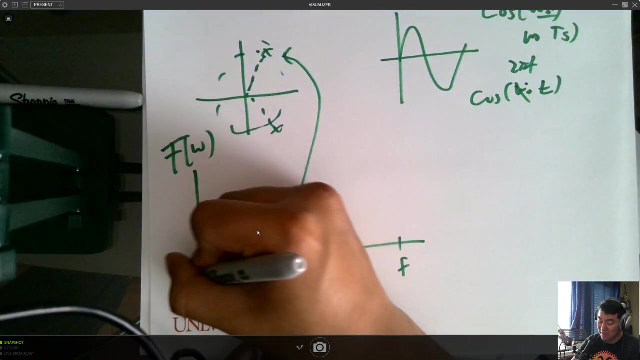 to. If you go on the frequency domain you can post this, as you know that a point right there. But if you were to put this f right here onto the Z, transform that right, there is there. If you were to draw the double spectrum, 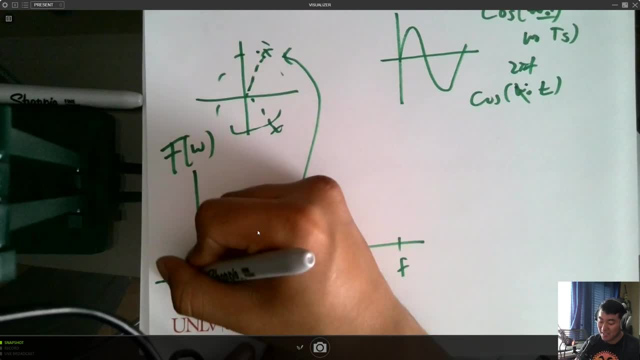 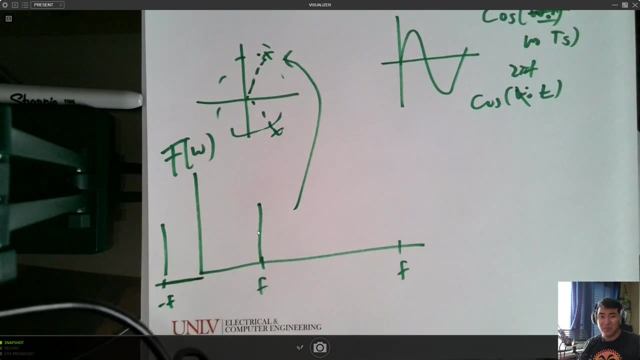 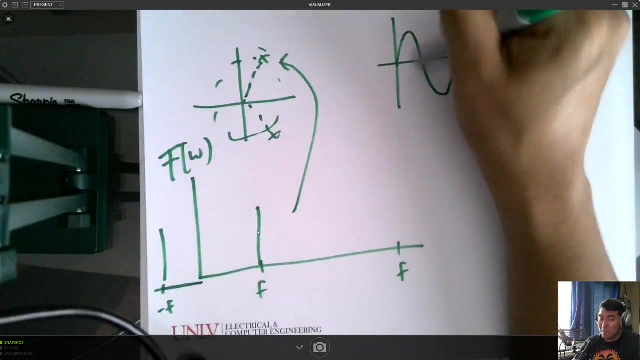 because the Fourier transform also has negative frequencies. you notice that you have a spot that comes right there. So this is the powerful thing I wanted to show you, And that's the Fourier transform And that's introduction To E361, where you're going to analyze, oh, systems signals like this: